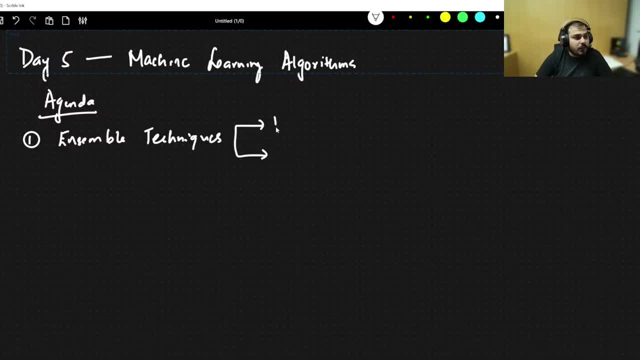 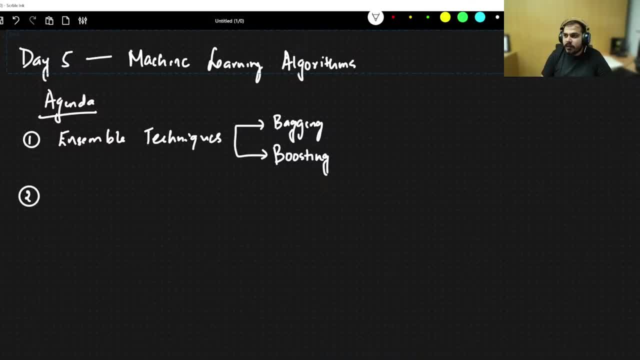 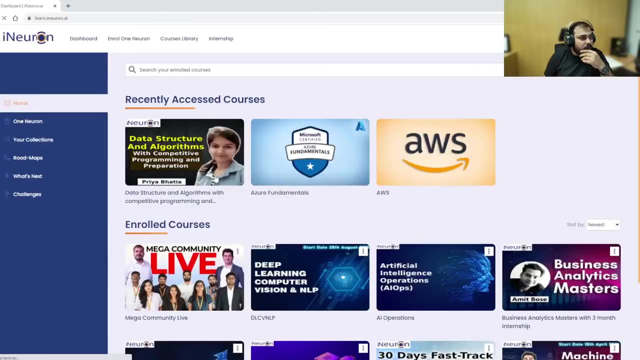 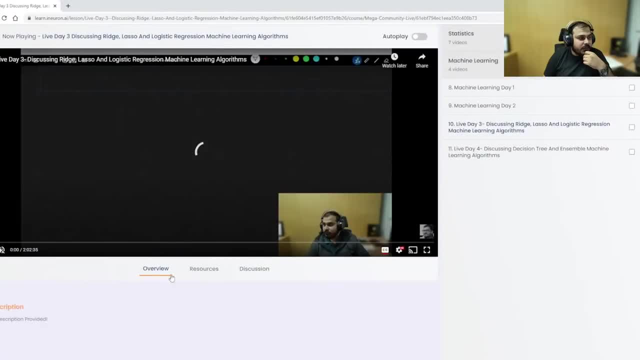 Everything is available. If you go to day three here, day four, all the discussion and everything is available here, Right, So just go and check it out. Everything will be available here. This is day five, right Day five. 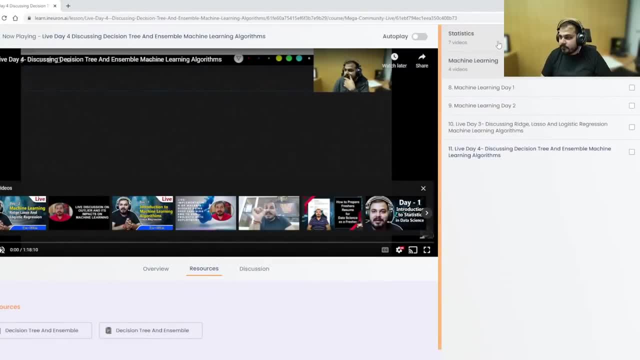 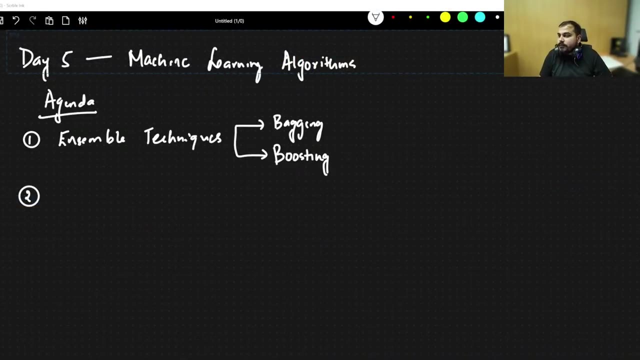 If you go and see in the resources again, everything is available Right. Okay, So the agenda of this session is ensemble techniques, bagging and boosting. then we are probably going to cover random forest and then probably we will try to cover adab boost and if I have more energy I will also try to cover xg boost. 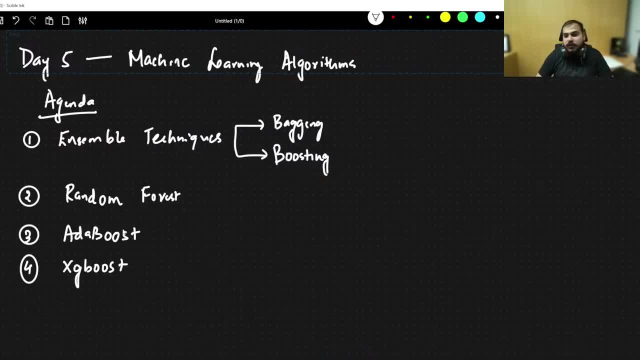 Okay. So all these algorithms, we'll discuss about it, Okay, And probably we will. We'll try to see what all things will be coming in today's session with respect to this, but I hope everybody is able to hear me now, Okay. 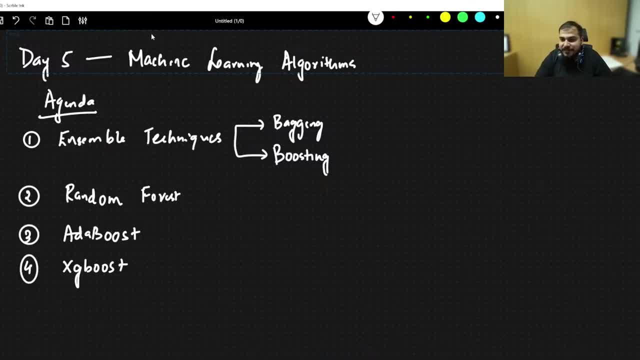 And, yes, hit the like button. I can see 300 people joining, but no likes. Why? Okay? So how was the previous session? I think it was quite amazing and you are able to learn properly. you are able to understand properly. 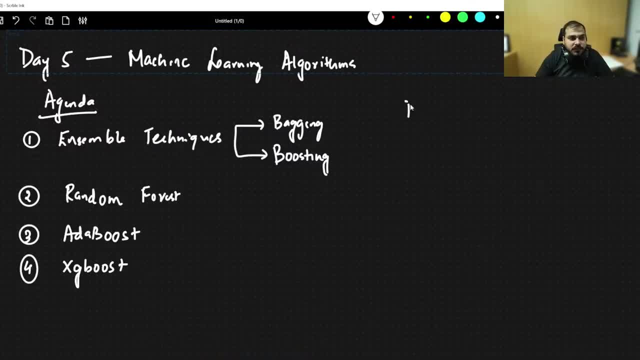 Yes, I may probably come up with Django also. So let's see, I will put up a vote next week and, yeah, we'll try to see what all things can be covered, like Django Flask. okay, specifically related to EDA deep learning. okay, so we will try to make this session. 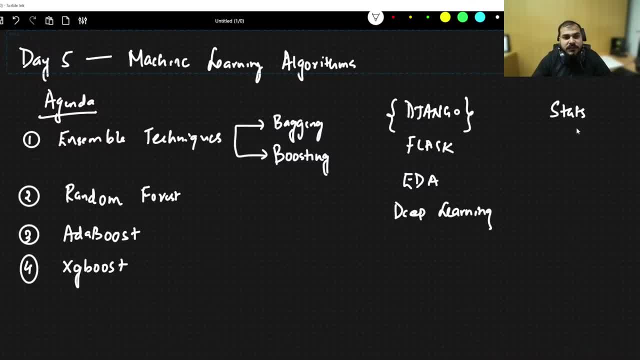 Right now, we have basically started stats and ML. probably in the future we may also have NLP, Okay, So all these things, but I'll take a break of around three to four days because I need to travel. Okay, And yes, that's it. 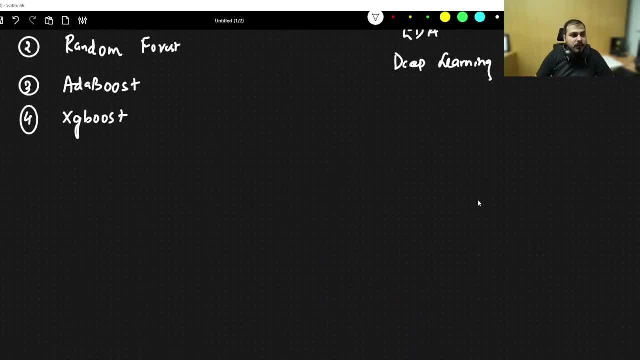 Just a quick announcement for everyone regarding One Neuron platform. Everybody, please listen to me on this platform, One Neuron platform. The platform has got matured. now We are having more than 100 plus courses and in a month we are trying to upload 20 courses. 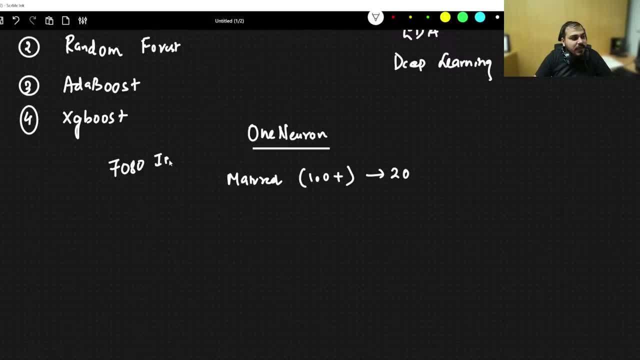 Right now the The price is 7080 INR for lifetime. okay, So this lifetime you will be able to see, you can also use 10% discount by writing Krish10 as coupon code. You can use Krish10, and probably from one month from now, mostly till March 31st. I guess this offer will be there only till March 31st. 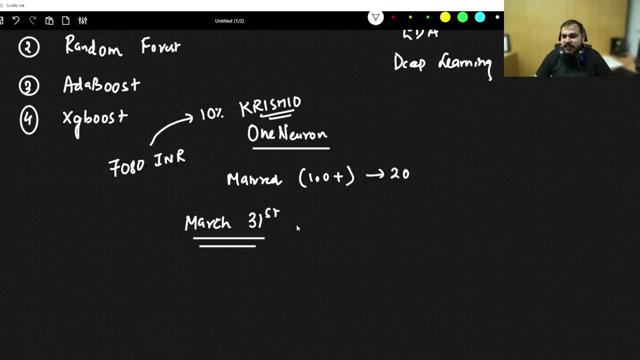 Okay, First till March 31st, probably in just some days. we are also coming up with live sessions, Live sessions inside One Neuron, Okay, So live session is also getting integrated, probably from Feb 2nd week or 3rd week. 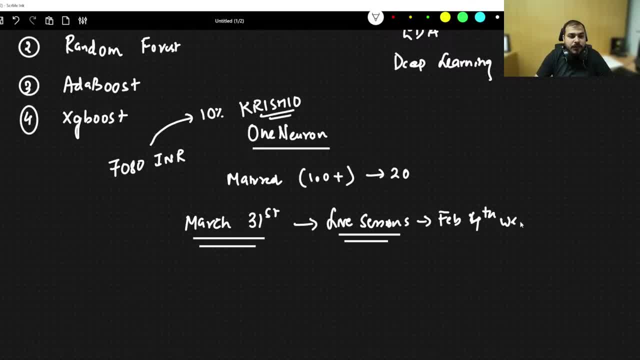 I think Feb 4th week. Okay, So after March 31st this price is going to become 20K INR based on subscription. basis Subscription basically means we are coming up with one-year, three-year, five-year plans. 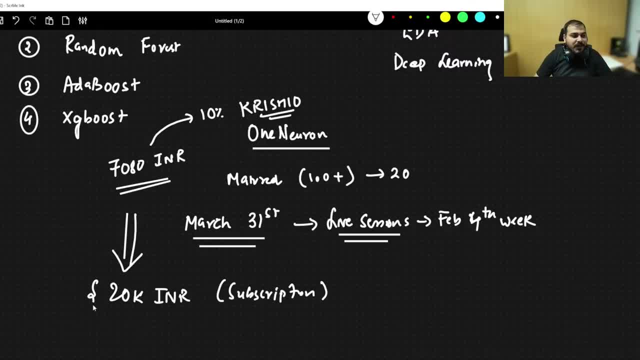 So utilize this opportunity, guys. Later on it will not be in my control to give you at this particular price, Because I am not the decision maker in One Neuron with respect to prices. So business decision. I have come up with this because at that point of time we will be having 200 plus courses without clearing session, live classes and all the things. 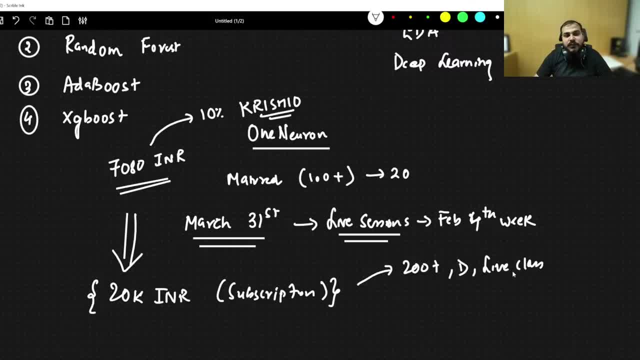 So it is a request: Please utilize this opportunity and take up One Neuron, Otherwise nothing is in my hand. Okay, And at that point of time, you don't scold me, Krish, You did this. You increased the price. 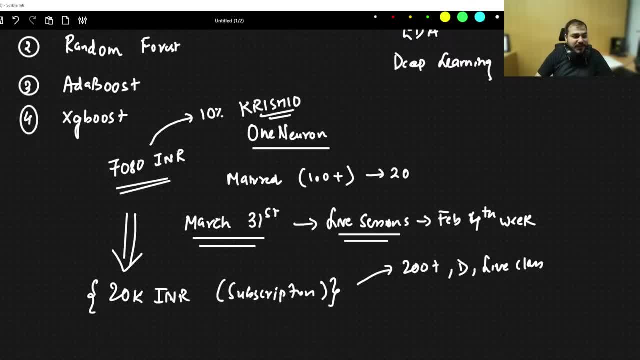 I did not do anything, Okay, So you will be able to see this: 20K INR. The price is going to become 20K INR. This has been decided by the investors, plus the business heads over here. Okay, And probably you will. 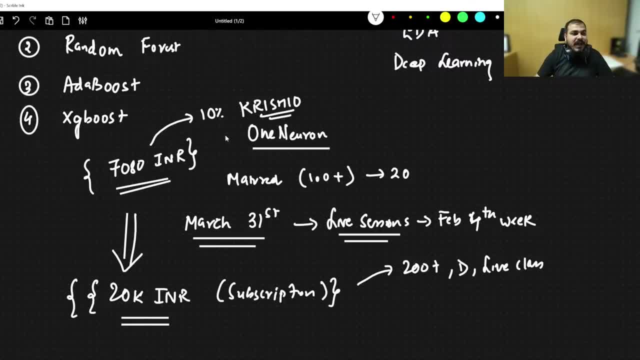 You will not be able to get it in 7080, and not specifically for lifetime. This will become one year, three year, five year subscription plan. So again, it's a request, Take it, Otherwise it's up to you. 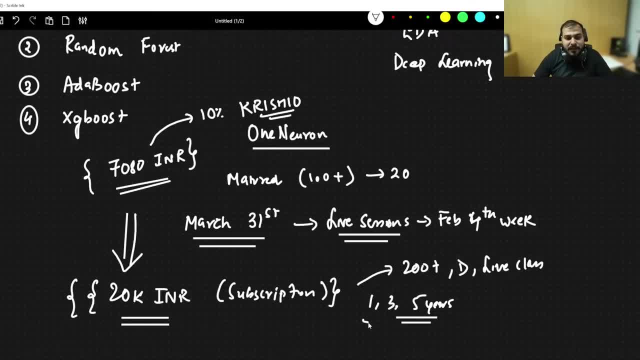 Okay, This 20K will be only for one year. three years, like one year plan will be 20K. three years- That will become a little bit more costly. and five year plan. We are just coming up with these three plans. 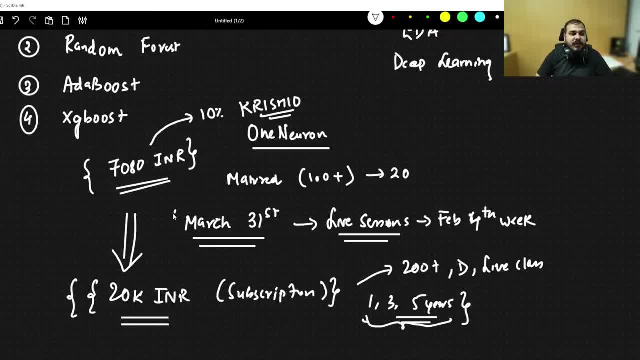 7080 right now is there For lifetime. mostly after March 31st we will not have that specific option because the platform will become completely matured. Okay, So it is up to you now. Go ahead, Take it. Don't scold me later on. 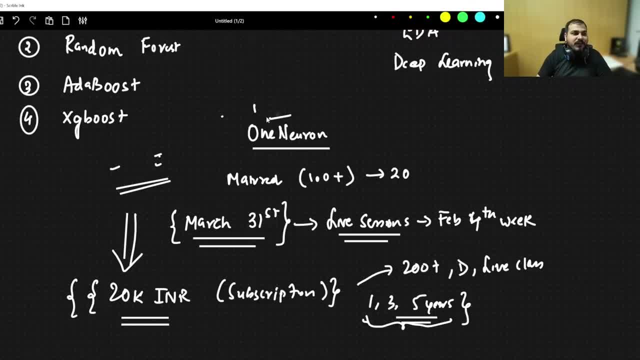 You cannot scold me because I tried to extend the offer till whatever thing was possible from me. Now it is up to you. Take ahead, Otherwise if later on if you want to go with high money, then not my choice. 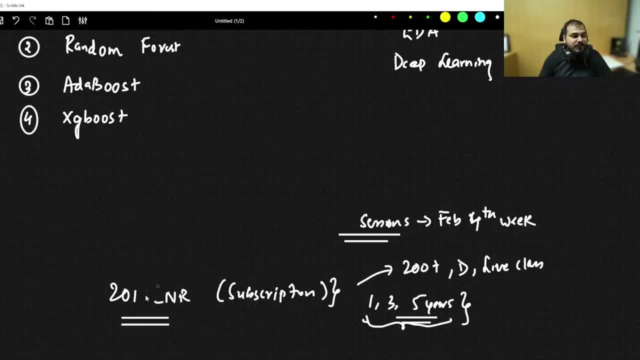 Okay. So for the people who have bought now, it's pretty much amazing. They are enjoying the lifetime thing They can give their kids and go, Because obviously you're not going to, you know, be in this earth for 100 years. 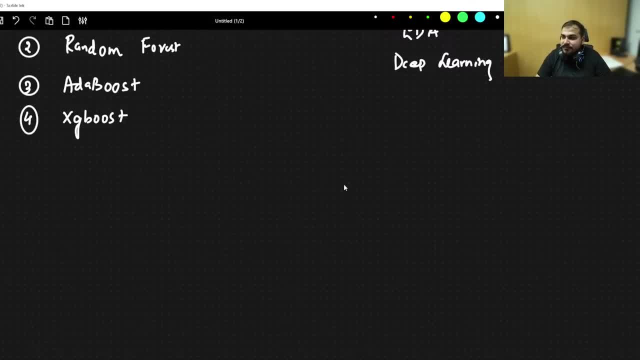 Okay, Okay. So let's go ahead and let's start the topics. These are the first topic that we are going to discuss. It's about ensemble techniques. Now, what exactly is ensemble techniques And we are going to discuss about it. 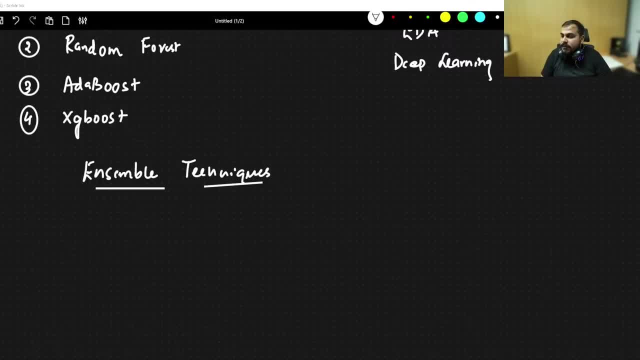 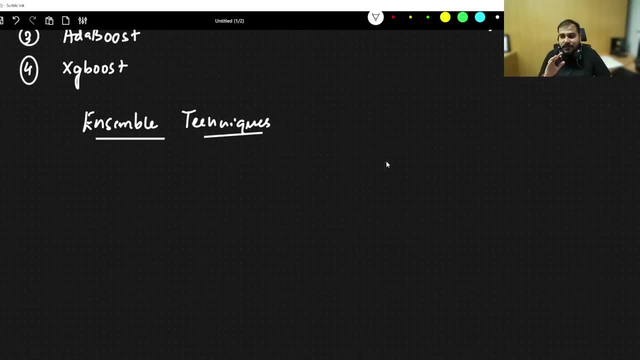 and take it, utilize this opportunity. you cannot tell me anything because i try to tell the, my entire team members to extend for some amount of time later on, because now we are having, we will probably be having 100 plus people in our company also, so we also have to look onto. 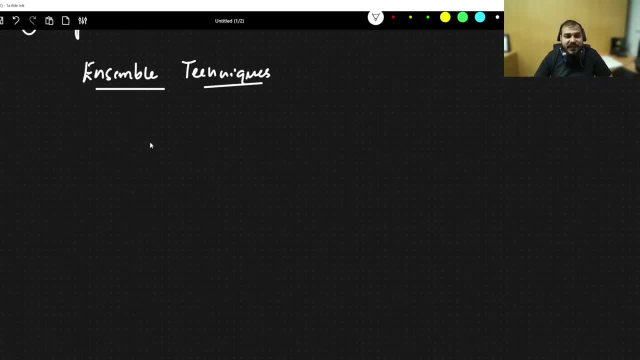 that so ensemble techniques. what exactly is ensemble techniques till now? so, guys, everybody ready, guys, you can find out all the information in the description regarding one neuron and all all the numbers also have given in the description. okay, so, uh, till now. uh, are we ready, guys should? 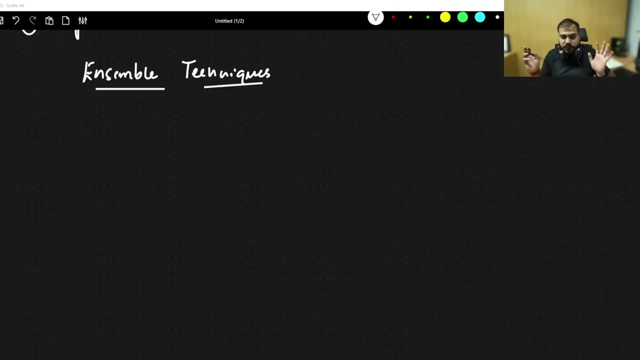 we go ahead. yes, big data spark: all the courses are available there. cloud is there, everything is there. okay, okay, guys. so shall we go ahead? shall we go ahead? everyone ready, ready, ready. yes, certification will also be given. in that already, certification is also given. i will just show you, if you want, okay, how the iron neuron. 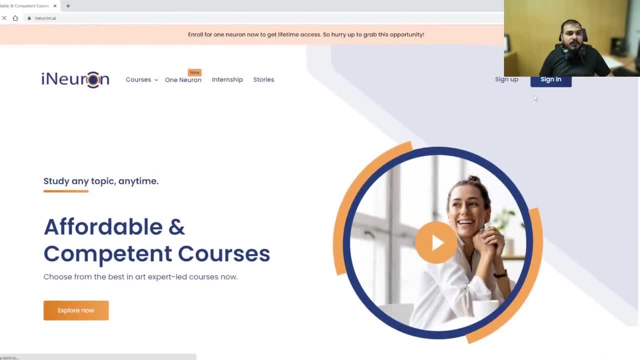 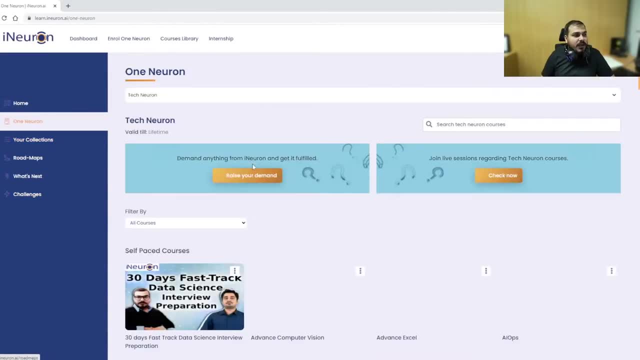 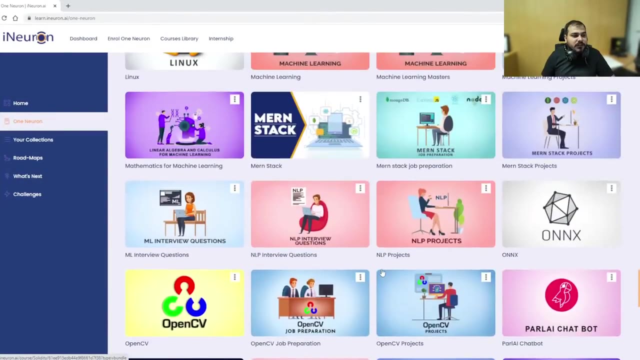 platform looks like now. now we are trying to add up a lot of options. so if you go and see over here, if you go in my courses, so this is how many options we have come up. one neuron- this is the one neuron platform. you can see all the courses here. we have included almost everything and still 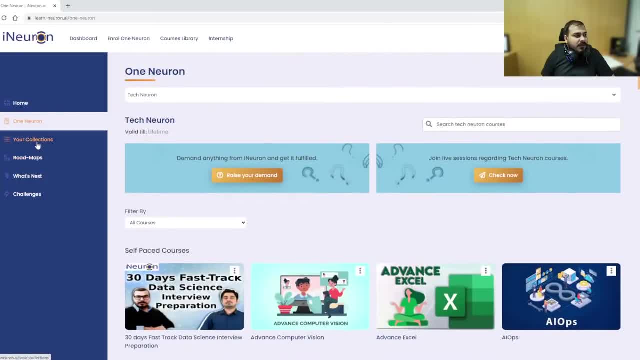 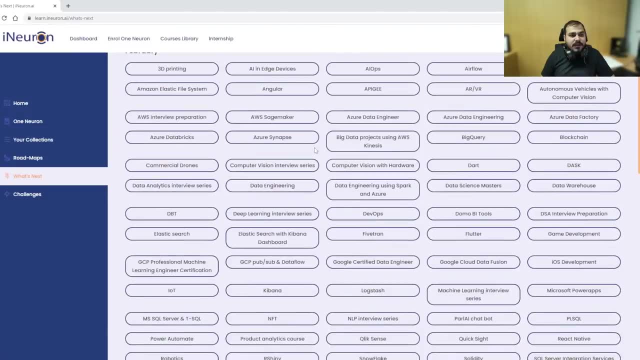 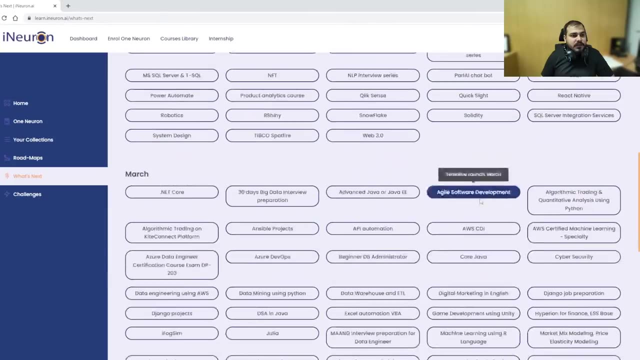 requests are actually going to come up and if you see we have also added options to you can see the what's next in the february month: this all courses are going to come in february. these all courses are going to come in march. this all courses are going to come. uh, modules, these all are going to 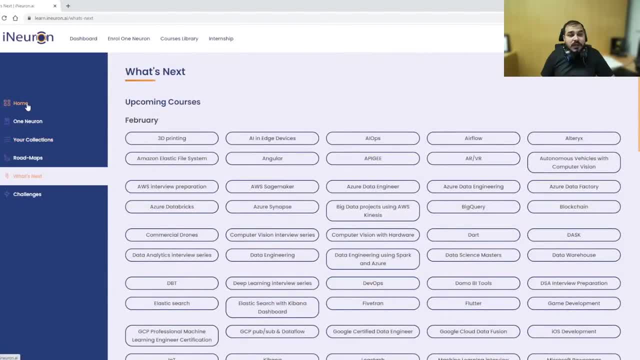 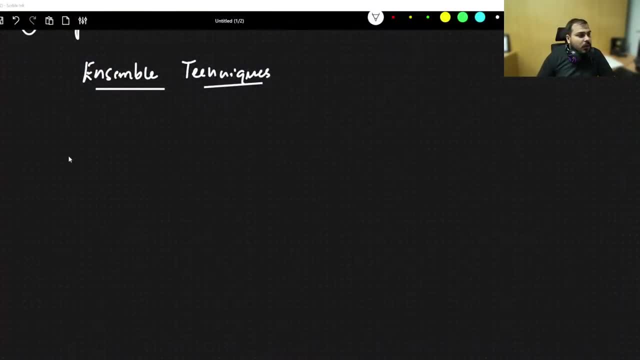 come. so everything is given over here, and we are also about to announce challenge for one neuron people. okay, so i will close it now. now let's go ahead with ensemble techniques. till now, we have solved two different kind of problem statement. one is classification and regression. okay, and 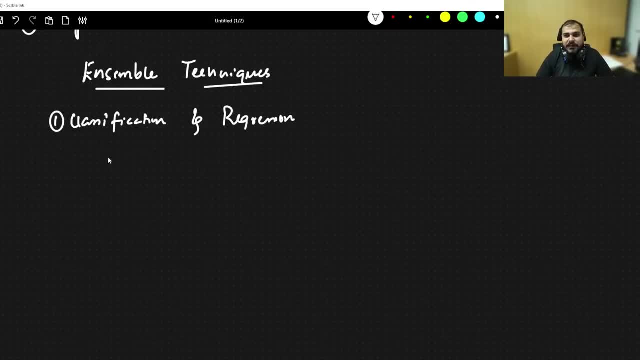 here. we have learned about different, different algorithms like linear regression, logistic regression. we have discussed about knn. we have discussed about yesterday what questions you have got, so i will get back to you guys in the middle and see you in the next video. okay, have a good. 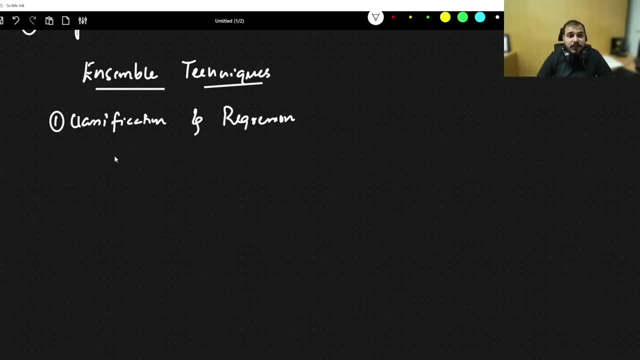 day. what did we discuss? our nape bias, different, different algorithms. we have already finished. okay, now, with respect to classification, regression problem. whatever algorithm we are discussing, there was only one algorithm at a time we were discussing, right, one algorithm at a time we are discussing and we are trying to either solve a classification or a regression problem. okay, till now we have. 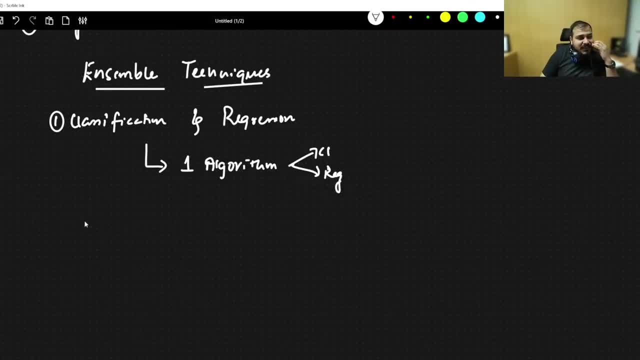 learned in this particular way. okay, now, the next thing is over here is that can we use multiple algorithms, multiple algorithms, multiple algorithms- to solve a problem? okay, multiple algorithms basically means can we? i'll just talk about it. okay, now in the if i ask this specific question. 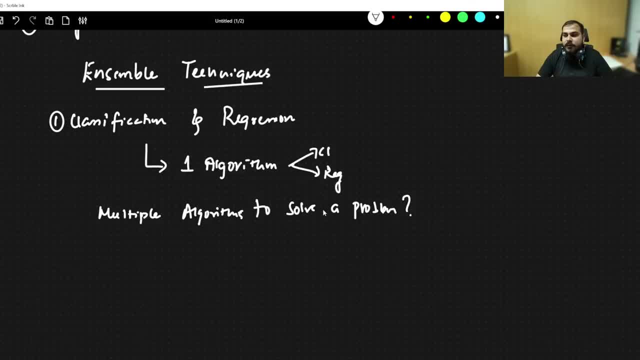 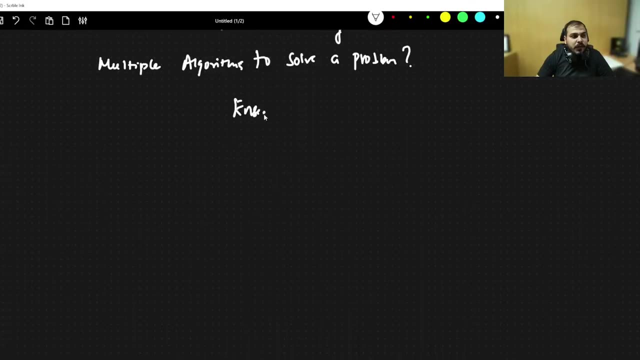 can we use multiple algorithms to solve a problem? okay, at that point of time i will definitely say, yes, we can, because we are going to use something called as ensemble techniques there. okay, now, what this ensemble techniques is. okay, so, ensemble techniques in ensemble techniques, we specifically use two different ways, two different ways. 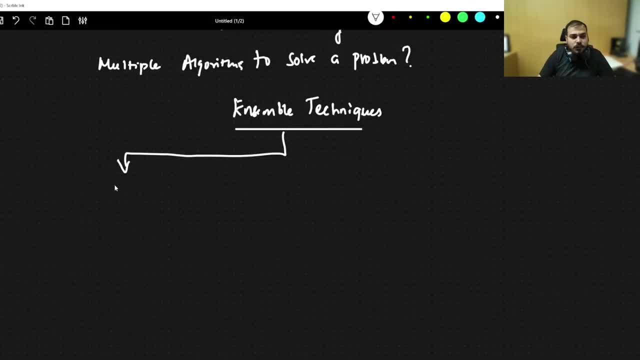 one is, one way is that we specifically use, and the other one- i'll just go to write it over here. so one that we basically use is something called as bagging technique, and the other one we specifically use is something called as boosting technique. okay, so, in bagging technique, in bagging technique, we what exactly we can do, and in boosting technique, 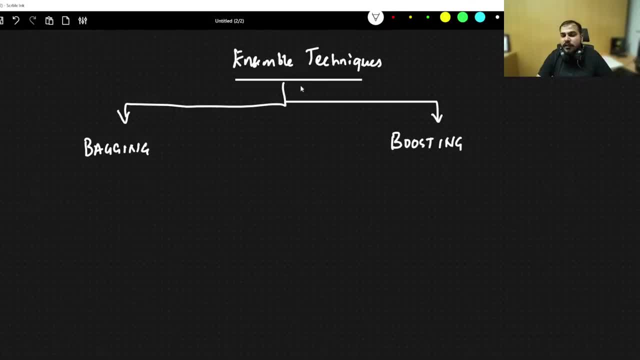 what we can actually do and how we are combining multiple models to solve a problem. okay, so let's first of all discuss about bagging now. how does bagging work? okay, how does bagging work? we'll try to discuss it over here. let's say that i have a specific data set. 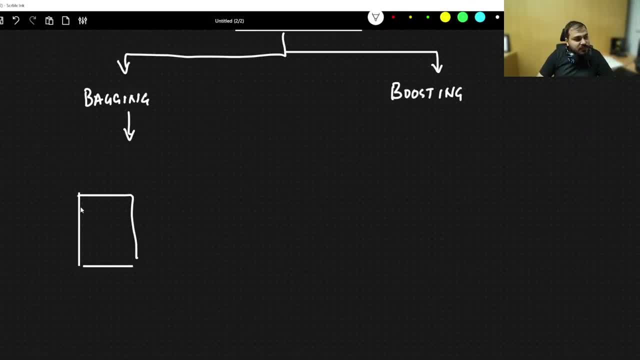 so this is my data set with: uh, with features, rows, columns, everything like this. i have this specific data set. okay, just imagine i have many, many features over here like this: f1, f2, f3, and probably i have my output. so this is my data set d. let's consider it okay now what we do in bagging. 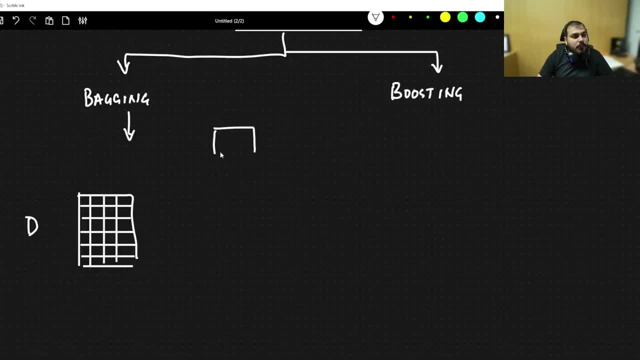 is that we create models, and this model can be anything. it can be logistic, it can be linear. for a classification problem. let's say that we create models and this model can be anything. it can be linear. for a classification problem. let's say that this is logistic model. so this is my model m1. 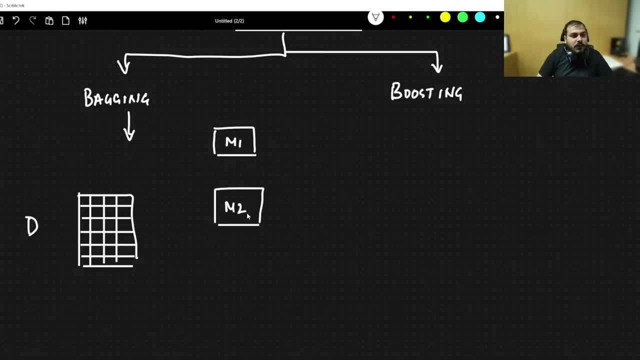 let's say, i have another model m2, then i may have another model m3. okay, i may have m4. tell me what all model we discussed with respect to classification till now with respect to classification- i'm just considering classification as an example what all model we discussed. let's say that this is: 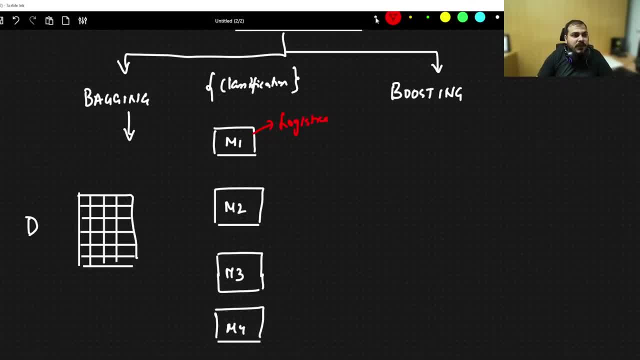 logistic, okay, and this is probably the other model which is like decision tree, okay, and then probably we use this model as uh knn classification, okay, and this model can again be decision tree, it's fine, let's use another decision tree, okay. so now here you can see that we have used so many models. okay, so many models are there. 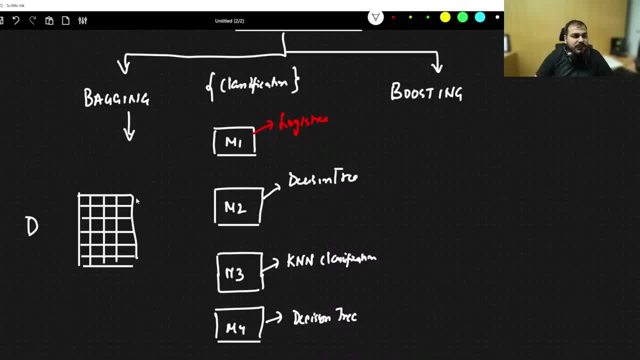 now, with respect to this particular model, what i will do is that the first step that i will do from this particular data set, i will just take up some rows and i will just take up some rows and i will. so i'll basically do row sampling and i'll take a row sampling of d dash. d dash basically means 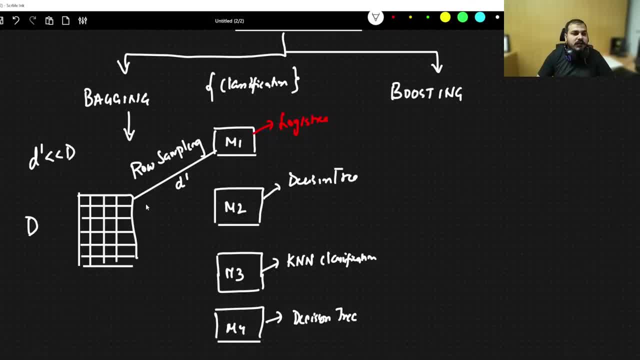 this d dash is always less than d. some of the rows i'll push it to m1, okay, okay, i can also use name bias, fine, okay. so what i'll do is that some of the rows i'll push it to model one. this model one will be training. okay, let's say that for out of this ten thousand record thousand rows, i'm 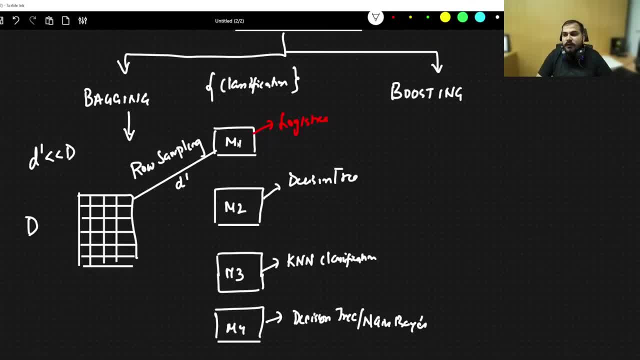 actually doing a row sampling of d dash. so i'll take a row sampling of d dash and i'll take a row sampling of thousand rows and giving it to m1 to train it. then what i'm actually going to do over here, i'm basically going to give this specific model m2 and again i'm going to do row, row. 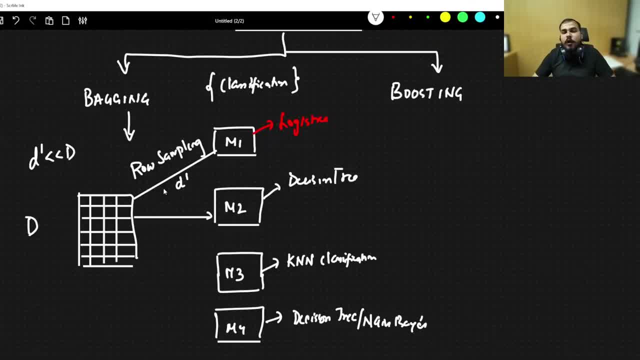 sampling and i'm again going to sample some of the rows and give it to model two. and again, remember some of the rows may get repeated: from this d dash to next d double dash. okay, similarly, i will do row sampling and give it to this, and again i may have d triple dash and d four dash, so different. 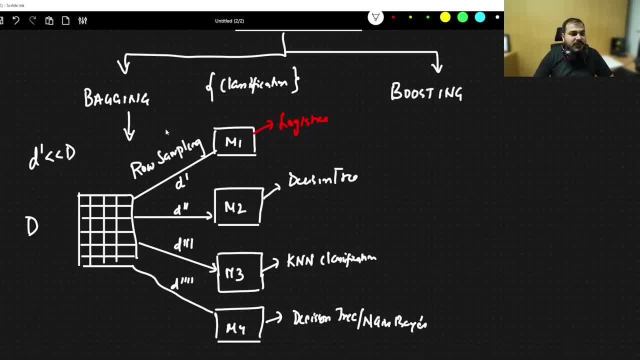 different, different rows, data points. when i say row sampling, basically i'm talking about data points, different, different data points. i will give it to separate, separate model and this model will specifically train. when i say d dash, that basically means: uh, suppose i say 10 000 are my. 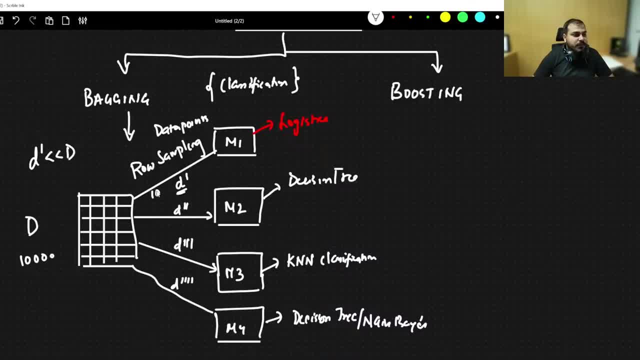 total number of data points. when i say d dash, this d dash may be thousand points, then d double dash may be another thousand points and some of the rows may get repeated over here. d triple dash- here also i can basically use. so here specifically, row sampling will be used. okay, i'll talk about. 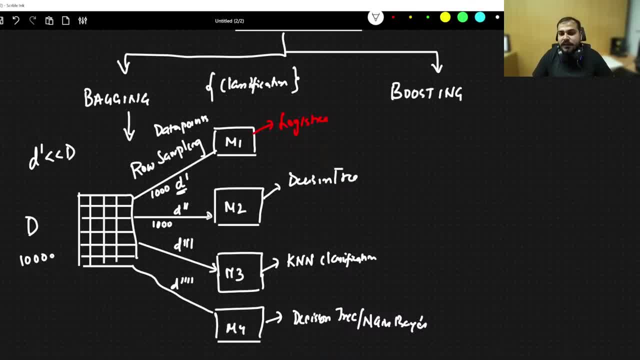 column sampling, also santosh column sampling will specifically happen in random forest, which i'm going to discuss about it now when i have this many specific stuff. each and every model will be trained with different kind of data. now how the inferencing will happen for the test data. 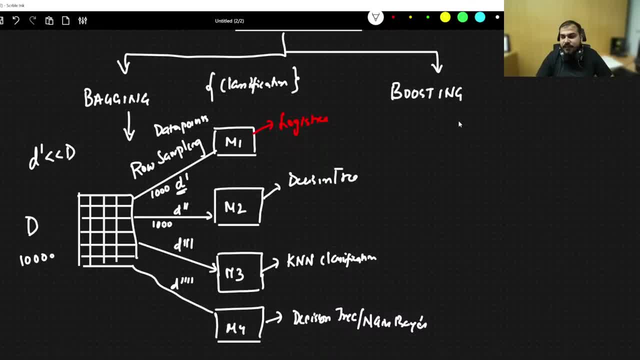 okay, how the inferencing will happen with test data. okay, so first thing. first let's say that i'm going to get a new test data over here now. new test data will be passed to m1- okay, will be passed to m1 and this m1, suppose it gives. 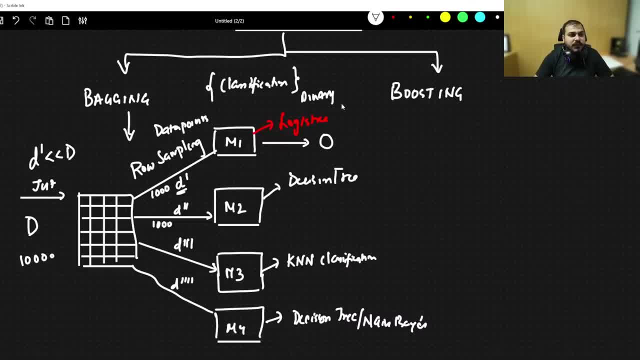 0 as my output. suppose let's say that i'm doing a binary classification. okay, it gives a 0 as an output. so this is my output of 0.. next, m2, for the new test data, gives 1, m3 gives 1 and m4 also gives. 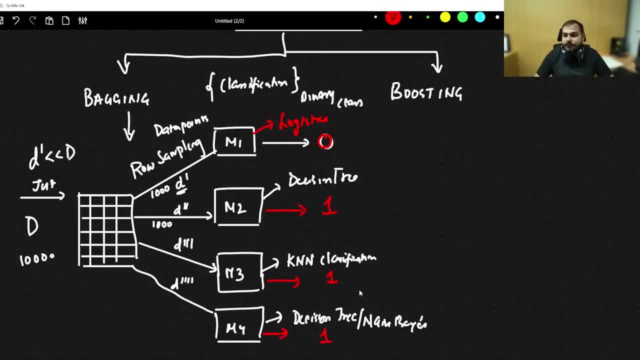 1 as the output now in this particular case. in this particular case, what will happen now? you can see over here, it's simple- what. what do you think the output may be in this particular case now? m1 has predicted for this particular test data as 0. the model m2 has predicted 1. 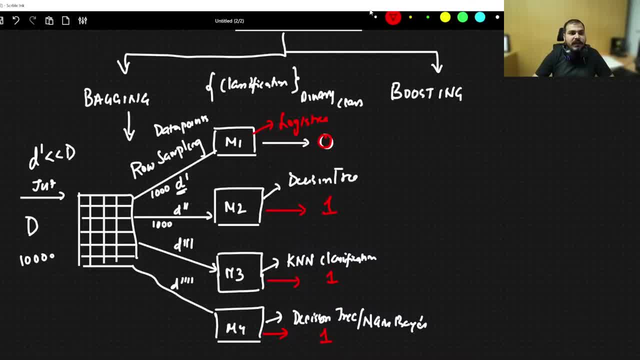 m3 has predicted 1 and m4 has predicted 1.. so, finally, all these outputs are going to get aggregated, are going to get aggregated, and a simple thing that gets applied is majority voting. okay, majority voting. so please tell me what will be the output with respect to this? the output will obviously be. 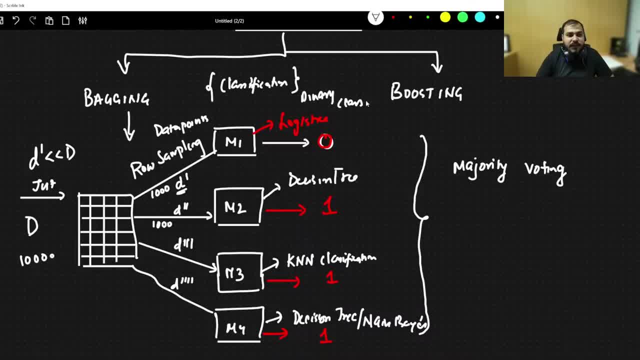 one because the majority voting that you can see three people are basically saying it as one, so my output over here will be one. okay, will be one. so this is the concept of bagging. okay, this is the concept of bagging, wherein you are providing different, different rows with probably all the 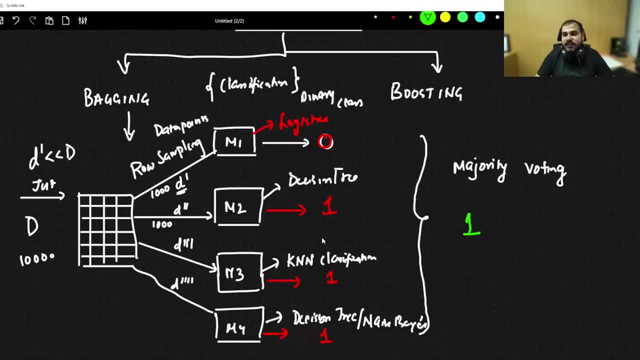 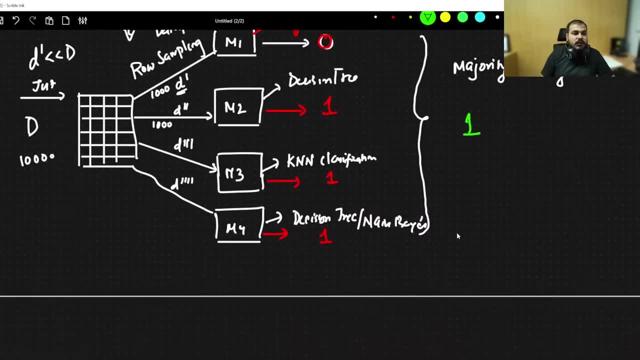 features, in this case, and giving it to different, different model again, which is a classification model. then, finally, you are combining them based on majority voting and you are getting the answer as one. okay, so this step is called as bootstrap aggregator. bootstrap aggregator: that basically means you are aggregating. 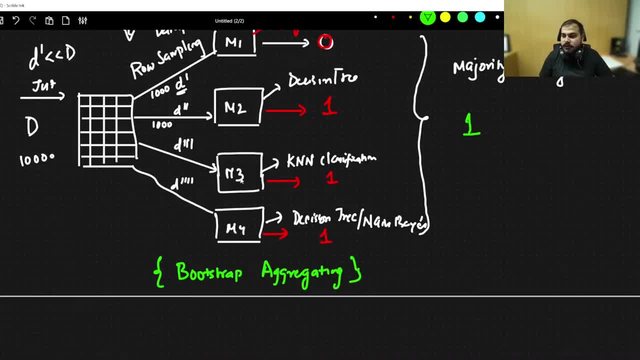 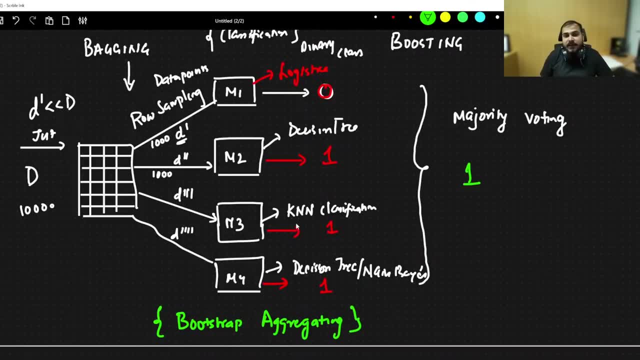 all the output that it is basically coming from. all the specific models. okay, all the specific models. now many people will say, krish, what about time? time guys like this kind of situation. you know we will be having more than 100 to 200 models, so it is very, very difficult that it will be a tie okay. 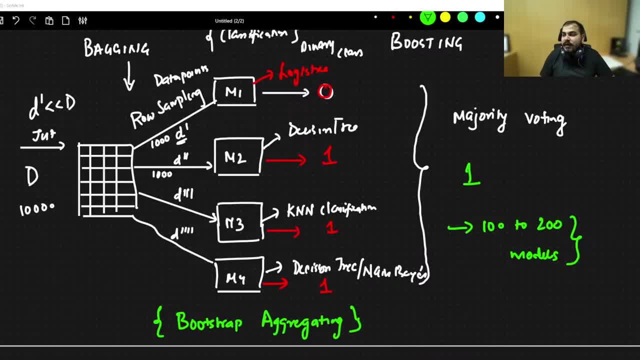 okay, who are repeating questions? they will be put up in time, okay. so what if you are saying that if the 50 of model says yes, fifty percent of models says no, always understand, guys, we will be having more than 100 to 200 plus models. okay, so in this particular 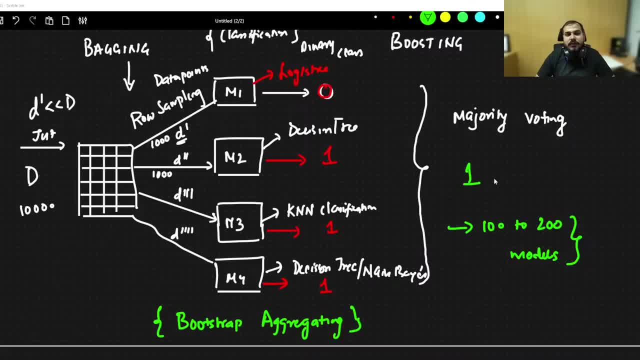 case, there will be high probability that always there will be a majority voting available. okay, it will always not be in that specific scenario, okay? so this was the concept about bagging. now some people will be saying that, krish, why are you using different, different models? guys, i'm not. 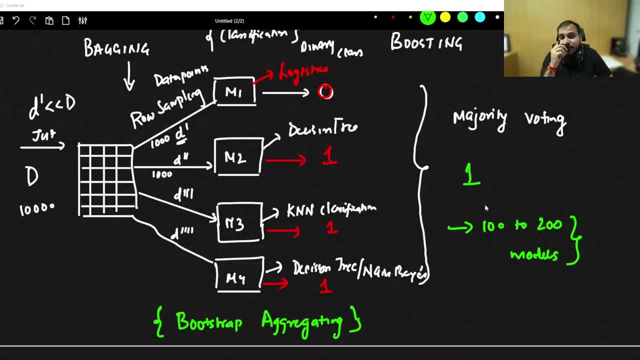 discussing about random forest over here. random forest uses only one type of model, that is, decision tree. but if we think as an concept of bagging, you can have different, different models over here and you can basically combine them okay. so this is a technique of ensemble techniques. 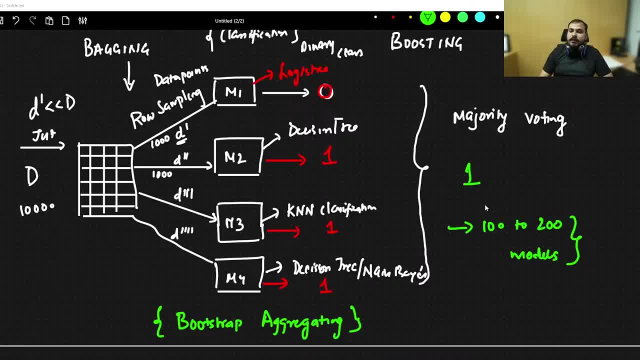 and this is basically called as bagging. okay, no, diksha, we don't use one algorithm, we can use multiple different algorithms in bagging. okay, when we say custom ensemble techniques, we can use definitely different different models. now, i hope everybody is you able to understand this? 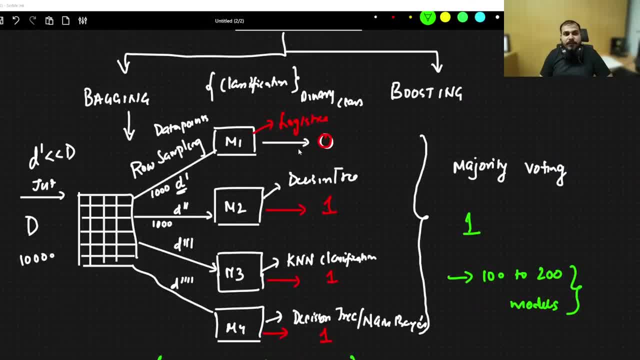 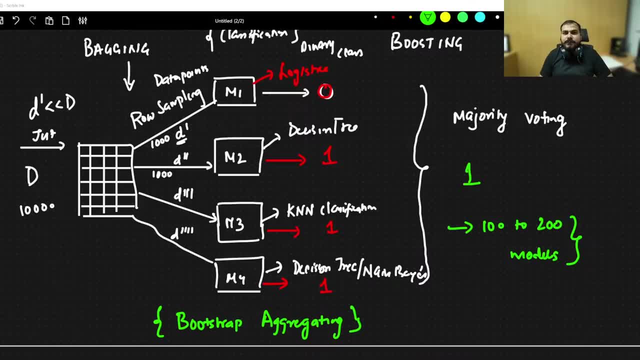 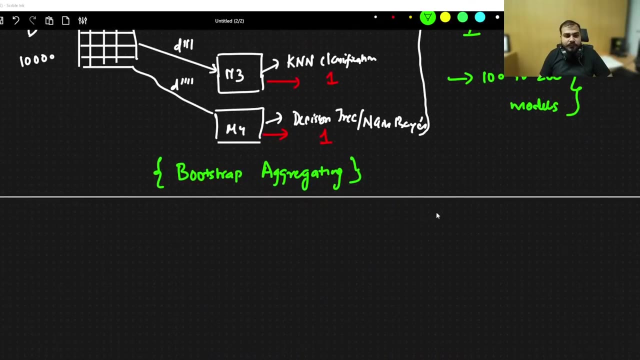 i hope everybody is able to understand. can i get a quick yes along with likes? likes are very less. why today? okay, go ahead, tell me. i hope everybody is able to understand it right. i hope everybody is able to understand it right. okay, perfect, so let me go ahead with the next one. 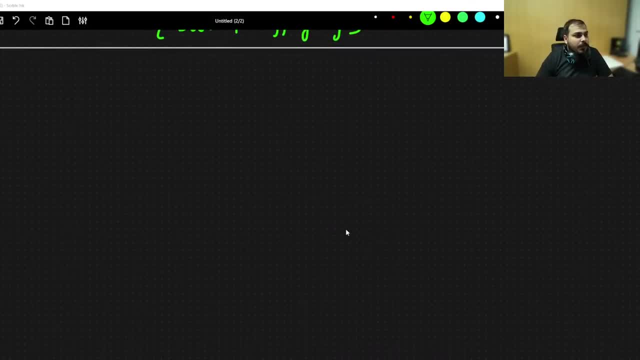 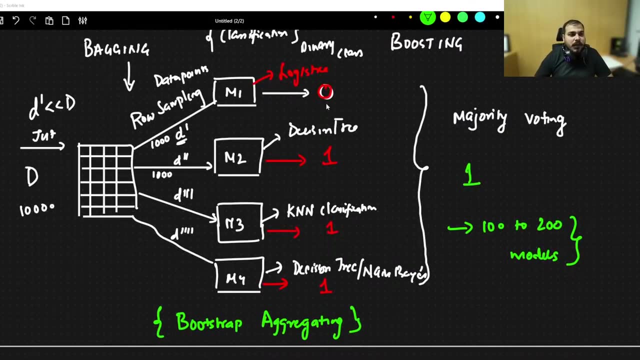 okay, okay now tell me one point i missed out. fine, this is with respect to the classification problem, with respect to the regression problem. what will happen with respect to the regression problem? what will happen over here? what will be my output in this particular scenario, in the case of a regression problem? in case of a regression problem, let's say that i got here 120. 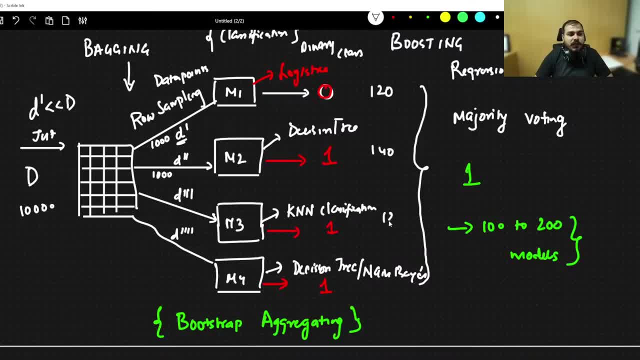 here 140, here 122, here 140- herealarment method. so, basically, what is going to happen now? you have some clean calls: here 120, here 140, here 102, here 130. how many different orders you have, Wonderful, okay. so that's the communication part. i'm going to highlight just one. fine, in one moment. okay, let's. 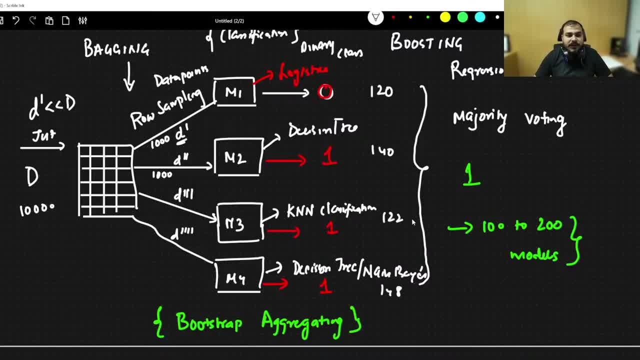 148 as an output. so in regression, what will happen is that the entire mean will be taken. mean will be taken, the output mean will be basically taken and that will be your output of the model. okay, average or mean, very simple, right, okay. so average or mean will be. 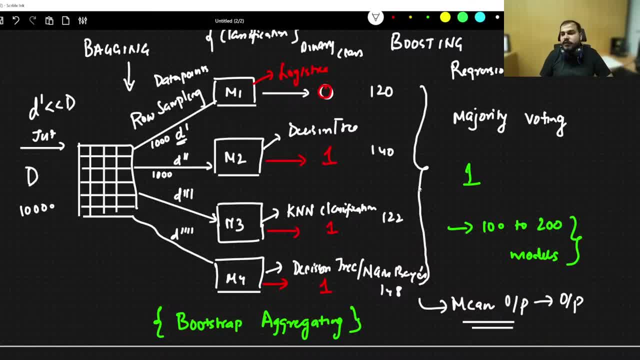 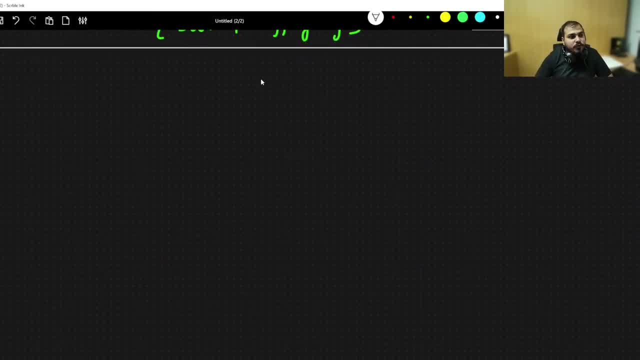 basically taken up and here, based on the average, you will be able to solve the regression problem. okay, great, now let's go ahead and try to understand, with respect to bagging and boosting, how many different types of algorithm are there. but before that, i need to make you understand what. 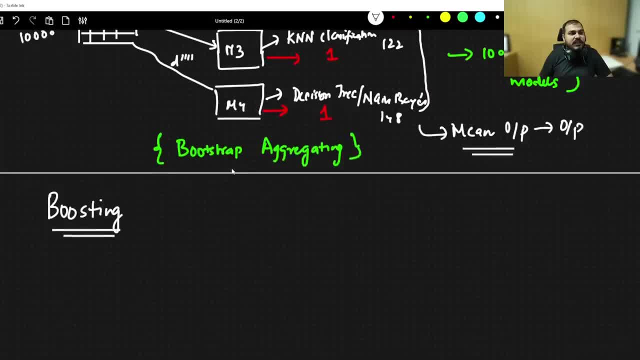 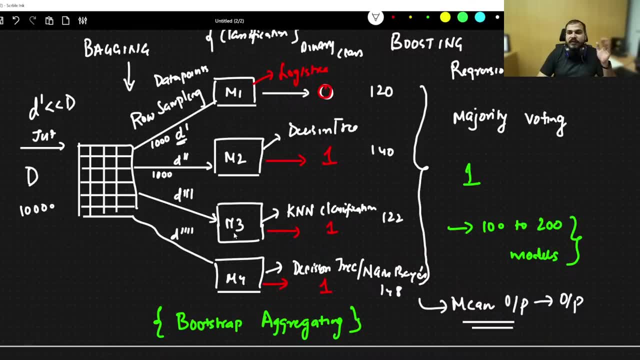 exactly is boosting? now, here in bagging, you have seen that you have parallel models, right, one one, one independent. you have parallel models. you are giving some row samples in different, different models and basically you are able to find out the output. okay, now in case of boosting. 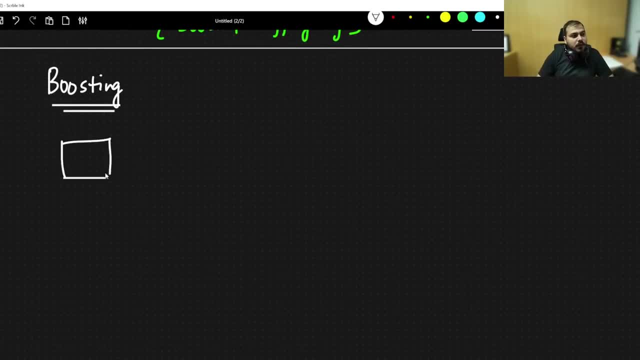 boosting is a sequential, combinational combination of models like this. you have lot of sequential models like this and one after the model, like: first i'll give my training data to this particular model, then it will go to this data, then this model, then this model. so this will be my m1, m2, m3, m4 and finally i will be getting my 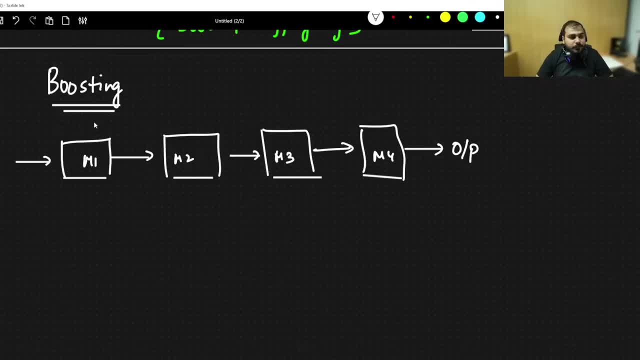 output. so here you can basically say that boosting is all about, and this m1, m2, mt, we basically mention it as weak learners. you so this will be weak learn, a weak learner, weak learner, weak learner. and finally, when we go to here in, it will, if i combine all these, weekin others. 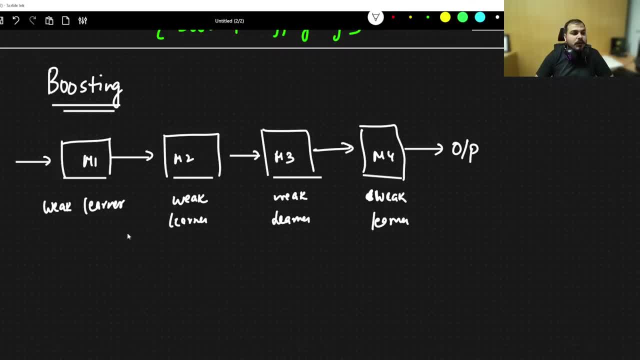 we plan a. we plan ok. once. combine all this week: learn a, it becomes a, becomes a, it becomes a strong. a lot of g. finally, if i try to camp and this, this will be basically become a strong learner. okay, so here you have all the models sequentially, one after the. 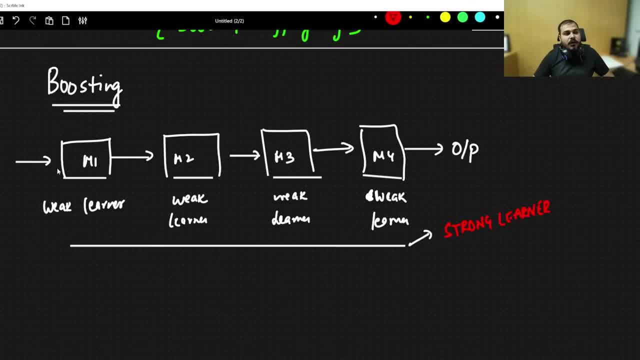 other, and then you will probably try to provide your input from one model to the next model, to the next model, and these all models will be a very simpler, weak learner model which will not be able to predict properly. but when you combine all this particular models together sequentially, 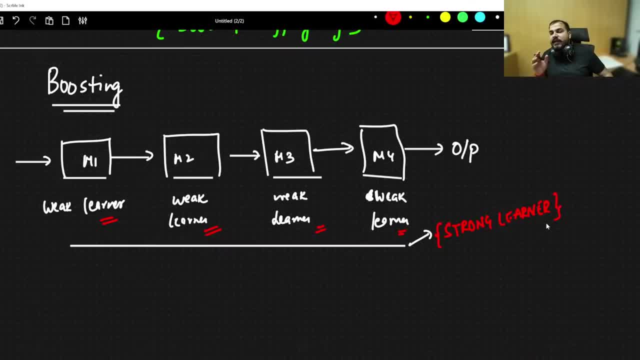 it becomes a strong learner. how this specifically works. i'll take an example of ada, boost, xg boost. i will show you that. okay. weak learner basically means the prediction is very bad- okay, for those models. but as you go sequentially, you combine them, they become a strong learner, okay. one example: i 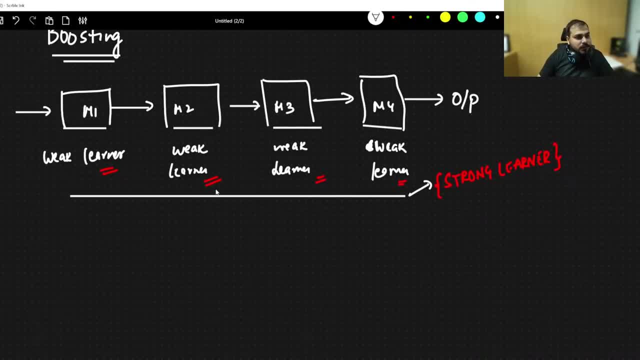 want to give you. let's say that. let's say that you are a data scientist, right? let's say that this model one may be a teacher with respect to physics. okay, then this model two may be a teacher with respect to physics. okay, then this model two may be a teacher with respect to physics. 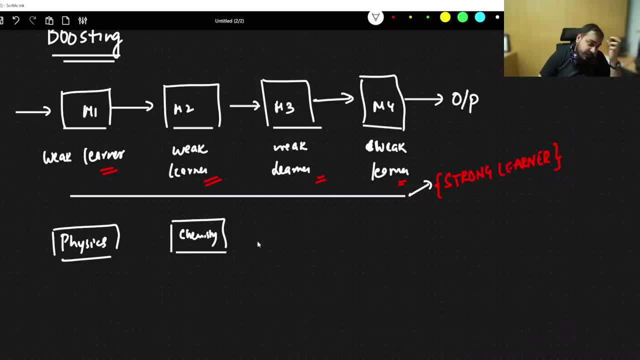 with respect to chemistry. okay, let's say, model three is basically a teacher of maths and model four is a teacher of geography. okay, now suppose, if you are trying to solve one problem, obviously, if the physics teacher is not able to solve that particular problem, then probably chemistry can help or maths can help, or. 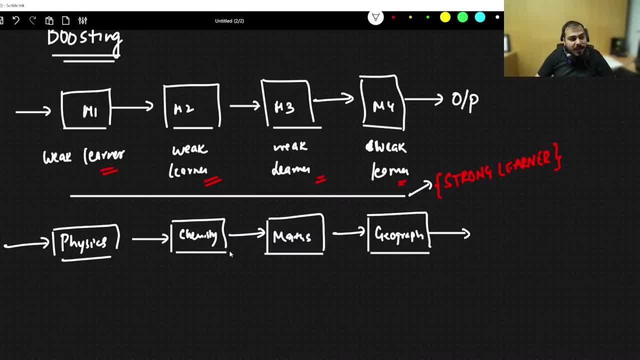 geography can help or someone can help. so when we combine this many expertise together, they will be able to give you the output in an efficient way. okay, so i hope everybody is able to understand sumit- i'll talk about it where- whether all the features are basically passed to all the models. 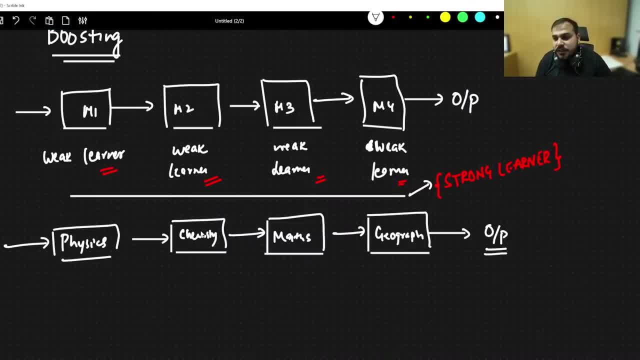 or not. i'll just talk about it. just give me some time, okay, but i just want to give you an idea about, in short, if someone asks you in an interview what exactly is boosting, okay, boosting is, you can just say that it is a sequential set of all the models combined together and these all models that are 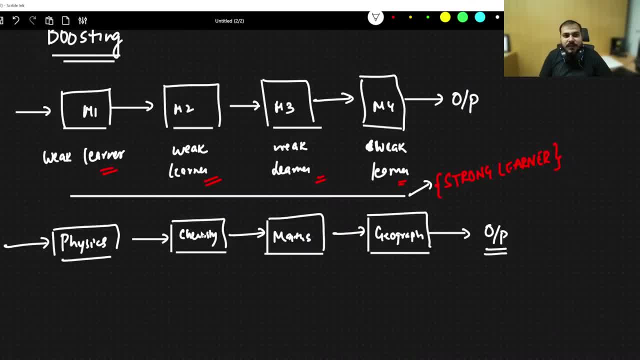 initialized are usually weak learners and when they are combined together, they become a strong learner and, based on this strong learner, they give them amazing output. and right now, if i say in most of the kaggle competition, they use different types of boosting or bagging techniques. okay, 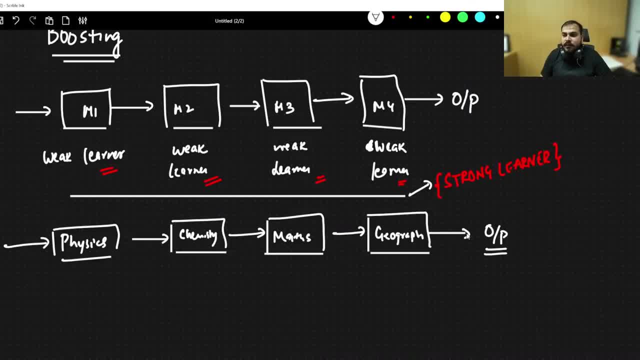 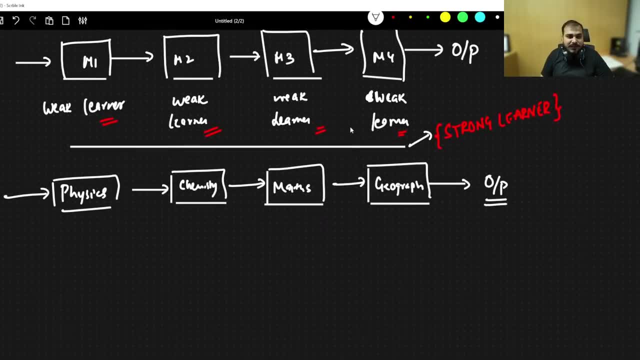 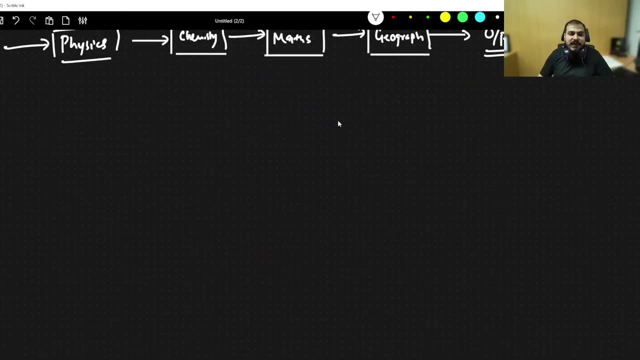 so i hope everybody is able to understand till here. okay, and i will show you with all these examples. so combine: okay, don't worry, i will show you. i'll show you an example. okay, don't worry, people, don't worry, i will show you by solving some examples. i will when i'm discussing about 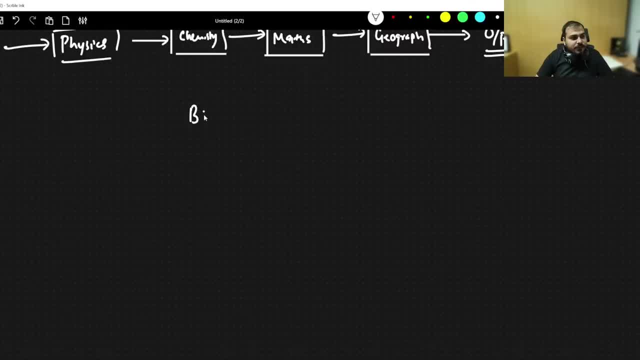 random forest and all. so you'll understand. so we have basically, as i said, bagging and boosting. in bagging, what kind of algorithm we specifically use? we use something called as random forest classifier and the second model that we specifically use is something called as random forest regressor. 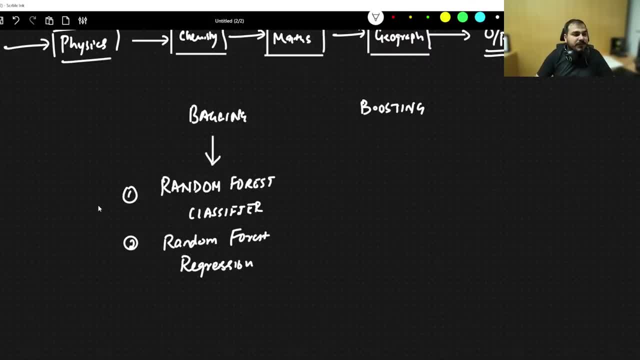 so we specifically use these two kind of models which i'm actually going to discuss right now. after this, and then in boosting, we basically use techniques like ada boost, gradient boost. number three is extreme boosting, and the second model that we specifically use is random forest extreme gradient boost, which we also say it as xg boost- extreme gradient boost. so all these things. 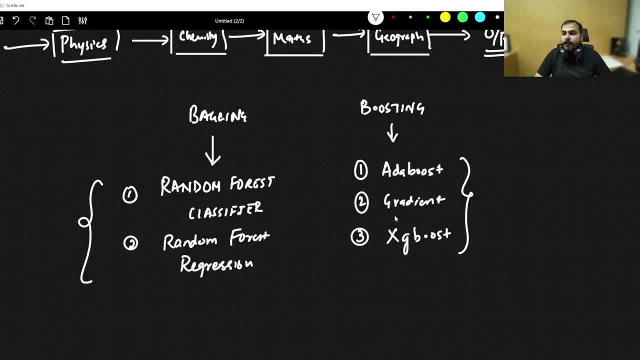 we will try to cover, let's say, whether we will be able to complete it today or not. but let's say i'll try my level best, whatever is trying to get completed, because again i have to go slow. i don't know how many people are learning for the first time and all and how they will be following. so 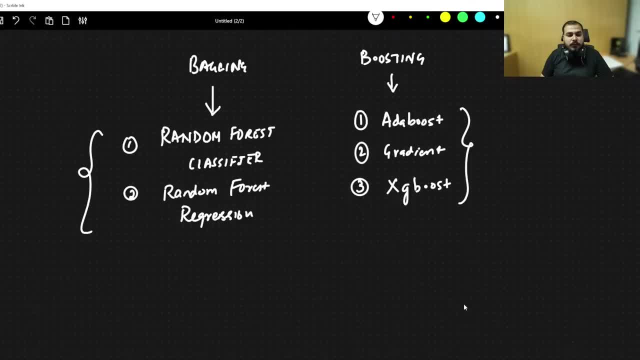 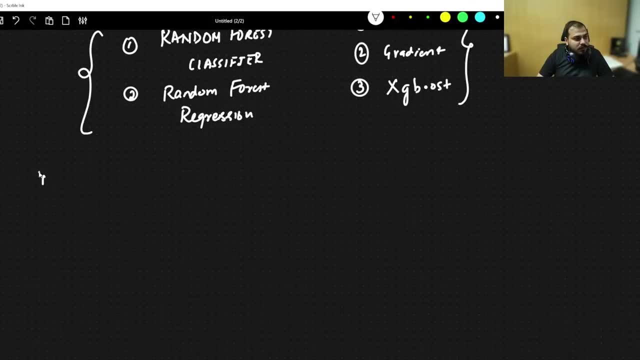 based on that, i will try to teach it little bit, slow. whatever things gets completed today, it's fine. otherwise, tomorrow the rest of the day will be the same. so i will try to teach it a little bit and the remaining part will get completed. so let's go ahead and let's discuss about the first. 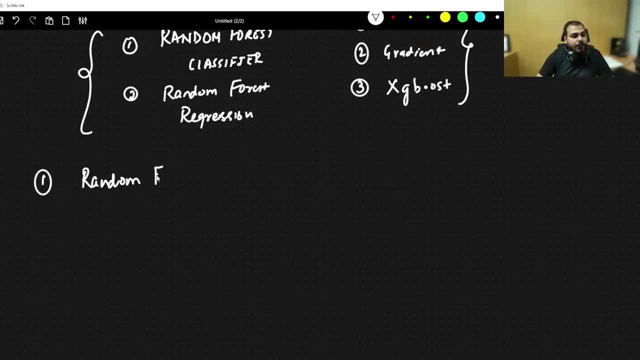 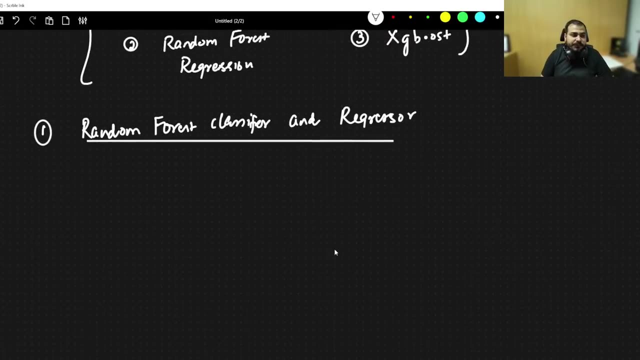 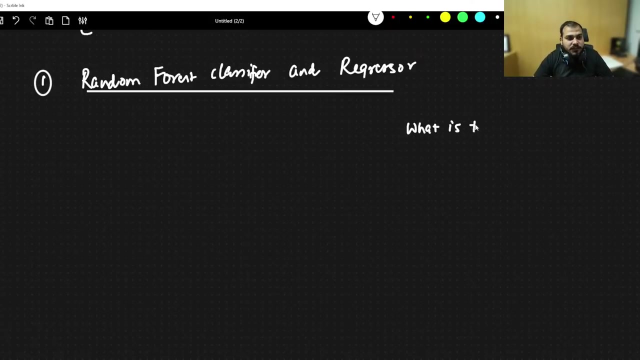 algorithm which is called as a random forest, random forest classifier and regressor. okay, now, first thing. first let's understand some things from the yesterday's class, i hope. what is the main problem with respect to decision tree? what is the main problem of decision tree? let's say, i have this particular question for you. i hope everybody remembers decision tree. 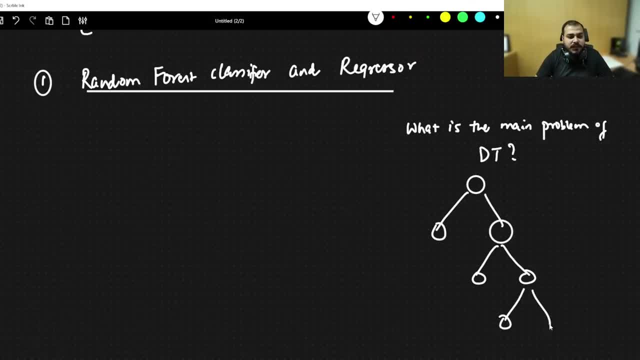 from yesterday's session. whenever we create a decision tree without any hyper parameter, does it not lead to overfitting? does it not lead to overfitting? tell me, yes, okay. does it not lead to overfitting? whenever you probably have a decision tree right, it leads to something like overfitting. why overfitting? because it completely 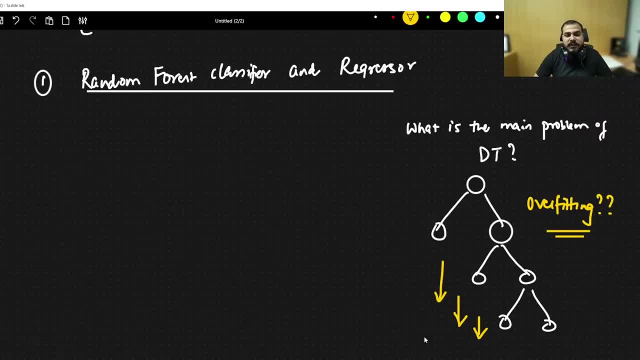 splits all the feature till its complete depth. okay now, during this scenario, overfitting basically means what we discussed, right. overfitting basically means: for training data, the accuracy is high. for test data, the accuracy is low. okay, so training data when the accuracy is high, i may. 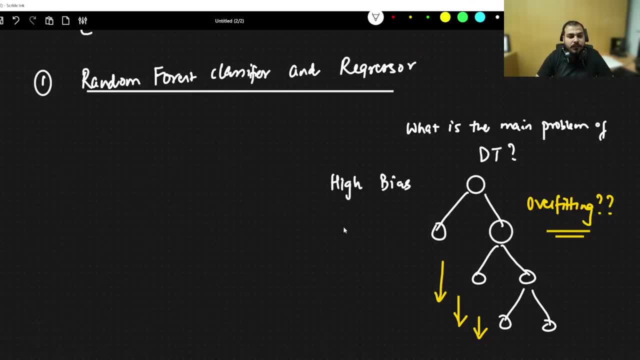 basically say it as high bias, okay. and then i may basically say it as sorry, not high bias. low bias and high variance. low bias and high variance, okay. so low bias and high variance. yes, obviously we can do pruning and all guys. but i again understand, pruning is an extensive task, probably if you're, if you have 100 features, if you have 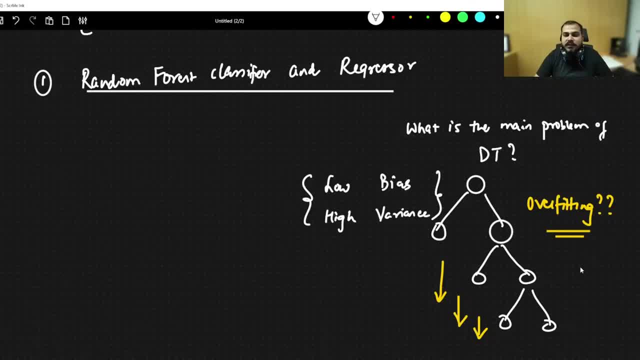 data points, which is like 1 million. to do pruning also, it is very much difficult. yes, pre-pruning can be done, but again we can do pruning, but again we can do pruning, but again we can do pruning but cannot confirm that it may work well or not. okay, so right now, with respect to decision tree, you 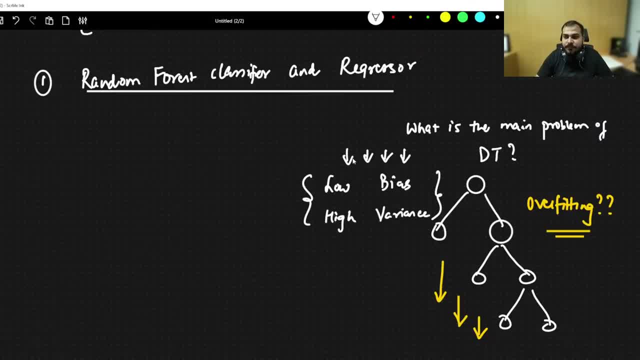 have this specific problem that is, low bias and high variance. okay, now in low bias and high variance. so you know that my model is basically the generalized model that i should get. it should have low bias and low variance. so if somebody asks you, why do you use random forest, you can. 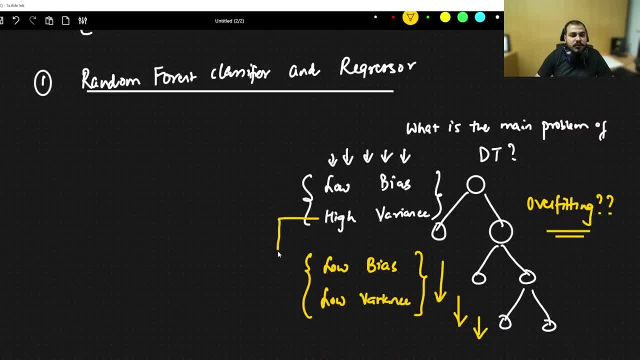 basically explain about decision trees like this. now my main aim is to convert this high variance to low variance. now i will be able to convert this high variance to low variance using random forest classifier or random forest regressor. now, what does random forest do? random forest is a bagging technique. 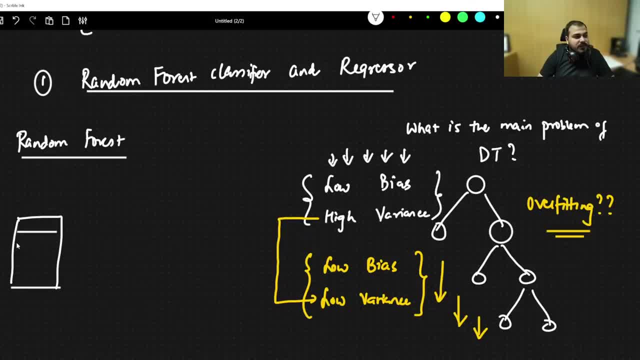 similarly, i have a data set over here. let's say that i have this data set, okay, and then here i will be having multiple models like m1, m2, m3, m4, m4. let's say, i have these four models like this, we'll have many, many models, okay. 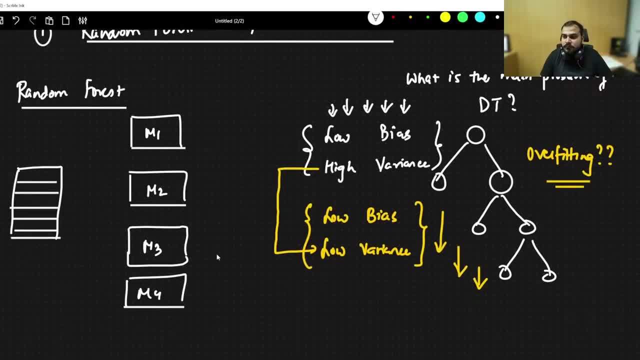 okay, now, with respect to this models, this models, all the models, are actually decision tree in random forest. all are decision trees. you don't have a different model over there, okay, so over here you can see that all the models are decision trees and you can see that all the models are decision trees. 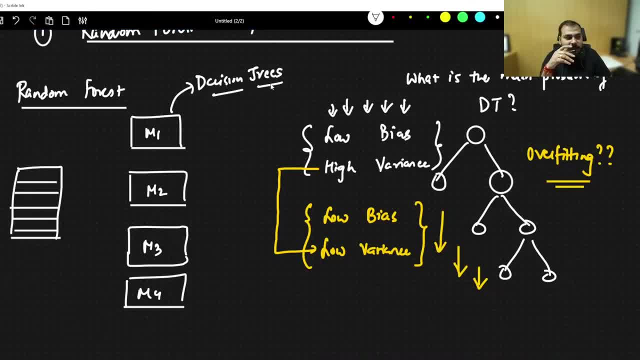 of decision trees that is going to get used in random forest. okay, so decision trees always gets used in random forest. the first thing that you should know now: whenever we are using decision trees, you know that decision tree if i by default. if we try to create it, it may lead to overfitting. because of that, every decision tree will basically create low. 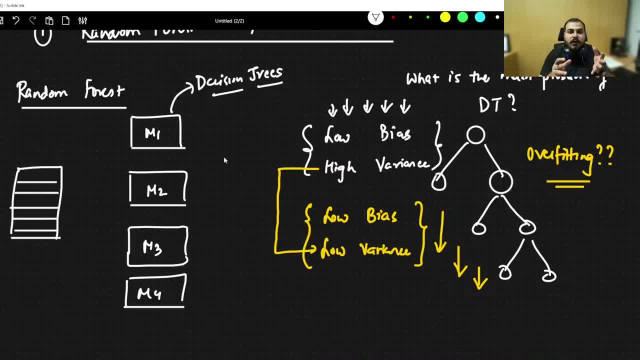 bias and high variance. but if we combine in the form of bootstrap aggregator, this high variance will be getting converted to reaccumulated and it would show like that in subject, in the background, and if you tit CAV here as well as in idiav: low variance because why? because majority of voting we will be taking from this particular. 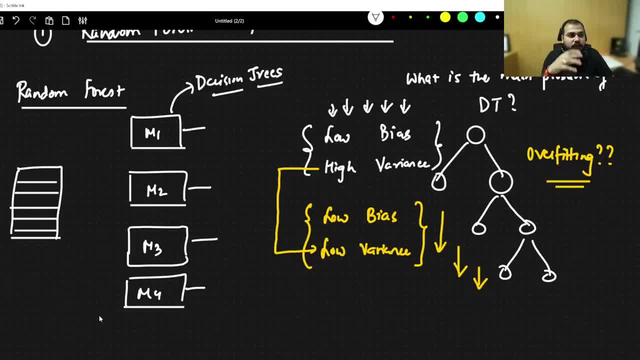 decision trees, like there will be many, many decision tree, so there lot of outputs will be coming and, with the help of majority voting classifier, this high variance will get converted to low variance. now in random forest, how it works in the first case, if i talk about random forest, 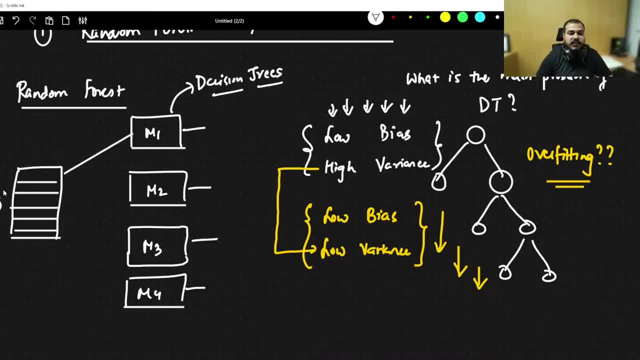 over here. two things basically happen with respect to the d dash data set. let's say, in first model we do some kind of row sampling plus feature feature sampling. that basically means we have to select some set of rows and some set of features and give it to m1. similarly you do. 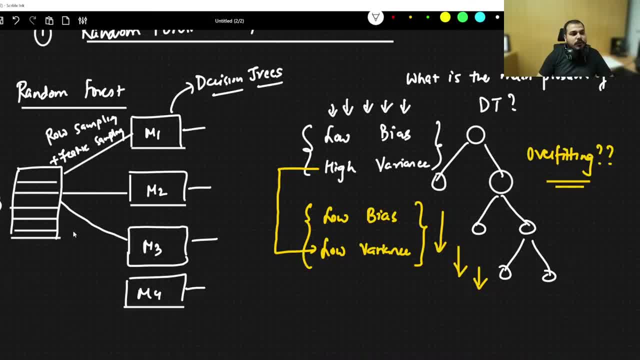 row sampling and feature sampling and give it to m2. then you do row sampling and feature sampling, you give it to m3 and then you do row sampling and feature sampling, you give it to m4. okay, now, when you do this, so what will happen? independently, you are giving. 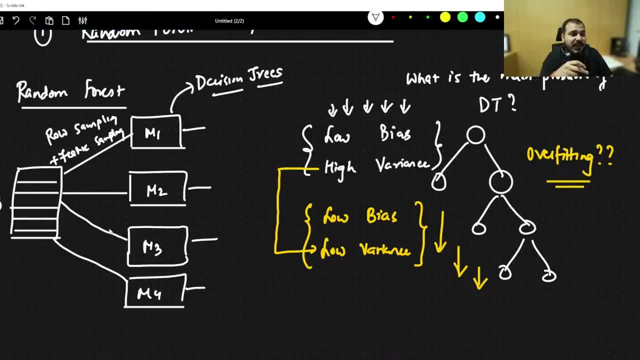 some features along with some rows. now there may be a situation that your features may also get repeated. okay, it may also get repeated. your records or data points may also get repeated. okay. so when you are probably training your model with this specific data sets and specific features, this model become expert in predicting something right, as i said. one example: 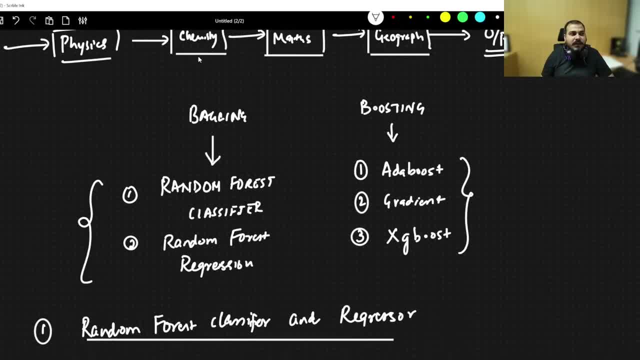 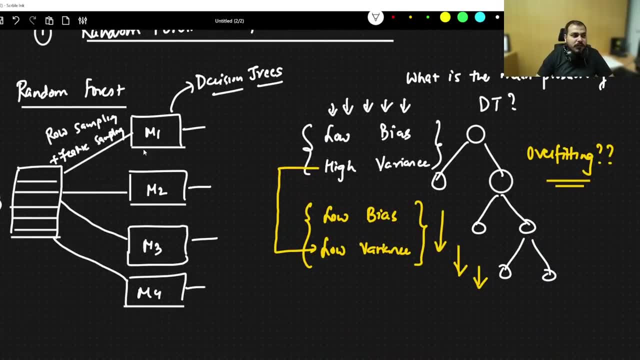 over. here i'm giving a physics model, some data. i'm giving chemistry data, chemistry model with some data. similarly, here i'm giving some information to some model, so the model will be an expert with respect to that specific data. so, based on all this particular data, whenever i 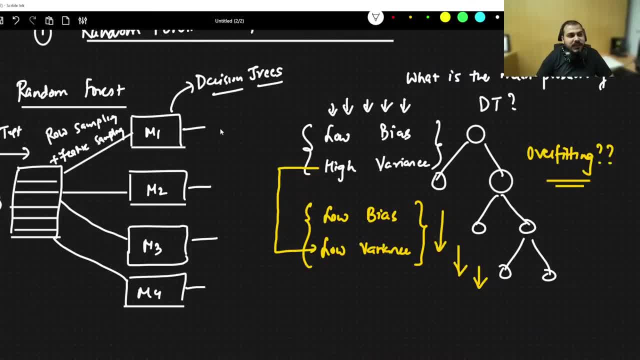 get a new test data. so what will happen? suppose let's say that this is a classification problem- the m1 model will be predicting zero, this will be predicting one, this will be predicting zero and this will be predicting zero. now, in this particular case, again, the majority voting. 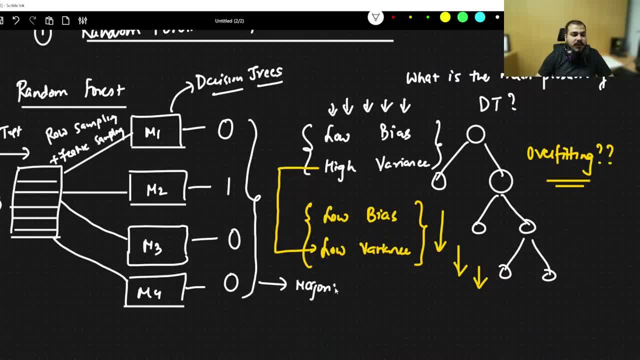 classifier of majority voting will happen in the case of classification problem, and then here you will be specifically able to get the output as zero. okay, so i hope everybody is able to understand. all the models over here are decision trees and based on that you will be doing: see, when i'm in an interview should be very, very. 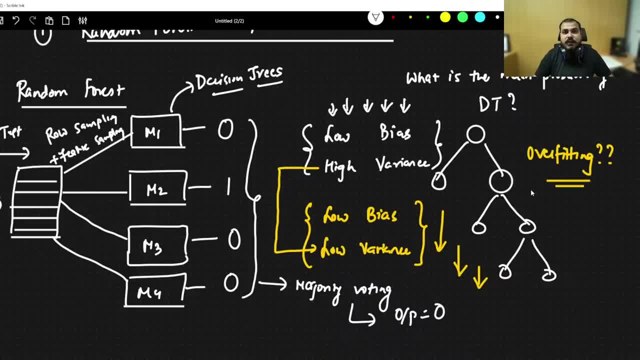 things. the things that i'm telling you over here is all. all the points are very much important and, similarly, if you tell the interviewer definitely your interview is crap in this kind of algorithm, i've seen some of my students saying that: okay, krish. when the interviewer asked me that which is my favorite algorithm, i said random forest. i told 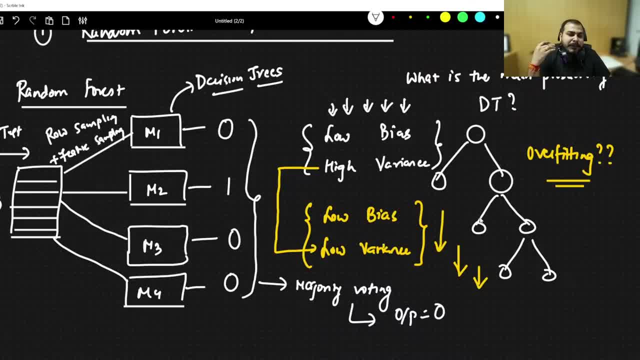 why did you say like that? because he said that, because that person- let me let him ask any questions in random forest. i'm very much confident about it and i'm also going to prove him. you know why they are very, very good. okay, so with this specific case here, you can basically see that. 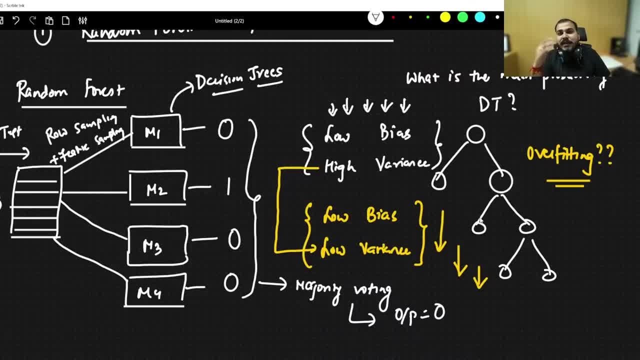 because of the overfitting condition of the decision tree. you're combining multiple decision tree so that you get a generalized model which has low bias and low variance. okay, so i hope everybody is able to understand boost feature sampling basically means suppose if i have one, two, three, four feature for the first model, i may give two. 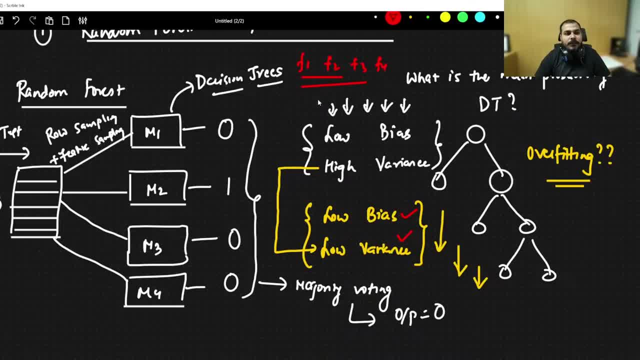 features. for the second model i may get three features. okay. for the fourth model i may give four features or any one feature also i can give to a specific model. so internally that random forest it take cares of, okay, so over here these things are there and this is how random forest works. only the difference between 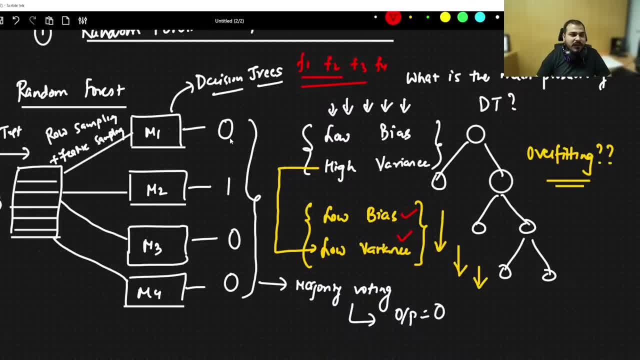 random forest classify and regression is that, in regression again, whatever output you are basically getting, you basically do the mean, that's it average. you just do the average. you'll be able to get the output okay based on all the models output that you are actually getting. okay now, 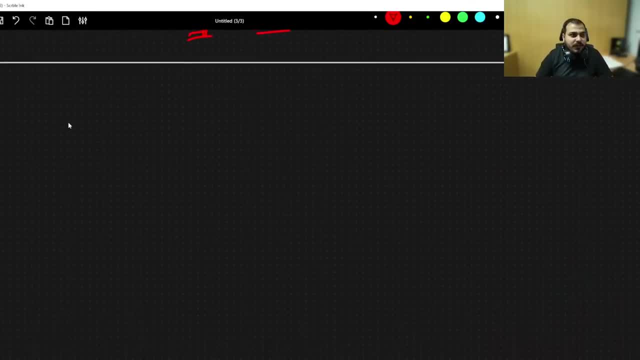 let's talk about some of the important points in random forest, random forest. the first thing first: is normalization required in random forest? is normalization required in random forest? the answer: what it is, you tell me. then the next question is that in knn, is normalization? when i say normalization or standardization, i'll i'll just talk about standardization. 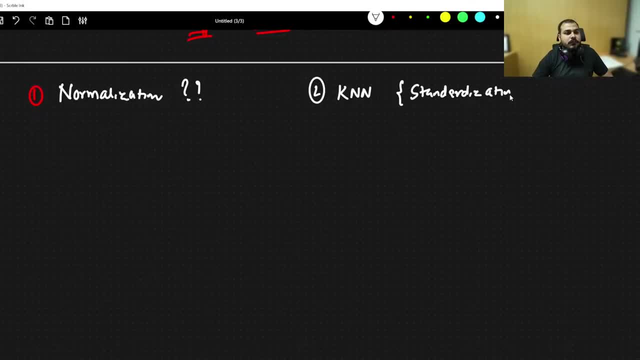 is standardization is required. so this will be my another question. so is normalization required in random forest? is normalization or standardization? i'll just talk about standardization in random forest or decision tree. you here, you can also say it as decision tree- is it required? okay, so for this the answer will be no, because understand decision tree will. 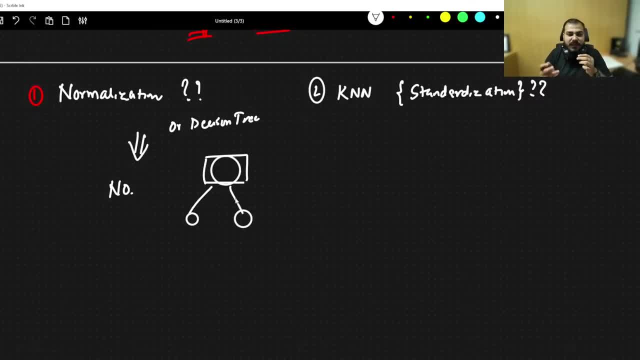 basically do the splits right. if you minimize the data also, that split won't be that much important. but if i talk about knn, either standardization, normalization, required over here, the answer is yes, because here we use two things. one is euclidean distance and manhattan distance. 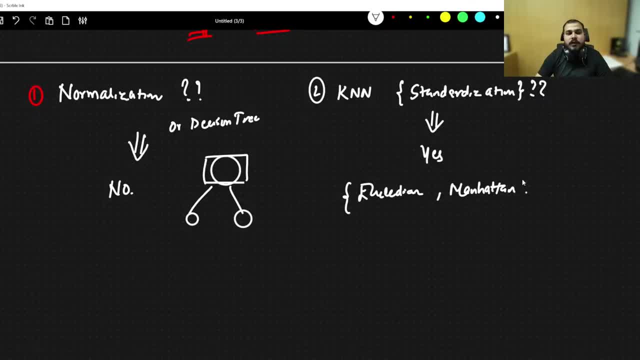 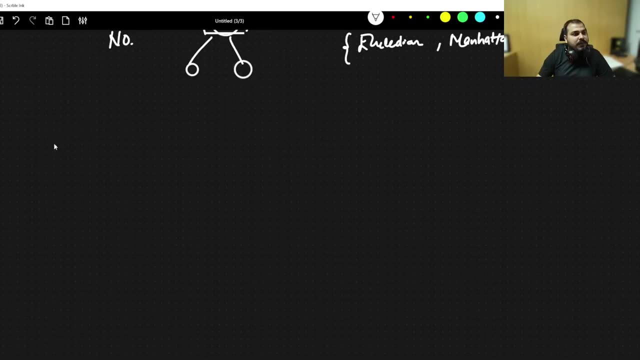 okay, manhattan distance. because of this, you definitely have to you apply standardization so that the computation or distance becomes easy. okay, so this is one of the most common interview questions that is basically asked in random forest. coming to the third question: is random forest impacted by outliers? is random forest impacted by outliers? tell me? 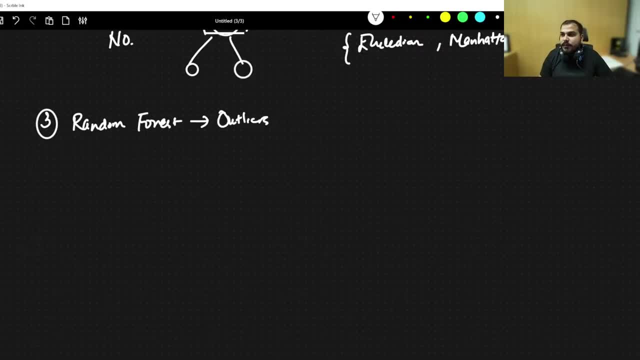 the answer: everyone, what should be the answer for this is: random forest um impacted by the outliers. okay, over here. over here, the answer will be no, just check it out. okay, why check it out from your side? i've already uploaded a video that is not over here, so go ahead. 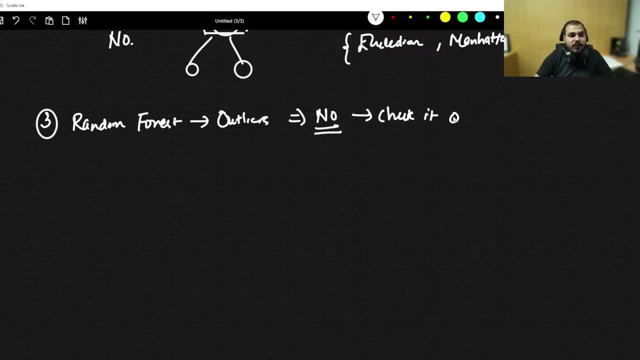 and go ahead and click on it and click on it and then go ahead and push that button. here you go, okay, do that, and then click on the start button and then click on submit video on this also. check it out outside basically means google and check it out. check it out in. 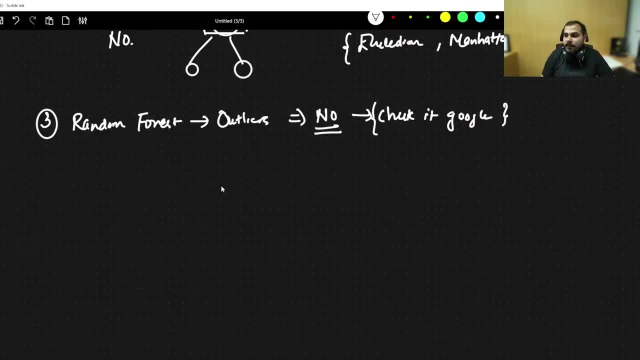 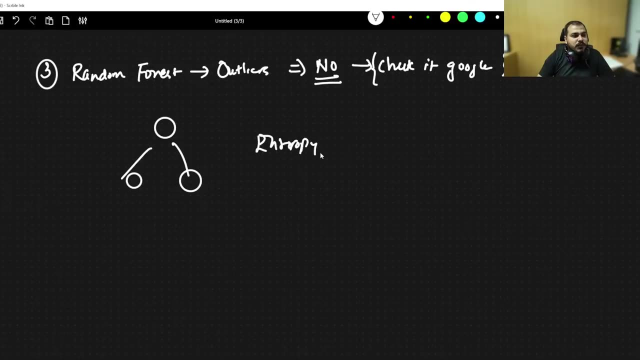 google. okay, okay, perfect. so i hope i have covered most of the things in random forest. now the reason i did not discuss about decision tree, how the decision tree is constructed, how entropy is used, how guinea is used- everything i have discussed yesterday. so that is the reason why i am directly. 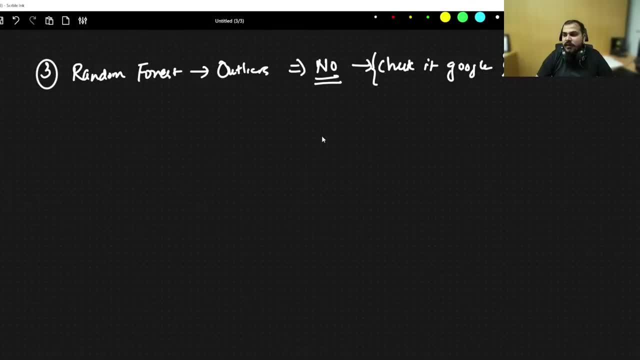 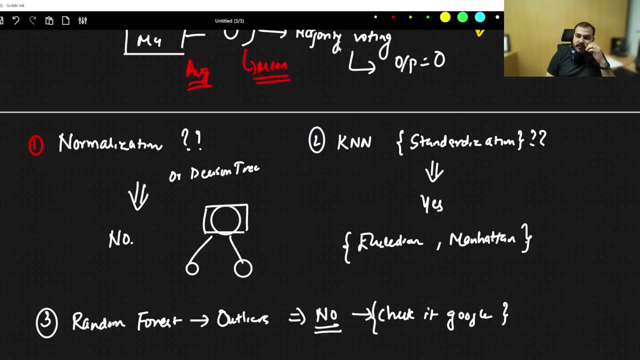 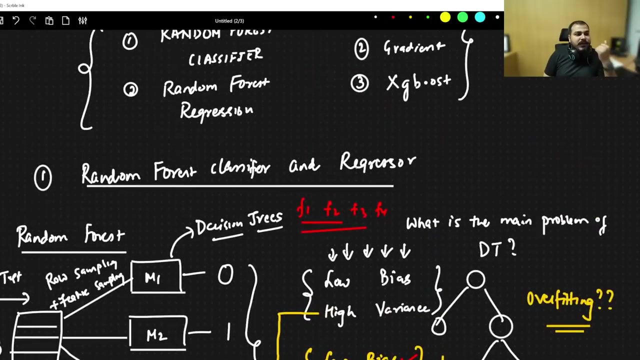 taking like this. so i hope you have enjoyed the session till now. okay, so one thing is that, because it gives equal opportunity to all the features by selecting randomly perfect. yes, sir, z score and standard scalar is same. yes, for standardization process you use z score. okay, so everybody clear with random forest and regressor. i hope you like this session till now. 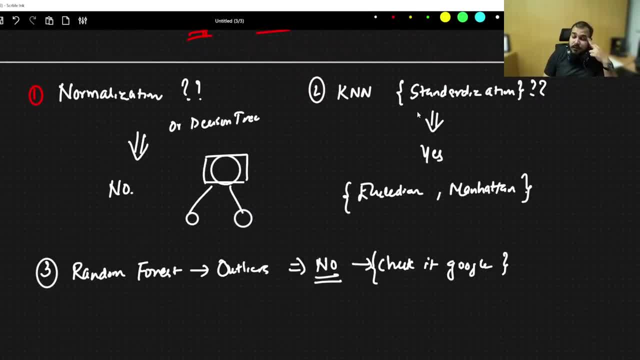 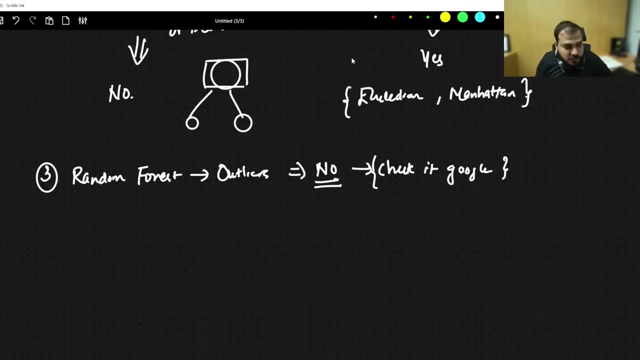 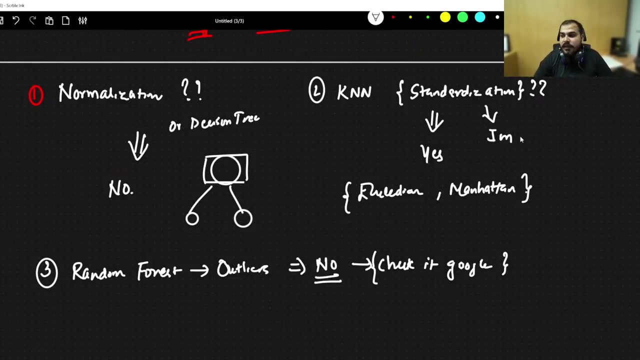 okay, guys, for outliers, because it gives an equal opportunity to all the features by selecting randomly, right. so because of that, is random forest impacted by outliers? this is the third question. okay, is knn impacted by outliers? is this knn algorithm impacted by outliers? so what should be answer? what should be answer: is it impacted by outliers? 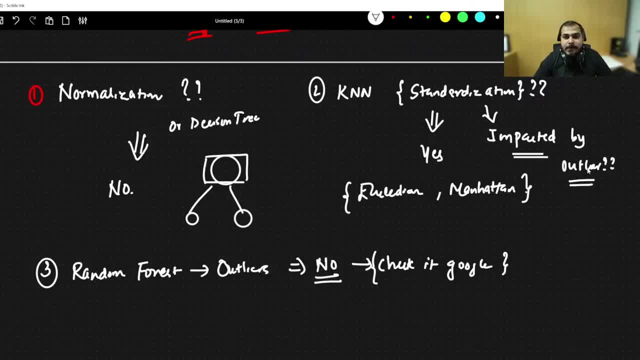 is knn impacted by outliers? the answer is yes, big yes, okay, i have also shown you this specific part also. okay, yesterday or day before yesterday, i think. okay, perfect, so these all are the interview questions that needs to be covered. so i hope you have enjoyed this session till now. i hope you have. 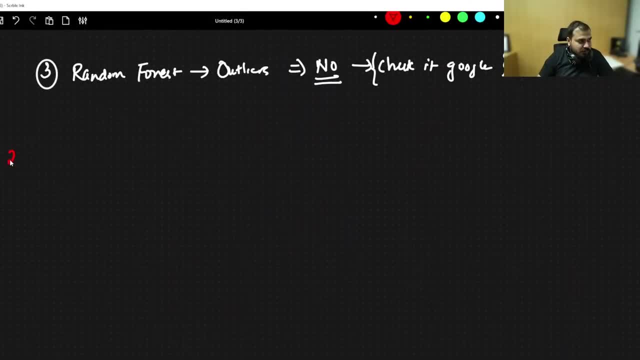 now let's go ahead and discuss about ada boost, the second one now. in bagging, most of the time we specifically use random forest. random forest- okay, or you can also create custom bagging techniques, okay. custom bagging techniques means whatever algorithm you want. use the combination of them. 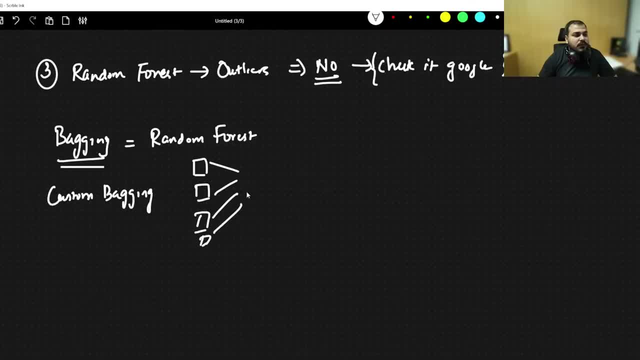 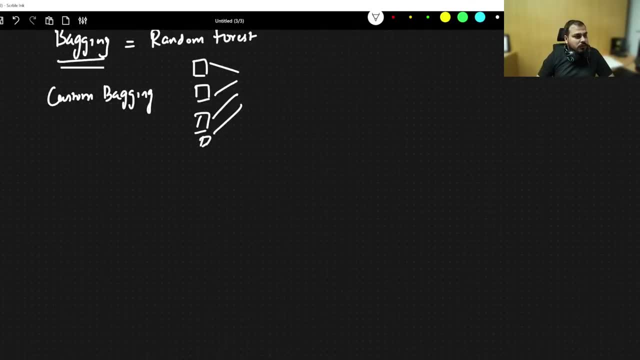 and try to give the output. okay, try to give the output. this also, you can do it manually with the help of hands. okay, perfect, so let's go. today we are. we are going to just give me a second, guys, today we are going to give you a second. tried a second one. 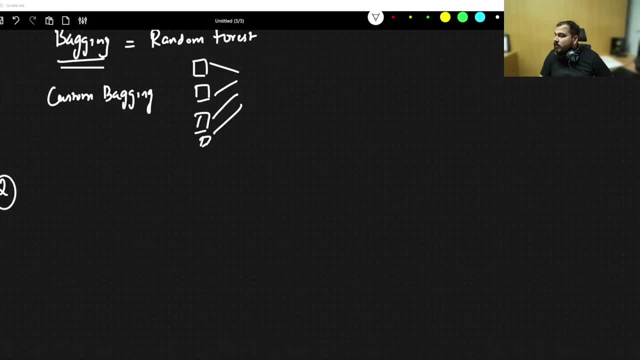 so now you can decide. you can add in me this list, these three 4 differentija, so let's go ahead and start, as we worked through this experiment so you can use your keyword. here is we call it, we will call this snow and i have 2 words: wii. 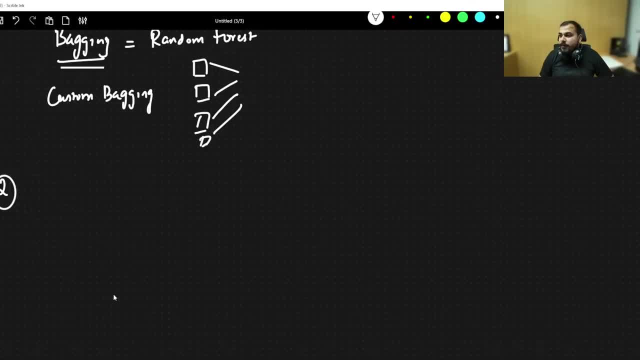 we will call it the custom bagging method, which is the tool that we are going to use for custom systems. ida is a wenthis tool, so this is the first one that we haveне do yet. bookmark is not one of them. you need to Suscribe to my channel. 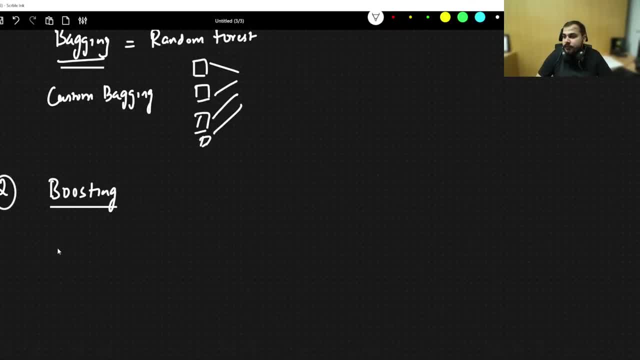 are going to discuss about is boosting technique, and this, the first thing, that first algorithm that we are going to discuss about is ada boost. okay, so ada boost. we are going to discuss about how does ada boost work? but till here, did you understand nicely? everyone is it interesting? 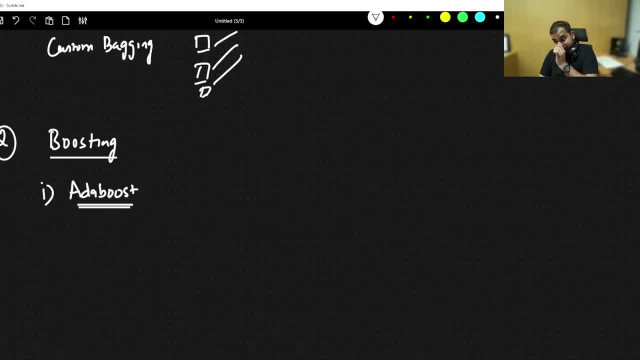 or not? anjan, uh, customized bagging techniques. take the data set. they apply a sampling code. give only those data set to your one model. right, a simple sampling techniques can actually help you understand all those things. yeah, perfect, perfectos. uh, we will solve a problem with respect to ada boost. just give me a second. 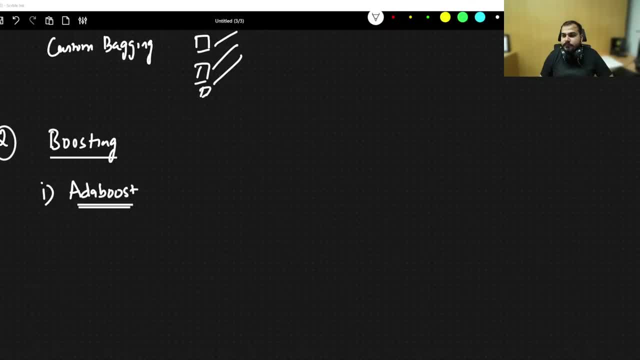 just a second. give me a second. i'm just trying to open my notebook. okay, now let's solve, uh, the first boosting technique, which is called as ada boost. okay, and uh, this is a boosting technique. um, in the boosting technique, you have heard that we have to basically solve in a sequential way. okay, this at least you know, i know there. 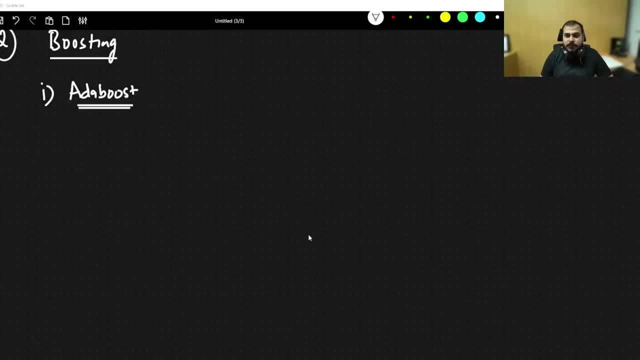 is a lot of confusion within you all, but we'll try to solve a problem. let's say: okay, so suppose i have a data set which looks like this: f1, f2, f3, f4, so these are my features. so let's say that i am having these features and probably these are my output. okay, so let's say that. 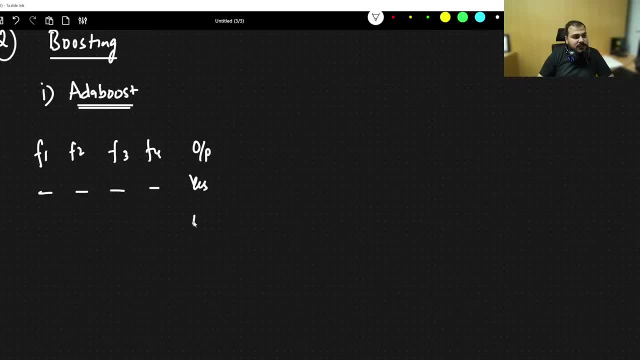 i am having these features like this and this is my output- like yes or no, like this, okay, so let's say that how many records i have over here? three, four, five, six and one more, is there seven? okay, so this seven records are there now in ada boost. the first thing is that. 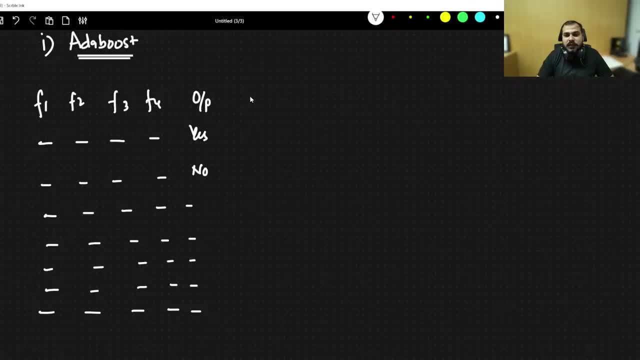 specifically with ada boost. uh, you really need to understand that, what all things we can basically do. okay, how do we solve this classification problem that we are going to understand the first thing first is that we define a weight, okay, in this, and the weight is very much simple. initially, to all the records, to all these input records, we provide an equal weight. 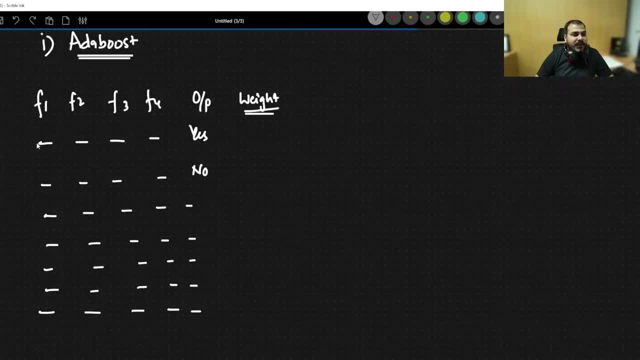 now, how do we provide an equal weight? we just go and count how many number of records are there now, in this particular case, the total number of records are one, two, three, four, five, six, seven. now every record i have to provide an equal weight. that is between zero to one. 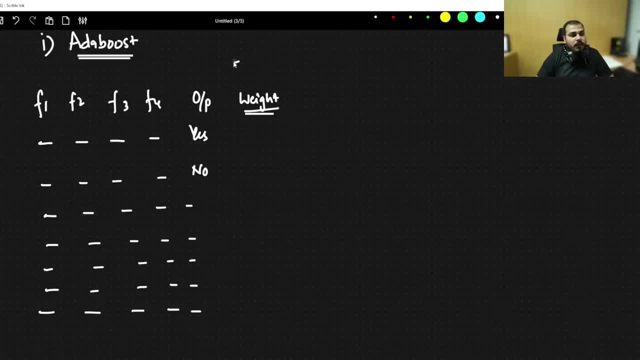 so the overall sum should be one, okay. the overall sum of the weights should be one, okay. so, in this particular case, what i can do, if i make one by seven, one by seven, one by seven to everyone, this will definitely become a before one. okay, therefore, that is now Hinterstones. 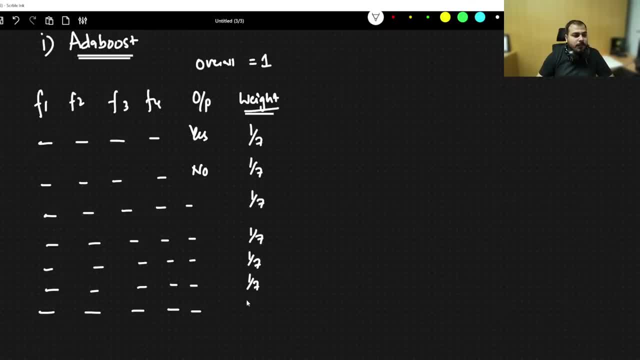 i can add and subtract to each row, then i can subtract one and i can put multiplying the weights, so it is one, three, four, five, six, seven and the one i am relativelyll over one. i am equal weights to all right and if i do the total sum it will obviously be one, right, i hope. 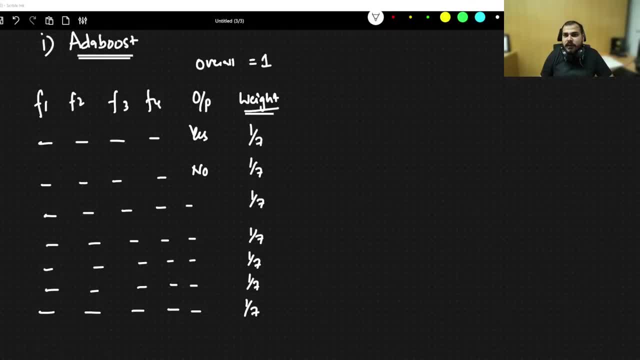 everybody is able to understand. till here, right now. let's go to the next one now. after this, what do we do? okay, after this, in adaboos, the first thing that we do is that we take any of this feature. how do you decide which feature to take, whether we should go with f1 or whether we should 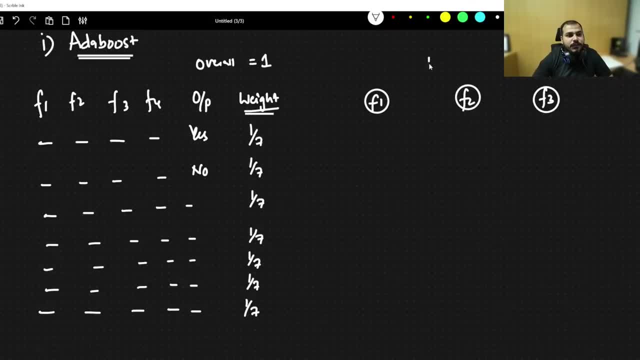 go with f2 or whether we should go with f3. this we can do it with the help of information gain and information gain and entropy or guinea right. based on this, we can definitely understand whether we should start making decision here. also, you specifically make decision trees, okay, decision. 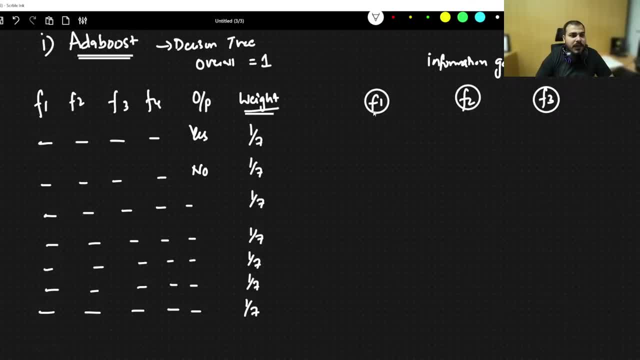 trees. so here, what you do is that you probably have to determine by using which feature i have to start my decision tree. okay, so suppose, out of all this, we have a decision tree and we have a decision tree and we have a decision tree, feature one, feature two, feature three: you have selected that. okay, the information gain and 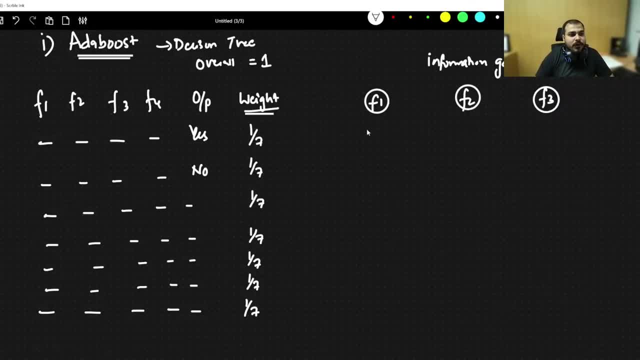 entropy of feature one is higher, so i'm going to use feature one and probably divide this into decision trees. now, when i divide this into decision tree, let's say that i'm dividing like this into decision tree- this decision tree depth will be only one, one depth, and this depth, since 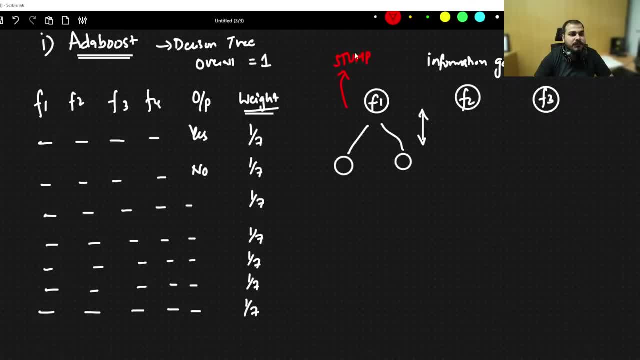 it has only one depth. we basically call it as stumps. okay, we call this as stumps, okay. so what we do over here specifically: we call this as stumps, okay. so what we do over here specifically: we will create a decision tree by taking only one feature and we will only divide it to one level. 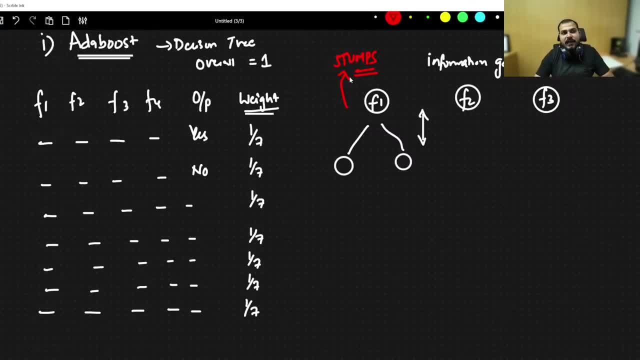 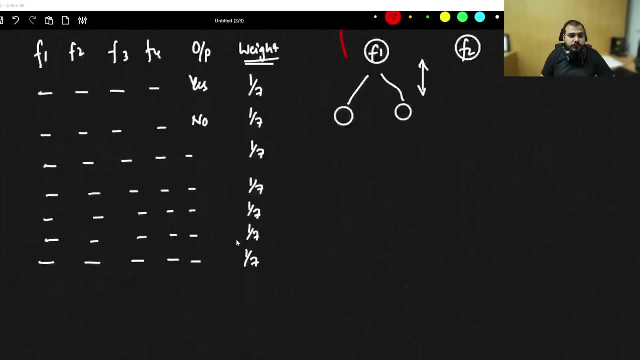 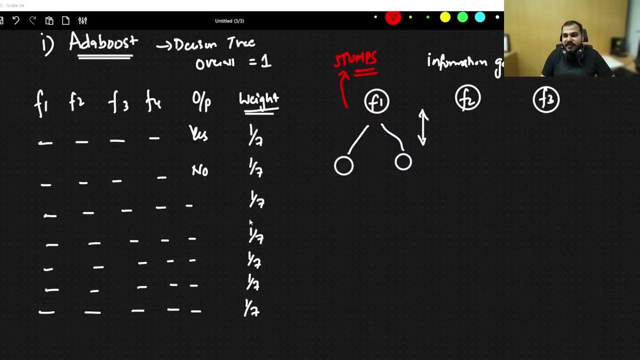 okay, one level or one depth, that's it, and this is specifically called as stump. okay, i hope everybody is able to understand till here. yes, quickly tell me, i hope everybody is able to understand till here. now, what we are going to do next is that from this particular stump- okay, the stump is basically getting- 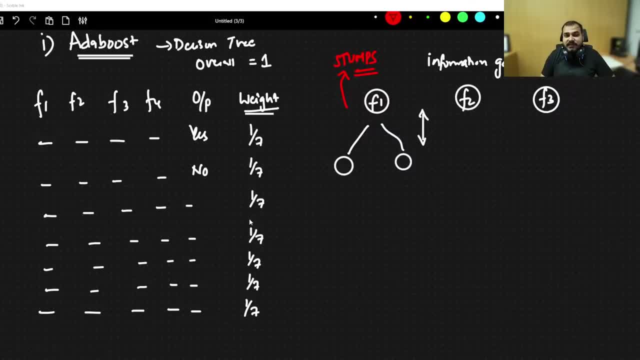 getting created only one. so that is ada boost. right, we say it as weak learners because this is weak learner, okay, weak learner. why that? there is a reason. we say this as weak learner, okay, so, only weak learner. so that is the first thing with respect to, uh, this particular ada. 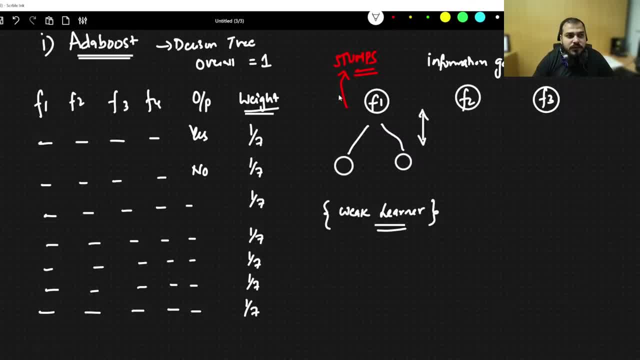 boost. okay. so the first step is that this is a weak learner. so for the weak learner, we basically create a stump. stump basically means one level decision tree, that's it. okay, based on the information gain and entropy, i have selected the feature and then i just made a decision tree with 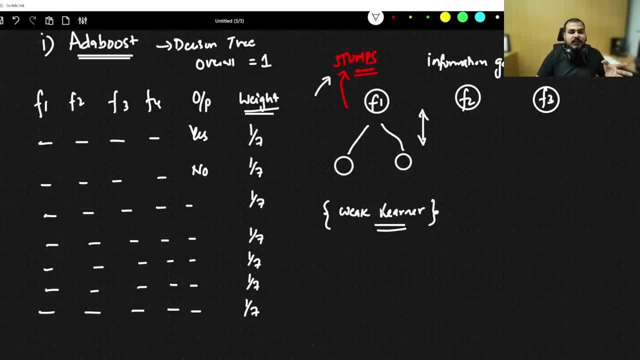 only one level. okay, why it is called as it is called: as weak learner, okay, so that is the reason we use only stump. that is, just a one level decision tree. now the next step happens is that we provide all these specific records to this f1 and we train this specific model. okay, only with one level decision tree, we train them. 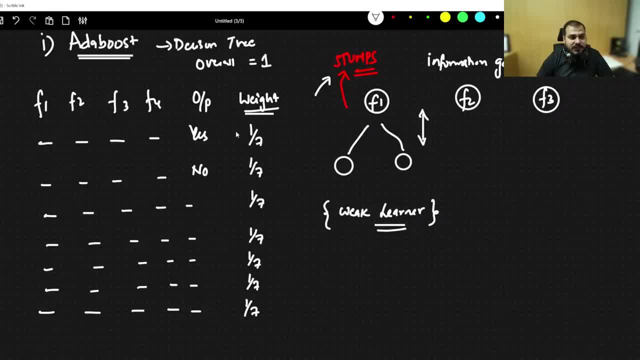 now, after we train them, let's say that we are going to pass all these particular records to find out how many are correct and how many are wrong. this decision, this decision tree, is basically giving okay. so let's say that out of this entire record is one record. one record was just given. 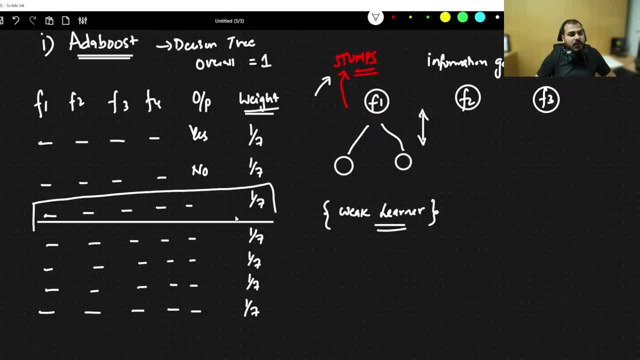 as wrong only one record this specific learner gave as wrong. okay, so let's say that, out of this entire record, one record was just given as wrong. let's say that this is the. this is the record which was given as wrong. okay, i will not say this, all this. 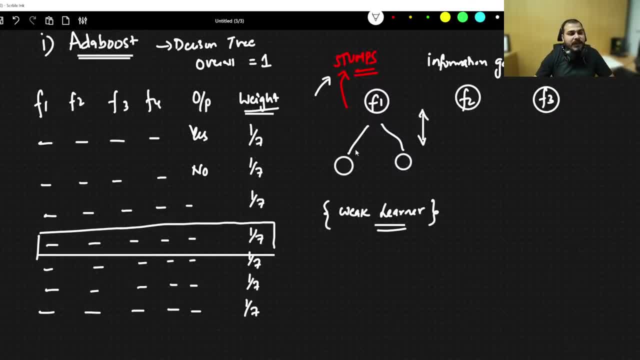 okay, so let's say that this record output was predicted wrong from this particular model. only one wrong was there after training the model. now what we need to do in this specific case, understand a very important thing. is that what we need to do after this? okay, so let's say that we have done. 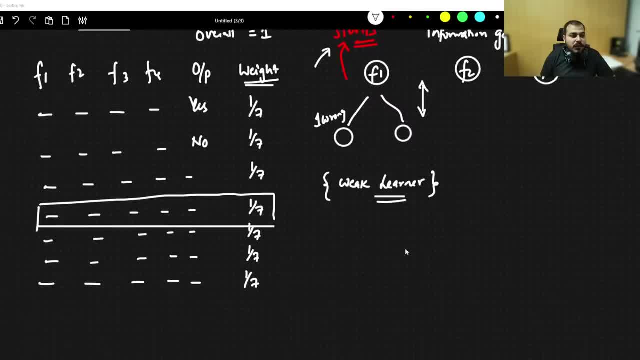 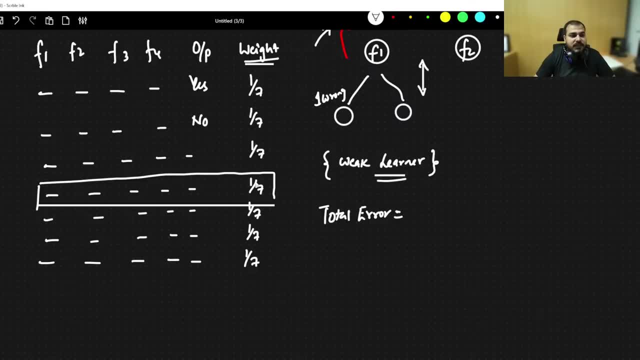 this, and probably after this particular model, we have done this, and probably after this particular model, we have done this, and probably after this particular model, we have done this and possibly after this, what we are actually going to do, we are going to calculate the total error. okay, so how many error this particular model made? let's say that in this particular case, only one was wrong, so this was only wrong. right, one was wrong. so if i want to calculate the total error, how will i calculate how many? how many of them are wrong? how many of them are wrong? only one is wrong. what is the weight of this? so i will go and write one by seven. so this is specifically my total error out of this specific model. okay, so let's say that in this particular case, only one was wrong, so this was only wrong. right, one was wrong. so if i want to calculate the total error, how will i calculate how many? how many of them are wrong? how many of them are wrong? only one is wrong. what is the weight of this? so i will go and write one by seven. so this is specifically my total error out of this specific model. okay, so let's say that in this particular case, only one was wrong, so this was only wrong. 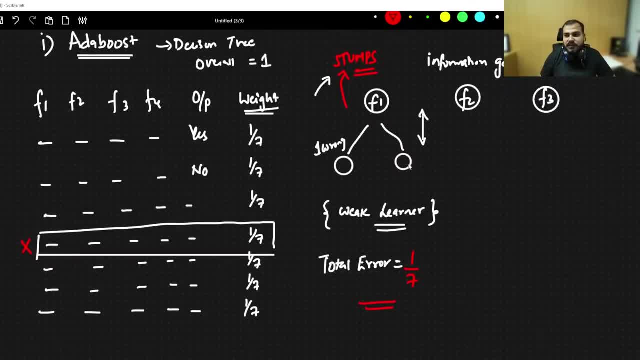 model which is my stump over here. okay, which is my f1 stump. everybody clear till here. just give me a confirmation now. this is my first step. the second step is that i need to see the performance of stump, performance of stump which stump this specific stump, and the performance is basically: 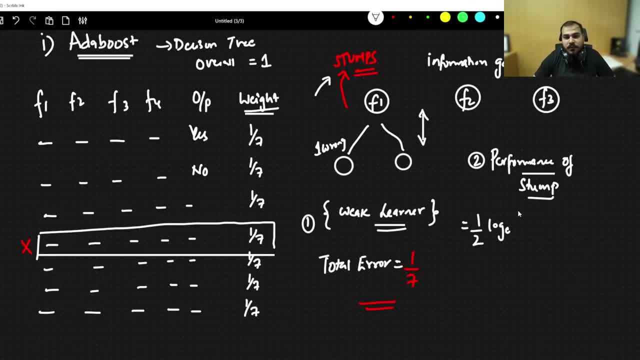 checked by a formula which is 1 by log e, 1 minus total error divided by total error. okay, why we are doing this? everything will make sense. okay, in just time, every, every, in just a small time, everything will make sense. the first step that we do in ada boost is that we try to find out the total error. 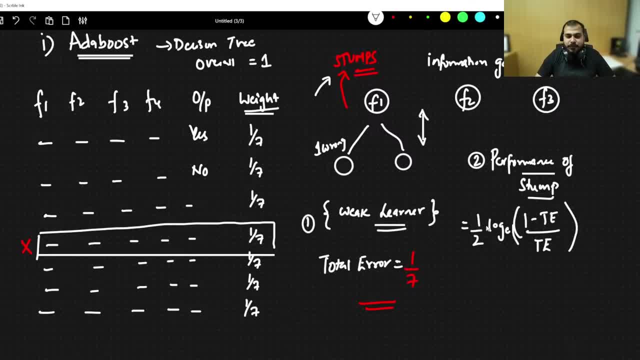 the second step, we try to find out the performance of stump. now, in this particular case, it will be 1 by log e, 1 minus 1 by 7, divided by 1 by 7. so once i calculate it, it will be coming as 0.895. you do it, you do the. 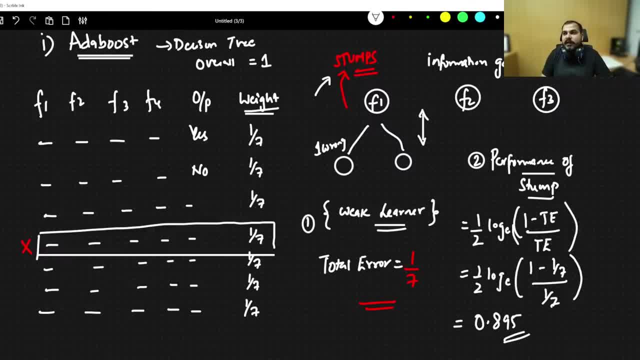 calculation and just let me know, okay, i'll give you time to write it down, because this is a little bit difficult, okay. f2 and f3. see again, understand, out of all these features, i found out from information gain and entropy that this is the best feature, okay. 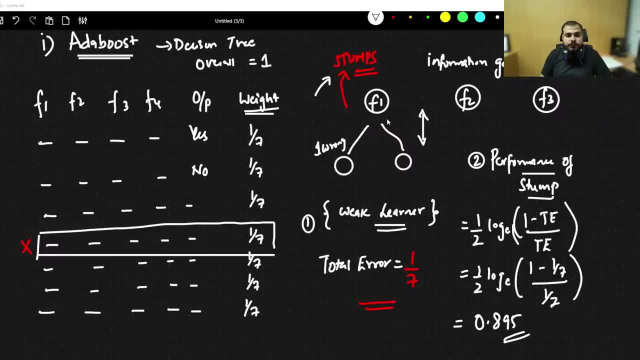 so let's say that i have calculated this as 0.895. so this is my second step. the first step is find out the total error. the second step is performance of stump. so i hope everybody is able to understand till here. can i get a quick like so that at least the like crosses 500? 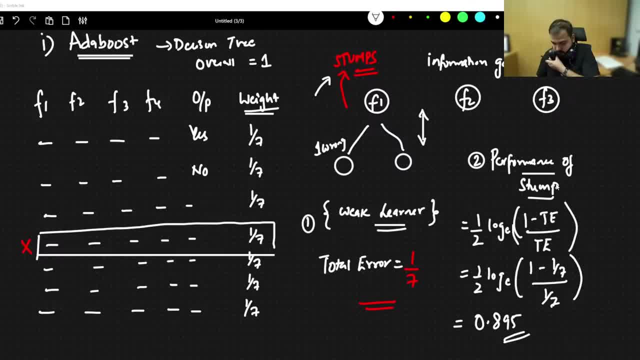 so the like should cross at least 500 now. come on, yeah, i'm, i'm putting so much of effort, you should also put some effort, right? what is t? e? t? e basically means total error. t? e basically means total error, okay, okay. fine, now, everybody is clear. till here. everybody is clear till here, okay, everybody. 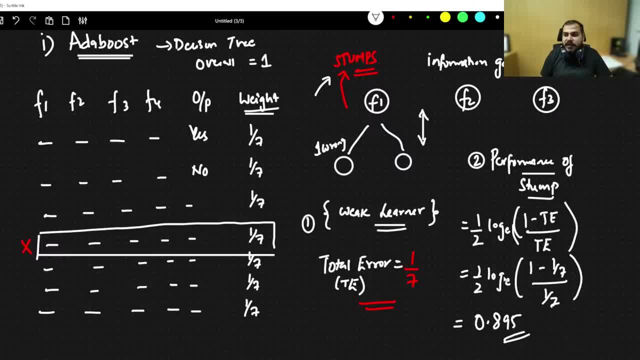 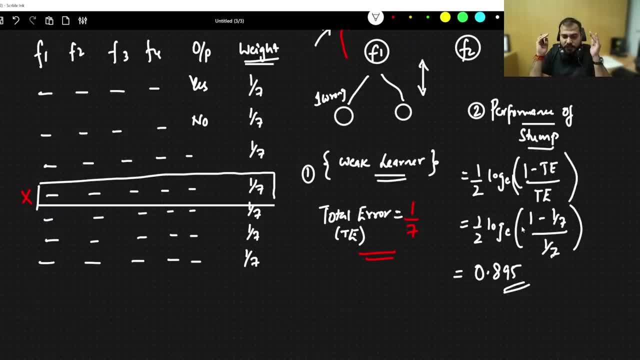 is clear till here. i hope everybody has got this. okay, so let's say that i have calculated this as 0.895. okay, now see, see the steps. okay, see the steps. understand: whenever i'm discussing about boosting, i'm going to combine weak learners together to get. 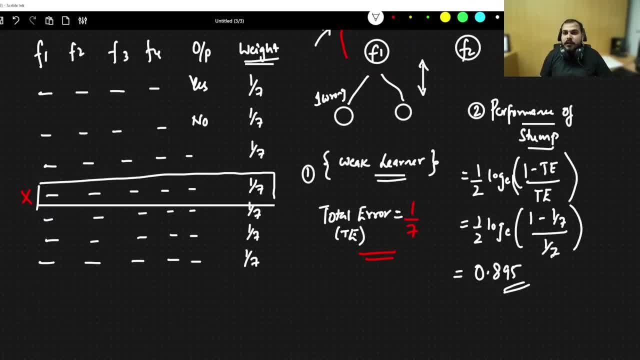 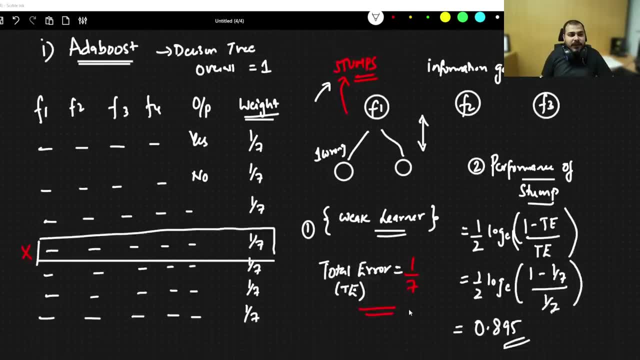 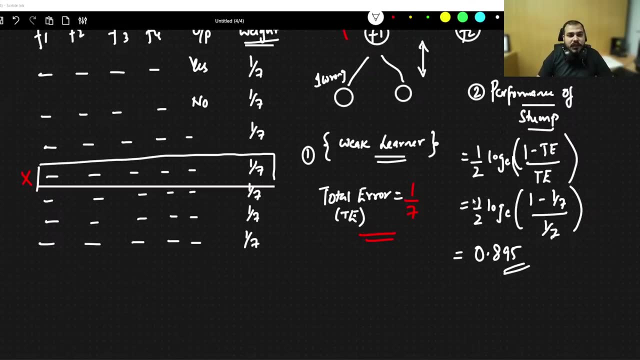 a strong learner. now, what is the next step out of this? now, what? what will be my third step? understand over here. my third step will be to update all these weights. to update all these weights- and that is the reason why i'm calculating this total error and performance of step. so my third step will basically be new sample weight from the decision. 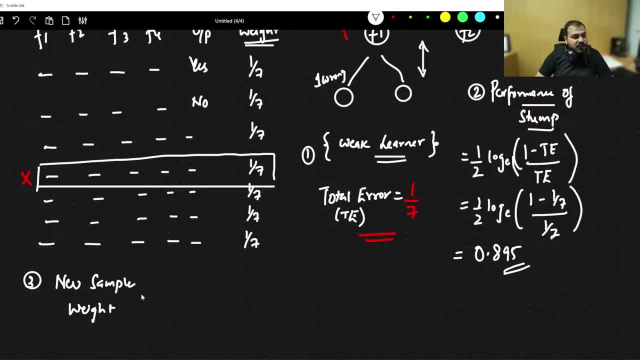 tree, one which is my stump. so i'll say: new sample weight is equal to: i need to update all these weights. why i need to update all these weights again understand, i'll talk about it just a second. so if i want to update the sample weights, first update. i will do it for correct records. 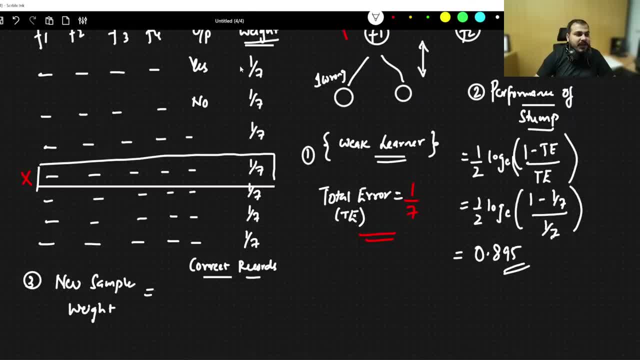 so see for correct records. whichever are correct, like this, all records are correct. this, all records are correct. you know this. all records are correct. now, when i update the weights of this way, update the weights of this particular record, it should reduce. it should reduce, okay. and when the the the wrong records. 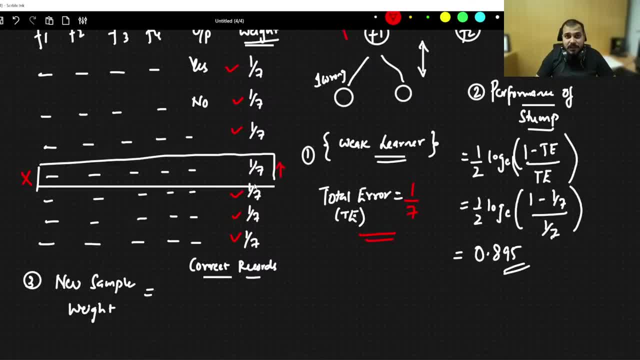 that i have this update should increase. why? because because if i increase these weights, then the wrong records that are there, that record should go to the next week learner. okay, that is the reason why i am doing it now: how to update this particular weights for correct records. for correct records, the formula looks something like this: 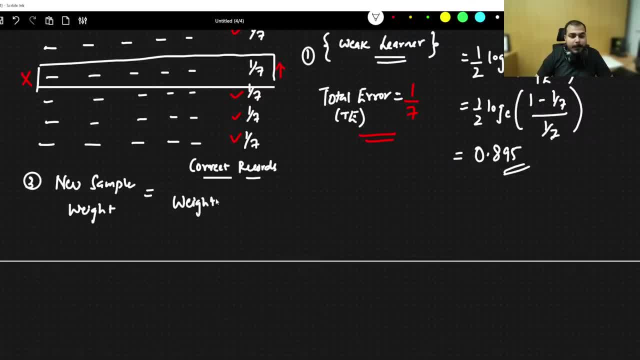 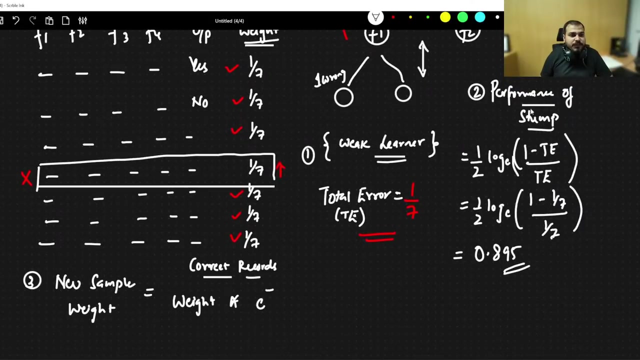 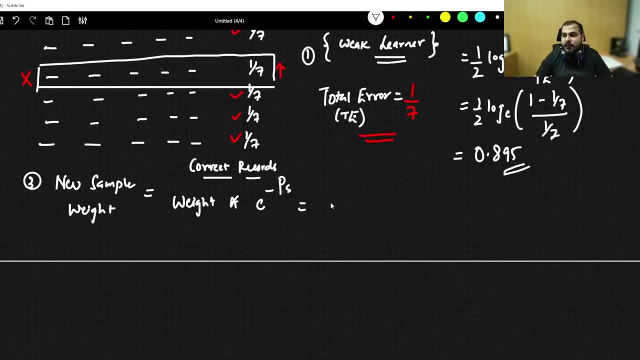 weight multiplied by just a second. let me check out the okay weight multiplied by e to the power of minus, this specific performance, okay, this specific performance, so e to the power of p, as i'll write, performance of stump, and then i will basically be able to write 1 by 7 multiplied by e to the power of minus 0.895, if i do the calculation everybody. 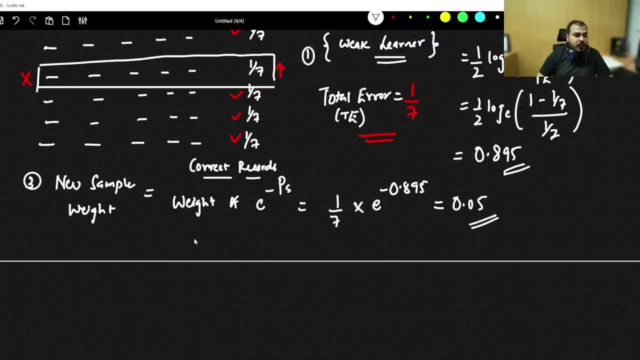 try to do it, the answer will be 0.05. okay, now, this is for correct records. what about incorrect records? for the incorrect records, the, the weights that is going to. the formula that we are going to apply is multiplied by e to the power of plus p s, not minus p s plus. 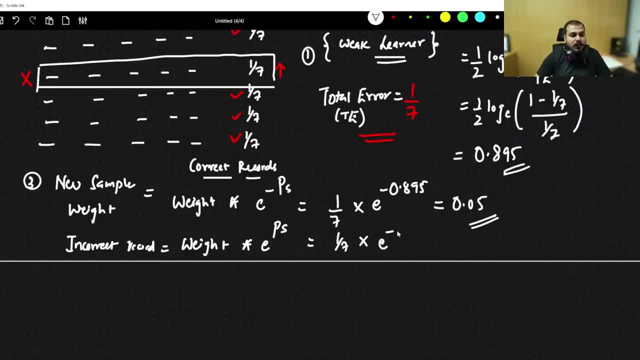 p? s. so here i'll write: 1 by 7, multiplied by e, to the power of e to the power of 0.895. so if i go and probably calculate this, i'm going to get it as 0.349. so these two are the weights that i have got. that basically means all these records now. 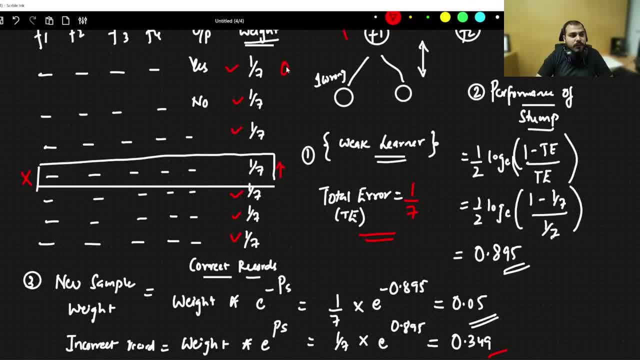 which are correct 1 by 7. the new updated weights will be 0.05, 0.05, 0.05, 0.05. sorry, not for the wrong records. then this will be 0.05, then 0.05 and 0.05. okay, so let me just see what is 1 by 7. 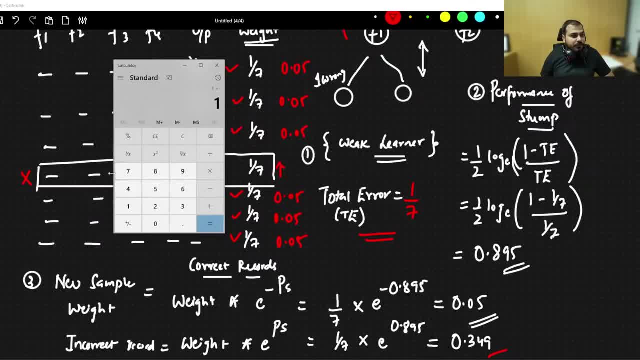 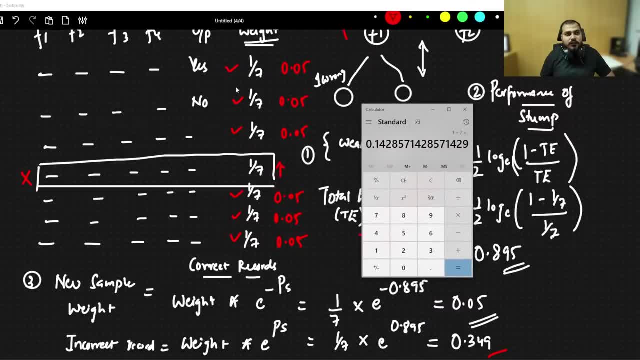 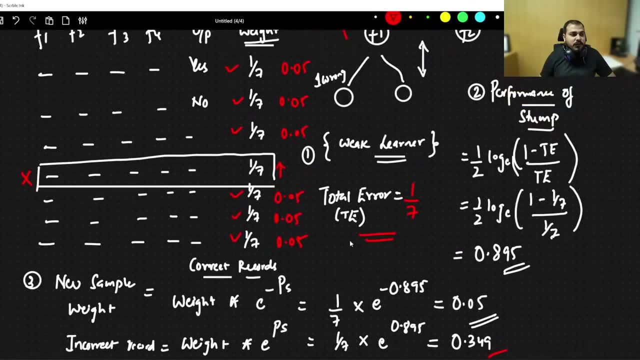 1 by 7, 1 by 7. so here you can see. initially it was 0.142, now it has got reduced to 0.05 because all these records are correct. okay, but the wrong record value is 0.349, so my weights will now become over here as 0.349. everybody clear till here. 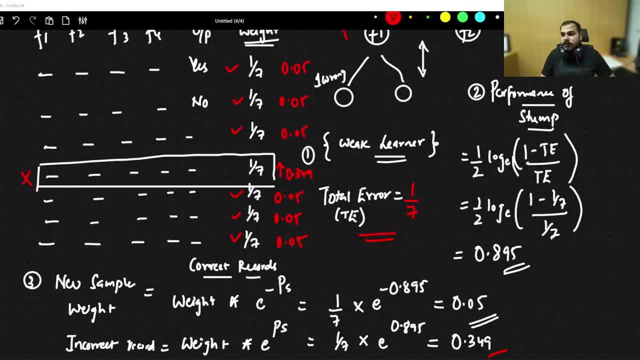 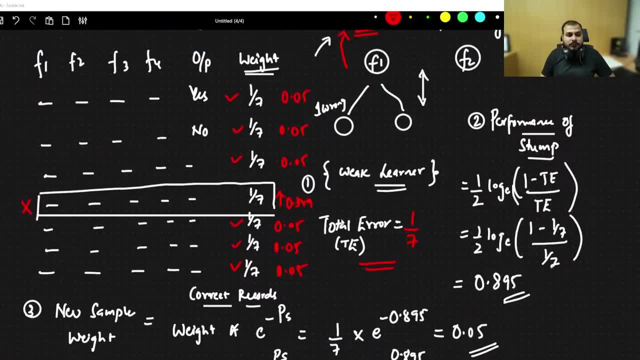 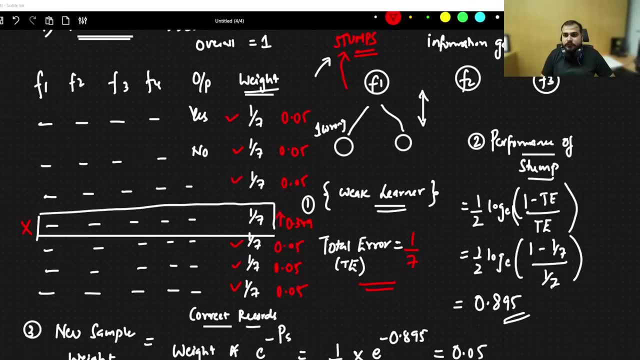 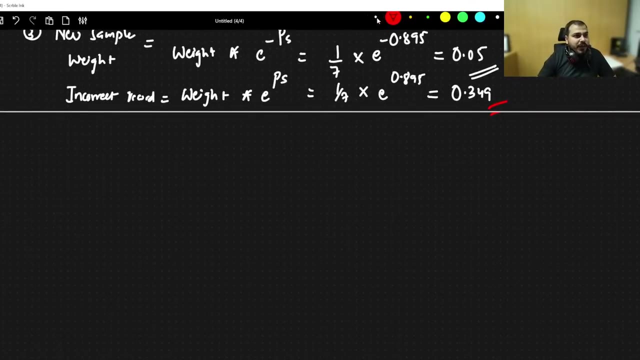 just give me a quick yes if it is, you got it or not. refractions, otherwise are they using Hall? okay, respect, 0.35. they are simply writing. I am going to give���amat 0.35, 0.35. now i am going give μέ. 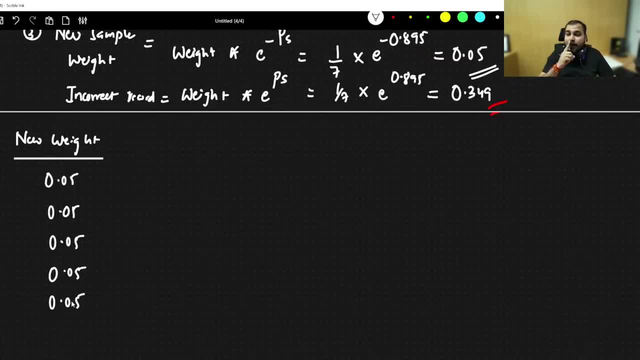 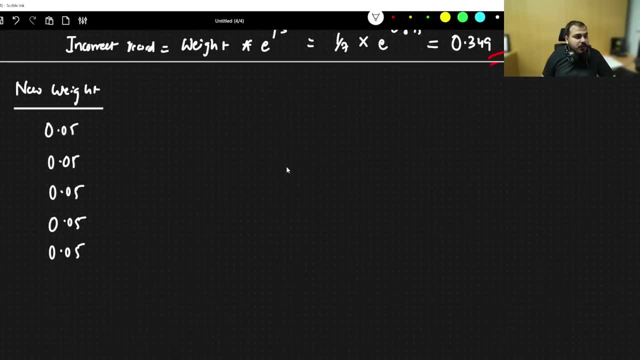 0.35, the new date: 0.35. zero videos to how many? one, two, three. okay, fourth record is here. fourth record: is there one, two, three, four, point zero, five, point zero, five. okay, how many records are there? one, two, three, four, five, six, seven. so my fourth record will basically become the new value that i'm having is something called. 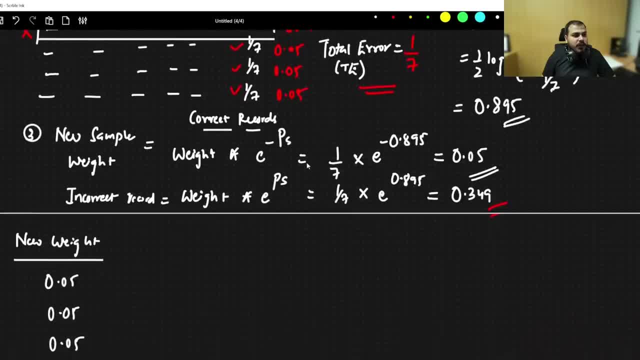 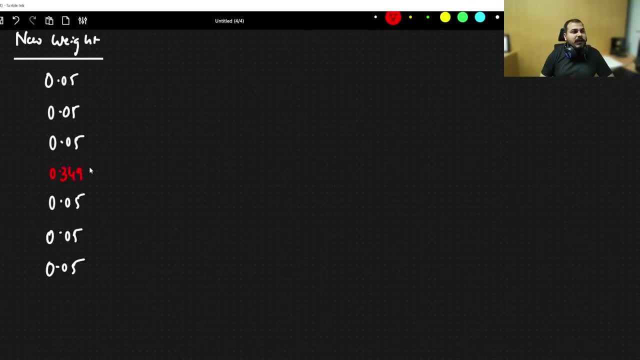 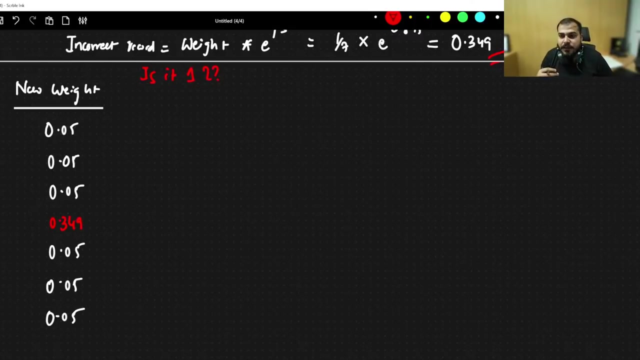 as point three, four, nine. okay, so point three, four, nine. now tell me, guys, if i do, the summation of all these weights is this, is it one? is it the summation one? is the sum summation one everyone tell me? is the summation one one? 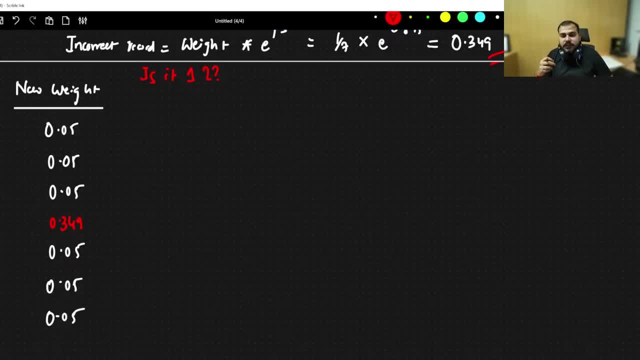 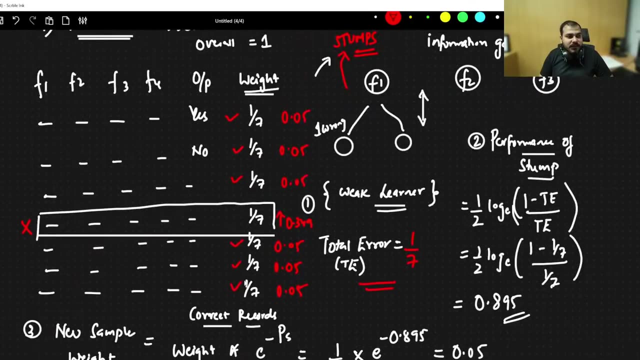 is the summation one. is it one? so probably no, i don't think so. it is one, because if i try to add it up it is not one, but if i go and see over here, these all are one. okay, if i combine all these things, one, two, three. 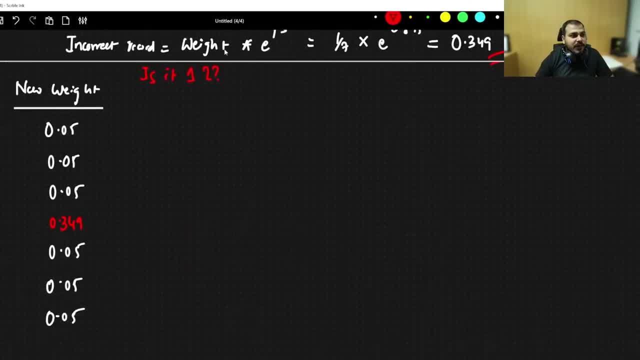 four, five, six, seven. these all are one. so here i have need to find out my normalized weight. now, in order to find out the normalized weight, all i have to do is i have to find out the normalized weight. all i have to do is i have to find out the normalized weight. 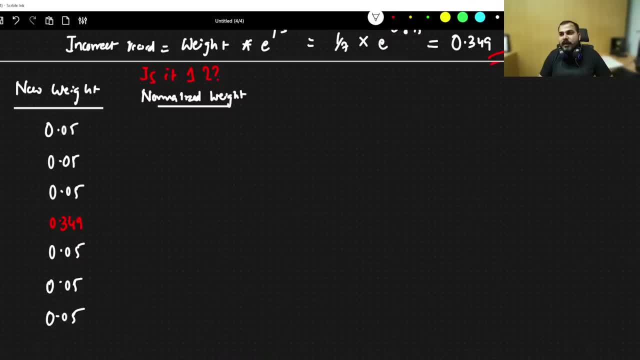 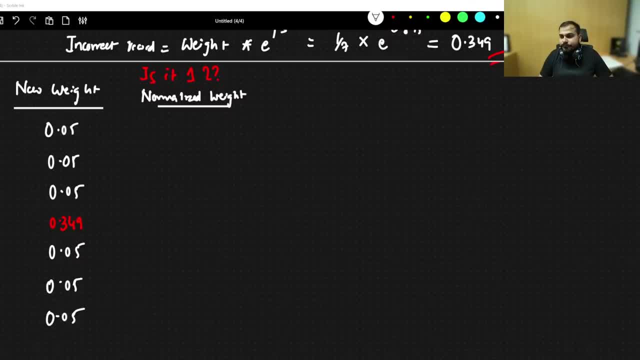 for finding out the normalized weight. tell me for finding out the normalized weight. tell me- think of it- what i have to find it out with respect to the, what i have to find it out with respect to the. what i have to find it out with respect to the normalized weight. 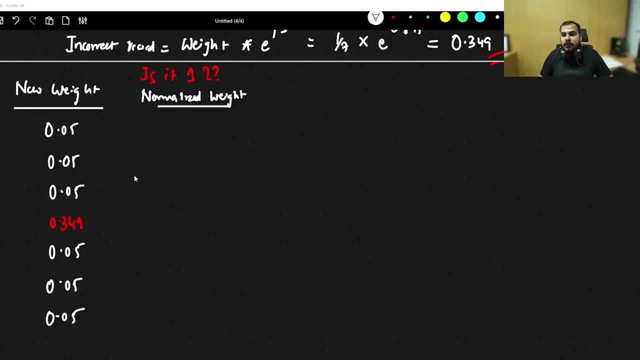 in order to find out the normalized weight, in order to find out the normalized weight, in order to find out the normalized weight. think over it, guys, what we have to do. think over it, guys, what we have to do. think over it, guys, what we have to do, because the entire submission should be one. 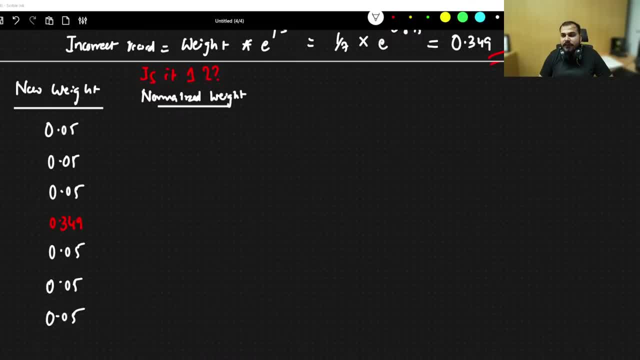 because the entire submission should be one, because the entire submission should be one. so we have to normalize, so we have to normalize, so we have to normalize. okay, we have to basically normalize, okay, okay, we have to basically normalize, okay, okay, we have to basically normalize, okay, now, in order to normalize all you have. 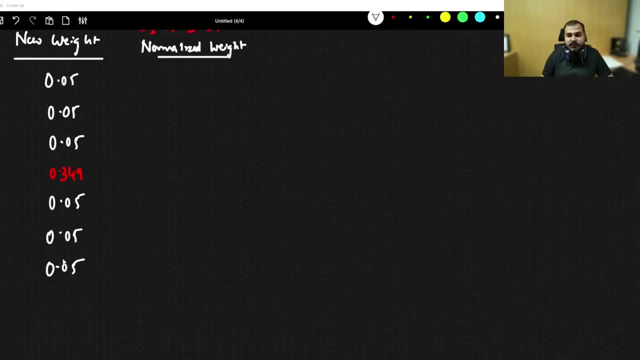 now in order to normalize all you have now. in order to normalize, all you have to do is that go and find out what is the to do. is that go and find out what is the to do? is that go and find out what is the sum of all these things? 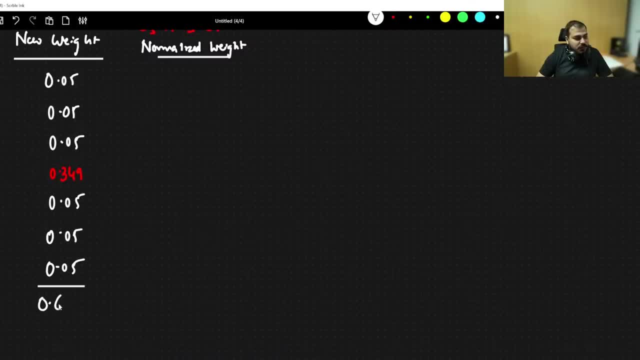 sum of all these things, sum of all these things, the summation of all these things, will the summation of all these things, will the summation of all these things will be point zero, point six, four, nine. all be point zero, point six, four, nine, all be point zero, point six, four, nine. all you have to do is that divide all the. 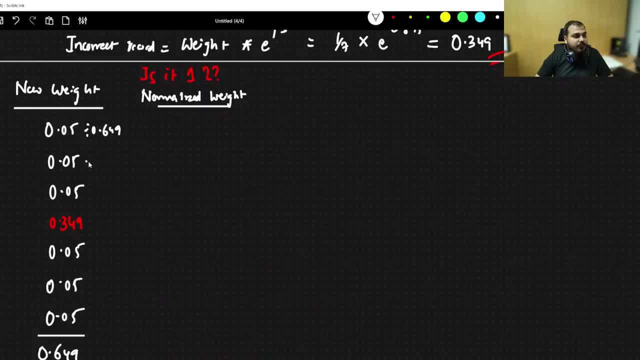 you have to do is that divide all the. you have to do is that divide all the numbers by numbers, by numbers by point six. four nine divided by point six. point six. four nine divided by point six. point six. four nine divided by point six, four nine, four nine. 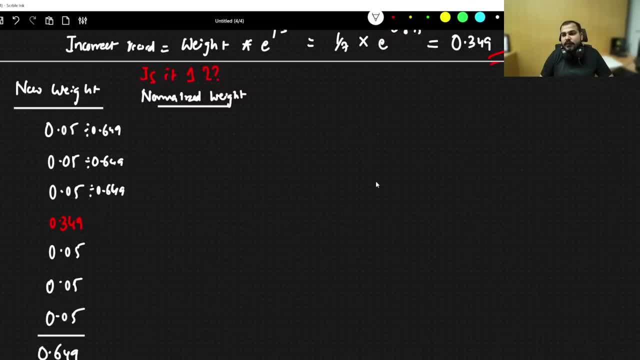 four, nine, point six, four, nine, point six, four, nine, point six, four, nine. like this: divide all the numbers by point. like this: divide all the numbers by point. like this: divide all the numbers by point six, four, nine, and tell me what will be. six, four, nine, and tell me what will be. 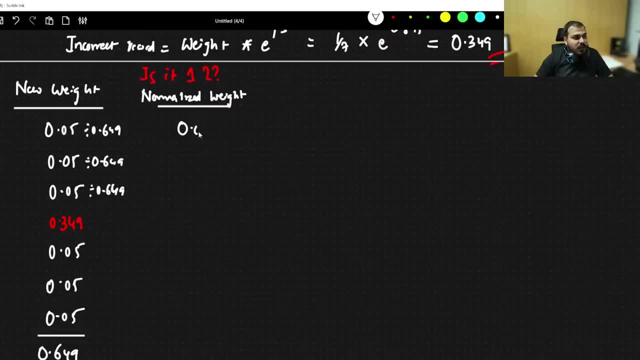 six, four, nine, and tell me what will be the answer that you will be getting. so, the answer that you will be getting so, the answer that you will be getting. so here: your normalized weight will now look here. your normalized weight will now look here. your normalized weight will now look like point zero seven, point zero seven. 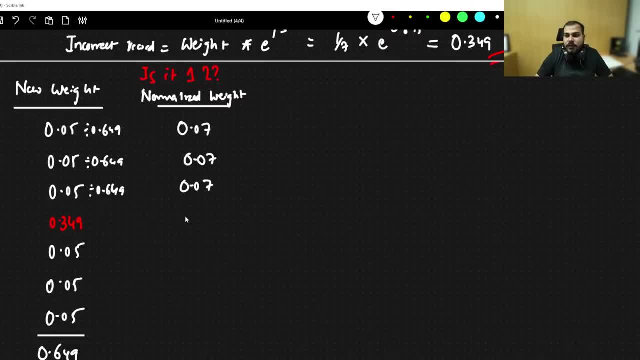 like point zero seven, point zero seven. like point zero seven, point zero seven, point zero seven, and this value will be point zero seven, and this value will be point zero seven, and this value will be somewhere around, uh, point five, three, seven. i guess in this. point five three seven, i guess in this. 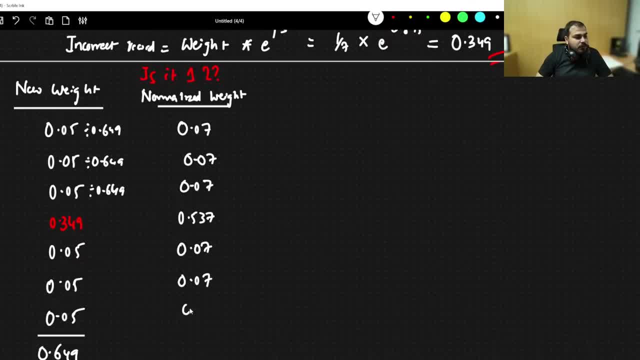 point five, three, seven, i guess. in this case, then this will be point zero seven case, then this will be point zero seven case, then this will be point zero seven, point zero seven, point zero, seven. okay, so point zero, seven, point zero, seven. okay, so, point zero, seven, point zero seven. okay. so this is basically a normalized weight. 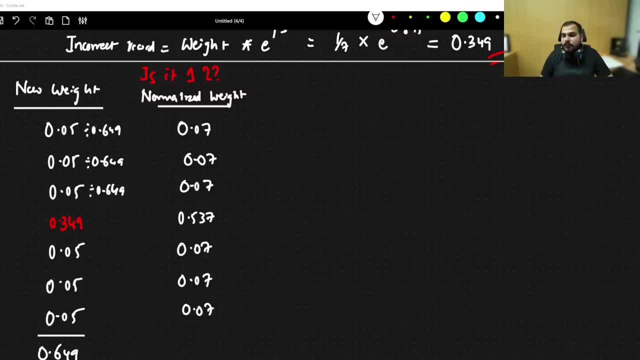 this is basically a normalized weight. this is basically a normalized weight. just let me know whether you're getting. just let me know whether you're getting. just let me know whether you're getting this thing or not. yes, i hope everybody is able to. yes, i hope everybody is able to. 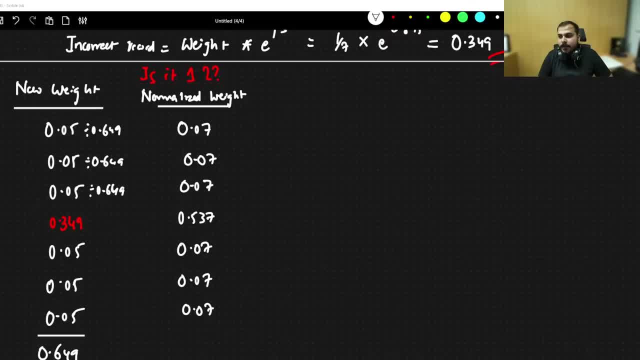 yes, i hope everybody is able to understand. yeah, here we are going to divide by all this. here we are going to divide by all this. here we are going to divide by all this: six, four point six, four, nine, okay. six, four point six, four, nine, okay. six, four point six, four, nine, okay now. this is my normalized weight now. 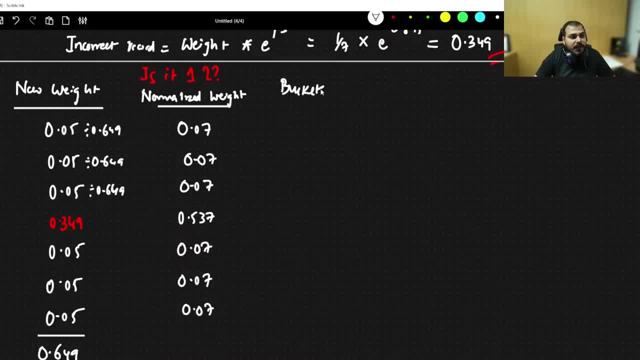 now, this is my normalized weight now. now, this is my normalized weight. now, after you get a normalized weight, we, after you get a normalized weight, we, after you get a normalized weight, we will try to create something called as, will try to create something called as, will try to create something called as buckets. 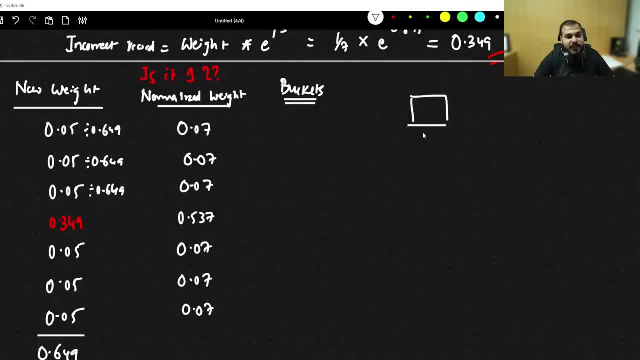 buckets, buckets, because see, because see, because see one decision tree. we have already created one decision tree. we have already created one decision tree. we have already created which is a stump right, which is a stump right, which is a stump right, which is a stump, and you know from this: 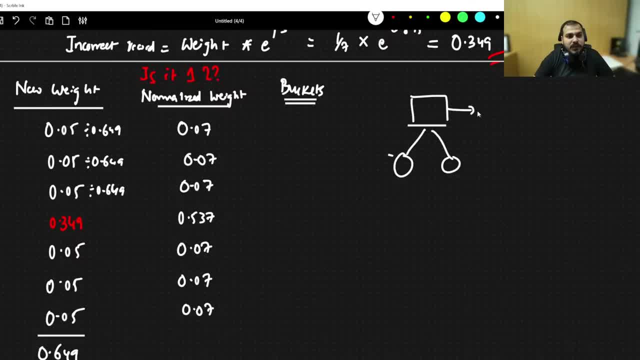 which is a stump and you know from this which is a stump and you know from this particular stump what you are going to particular stump. what you are going to particular stump, what you are going to get okay as an output, then in the. get okay as an output, then in the 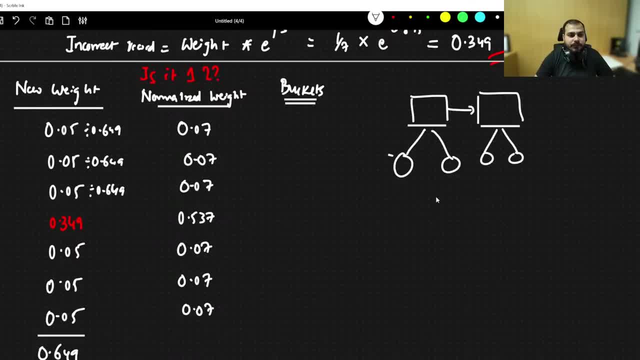 get okay as an output, then in the sequential model we will go and combine sequential model. we will go and combine sequential model. we will go and combine another model over here right now. it's another model over here right now. it's another model over here right now. it's because this model is giving one wrong. 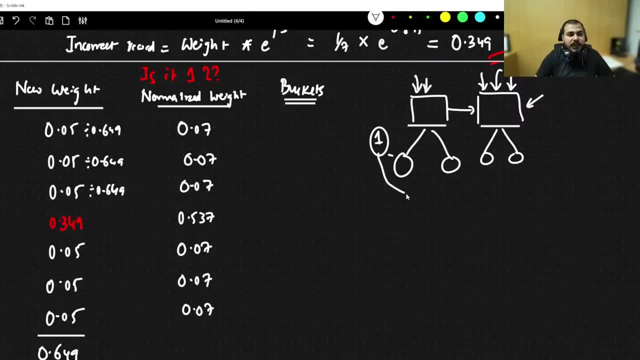 because this model is giving one wrong, because this model is giving one wrong now, what i have to do is that, whatever now. what i have to do is that, whatever. now. what i have to do is that whatever is wrong along with other data points, i is wrong along with other data points- i. 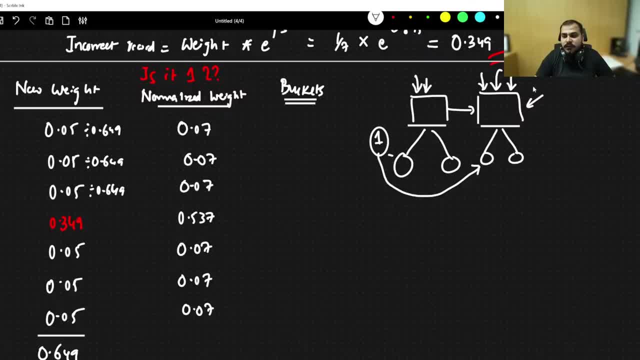 is wrong, along with other data points. i need to provide this specific model, with need to provide this specific model, with need to provide this specific model, with those records, those records, those records, so that this model will be able to train, so that this model will be able to train. 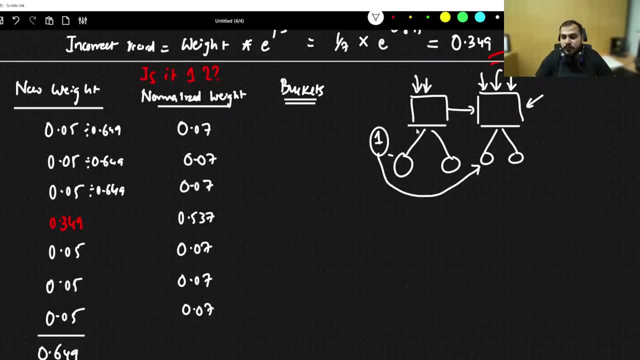 so that this model will be able to train on this and probably be able to get the on this and probably be able to get the on this and probably be able to get the output output output okay here, some is not uh, here, some is not uh. here, some is not uh. then, probably i have done the division. 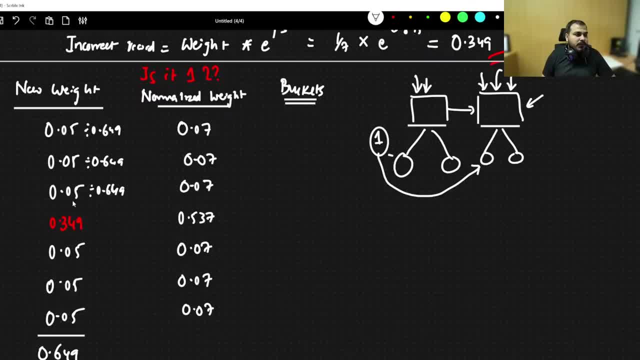 then probably i have done the division, then probably i have done the division wrong. let's see wrong. let's see wrong, let's see. point to one. one point five. two point to one, one point five. two point to one. one point five, two point two, five three. 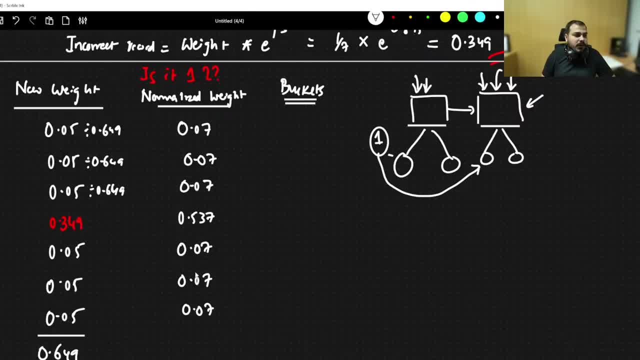 point two, five, three. point two, five, three, uh, 0.649. so let's see uh 0.649. so let's see uh 0.649. so let's see one, two, three, four, five, six. let me open the. it will be, it will be. 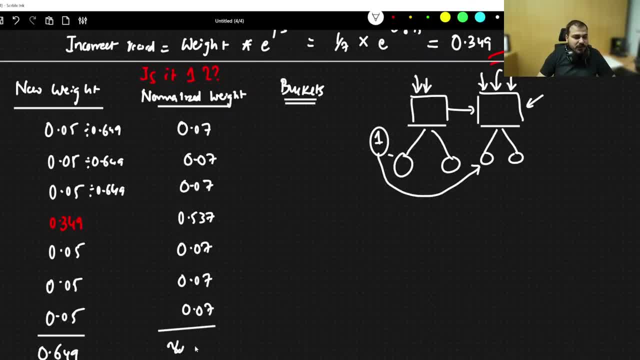 let me open the. it will be. it will be. let me open the. it will be. it will be approximately equal to guys one. approximately equal to guys one. approximately equal to guys one. this will be approximately equal to one. this will be approximately equal to one. this will be approximately equal to one, don't worry. 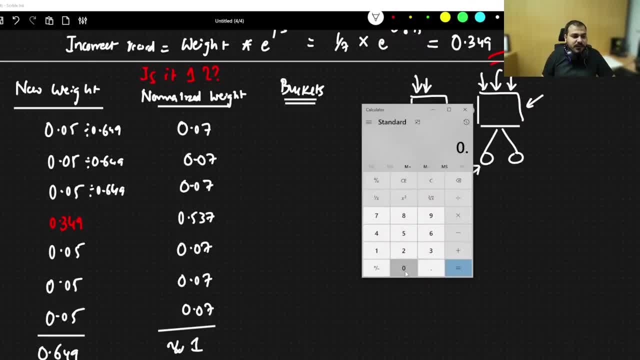 don't worry, don't worry, i am. i'm missing some decimals, otherwise i am. i'm missing some decimals, otherwise i am. i'm missing some decimals, otherwise it will become one. only see, it will become one. only see, it will become one. only see point zero five divided by 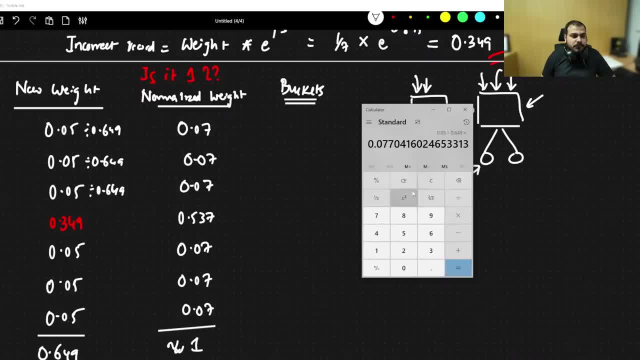 point zero, five divided by point zero, five divided by point six four, nine. point six four, nine. point six four, nine. it is point seven, seven. it is point seven, seven. it is point seven, seven. point zero, seven, seven. okay, so if i take point zero seven, seven, okay, so if i take. 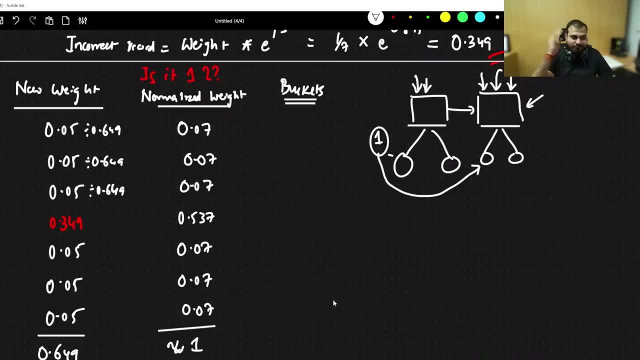 point zero, seven, seven, okay. so if i take seven, seven, seven, seven, seven, seven, come on, guys. common sense, okay. come on, guys. common sense, okay. come on, guys, common sense, okay, common sense, common sense, common sense, now, now, now. let's create buckets now based on. let's create buckets now based on. 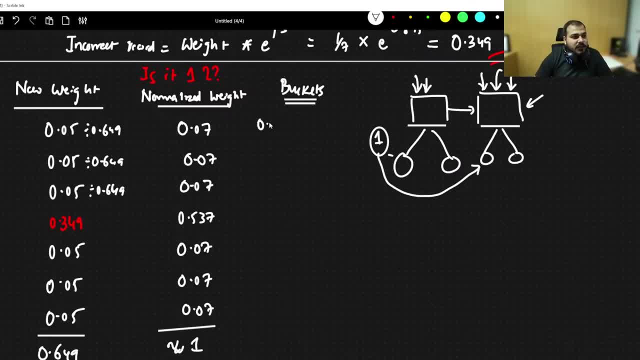 let's create buckets now, based on buckets. how the buckets will be created. buckets. how the buckets will be created. buckets how the buckets will be created over here. i will take 0.07 over here. i will take 0.07 over here. i will take 0.07 until sorry, whatever is the. 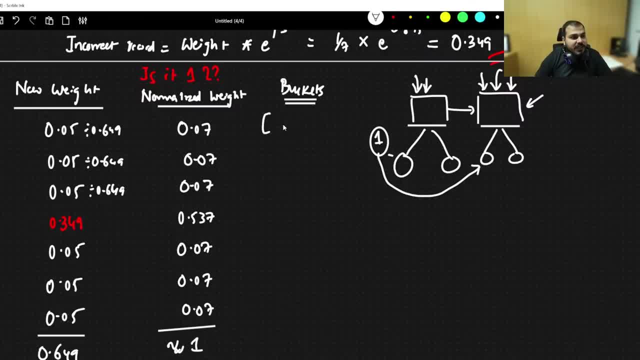 until sorry. whatever is the until sorry, whatever is the value over here- normal weight value- okay. value over here- normal weight value- okay. value over here- normal weight value- okay. so i will start creating my buckets, so i will start creating my buckets, so i will start creating my buckets. buckets, basically, from 0 to 0.07. 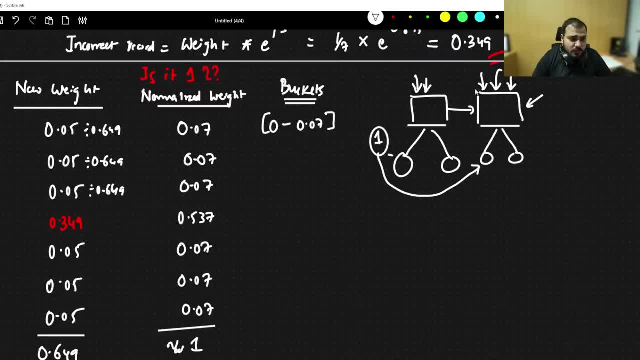 buckets, basically from 0 to 0.07 buckets, basically from 0 to 0.07. okay, see what did i say now. okay, see what did i say now. okay, see what did i say now. for this decision, tree or stump i need. for this decision, tree or stump i need. 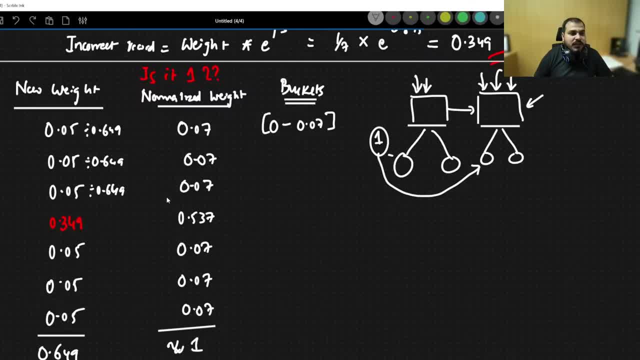 for this decision, tree or stump, i need to provide some records. to provide some records, to provide some records now. how do we decide that? okay, there now. how do we decide that? okay, there now. how do we decide that? okay, there should be a way that we should be able. 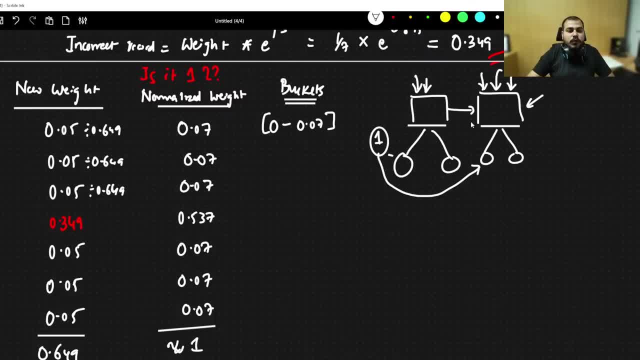 should be a way that we should be able, should be a way that we should be able to say that that specific wrong number, to say that that specific wrong number, to say that that specific wrong number of records should go to that decision of records should go to that decision. 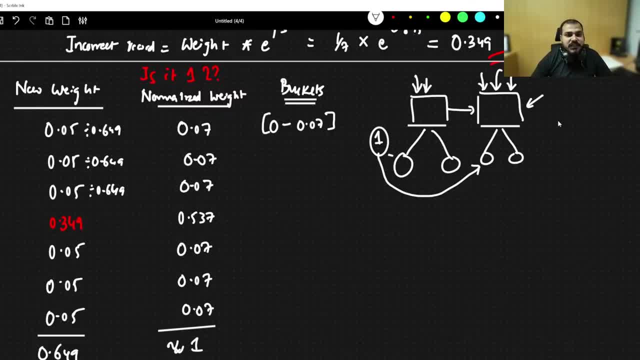 of records should go to that decision tree. so for that purpose, what we do is tree. so for that purpose, what we do is tree. so for that purpose, what we do is that this decision tree will randomly that this decision tree will randomly that this decision tree will randomly create some numbers. 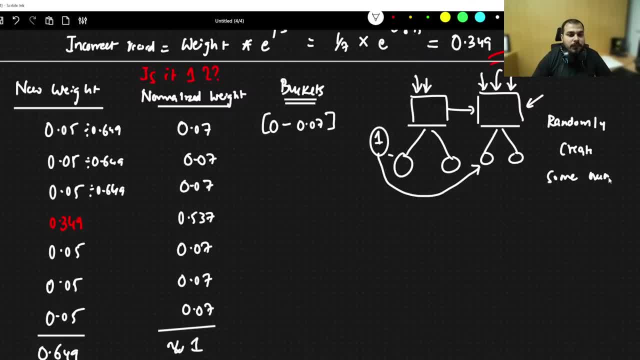 create some numbers. create some numbers randomly. create some numbers randomly create some numbers randomly. create some numbers, some numbers between, some numbers, between some numbers between zero to one, zero to one, zero to one. okay, randomly create those numbers between. okay, randomly create those numbers between. okay, randomly create those numbers between zero to one, and whichever bucket it will. 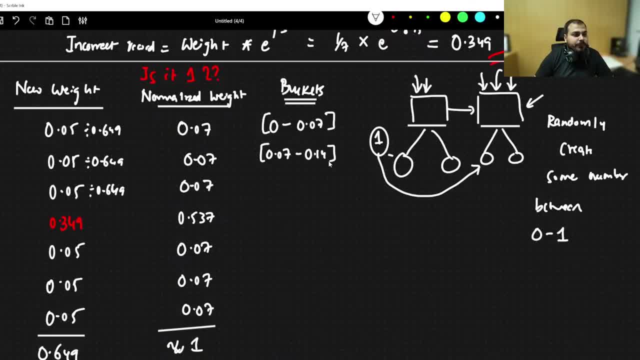 zero to one and whichever bucket it will zero to one and whichever bucket it will come in like zero seven to zero one four. come in like zero seven to zero one four. come in like zero seven to zero one four. okay, zero one four two zero seven. okay, zero one four two zero seven. 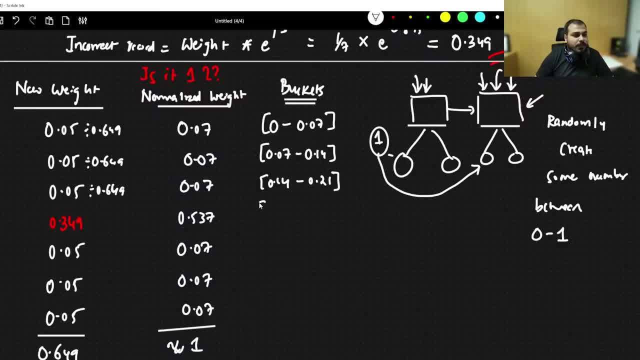 okay, zero one four two. zero seven basically means zero, basically means zero. basically means zero two one. okay, then zero two one two one. okay, then zero two one two one. okay, then zero two one, two. see how the bucket is getting created. two: see how the bucket is getting created. 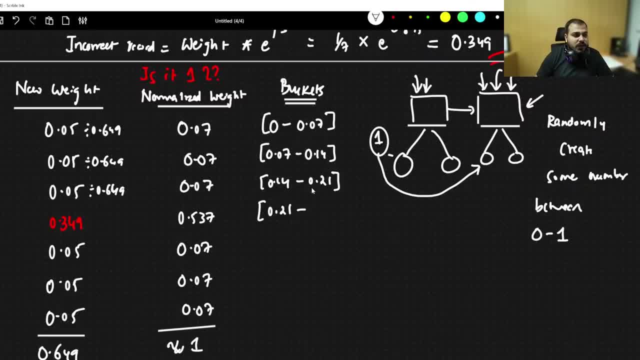 two. see how the bucket is getting created. this value is getting added to this. so this value is getting added to this. so this value is getting added to this. so that becomes this bucket. okay, zero two. that becomes this bucket. okay, zero two. that becomes this bucket. okay, zero two one plus point three. five, three, seven. 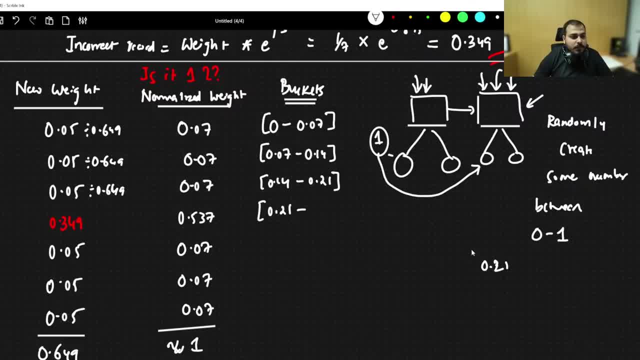 one plus point three, five, three, seven. one plus point three, five, three, seven. how much it is, how much it is, how much it is? zero, two, one, zero two. one zero two, one point five, three, seven, point five, three, seven, point five, three, seven. it is nothing but four, seven, zero. 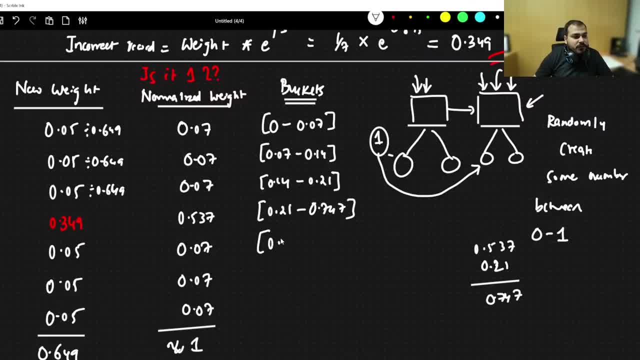 it is nothing but four, seven, zero. it is nothing but four, seven, zero. point seven, four, seven. okay, then, point point seven, four, seven. okay, then point point seven, four, seven. okay, then, point seven, four, seven, seven, four, seven, seven, four, seven, two, two, two, point seven, five, one. 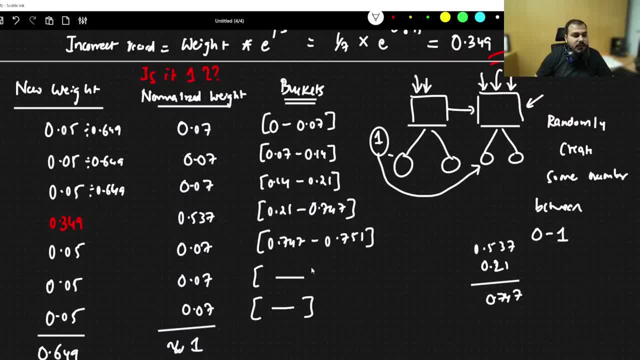 point seven five one. point seven five one. like this: you create all the buckets. okay, like this, you create all the buckets. okay, like this, you create all the buckets. okay, you can create all the buckets. now tell me you can create all the buckets. now tell me you can create all the buckets. now tell me which record is basically having the biggest? 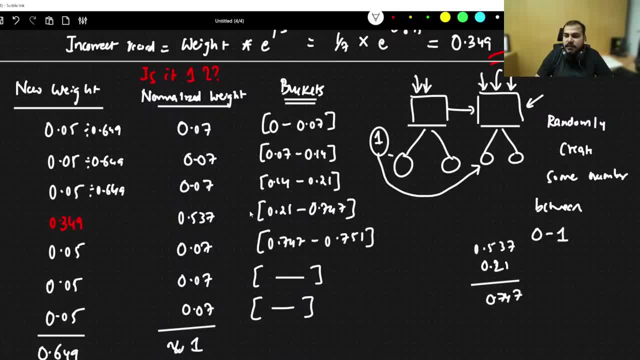 which record is basically having the biggest? which record is basically having the biggest bucket size? which record is having the biggest? which record is having the biggest? which record is having the biggest bucket size? obviously this record bucket size. obviously this record bucket size. obviously this record. so if i randomly create a number between 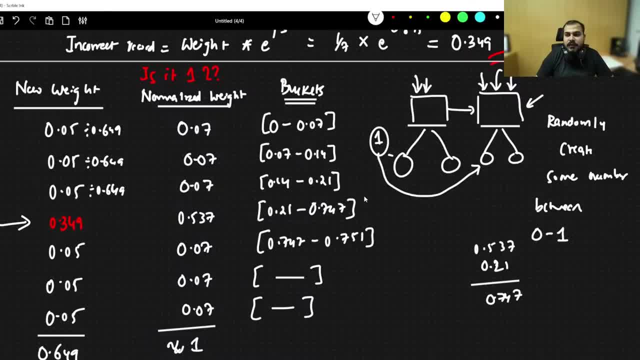 so if i randomly create a number between, so if i randomly create a number between zero to one, zero to one, zero to one, what is the highest probability that the? what is the highest probability that the? what is the highest probability that the values will be going in? 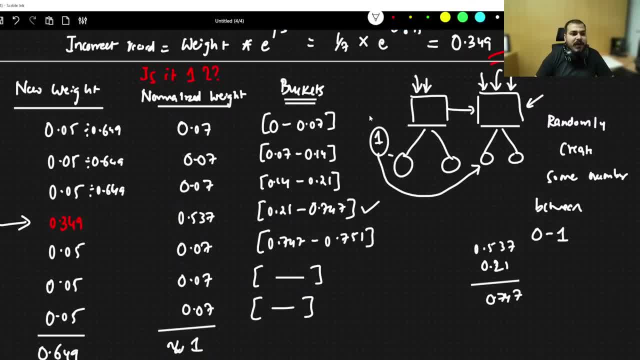 okay. so in this particular case, most of okay. so in this particular case, most of okay. so in this particular case, most of the wrong records will be passed along. the wrong records will be passed along. the wrong records will be passed along with the other records, obviously other. 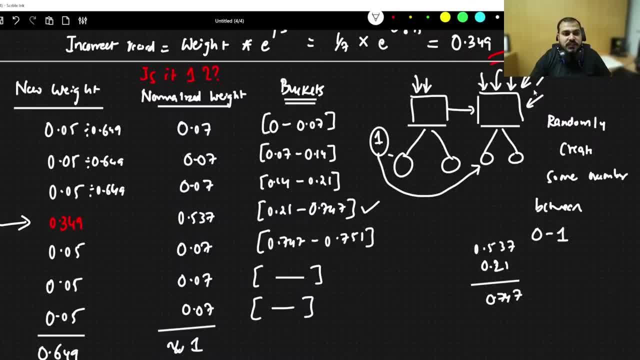 with the other records, obviously other. with the other records, obviously other records. there are chances that other records. there are chances that other records. there are chances that other records will go to the next decision tree records will go to the next decision tree records will go to the next decision tree but understand maximum number will go. 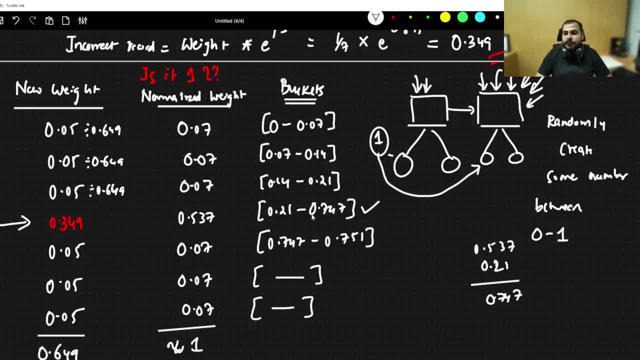 but understand maximum number will go, but understand maximum number will go. with the wrong records because the with the wrong records because the with the wrong records because the bucket is high over here. bucket is high over here, bucket is high over here, right, right, right. so the bucket is high over here, so most 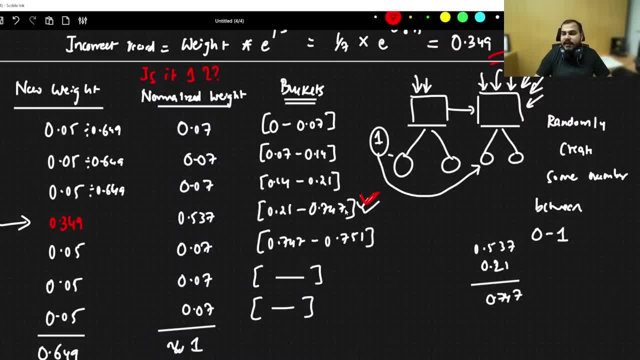 so the bucket is high over here. so, most so, the bucket is high over here. so, most of the time, this specific record will of the time, this specific record will of the time, this specific record will get created, selected, get created, selected, get created, selected, and then it will be gone to the second. 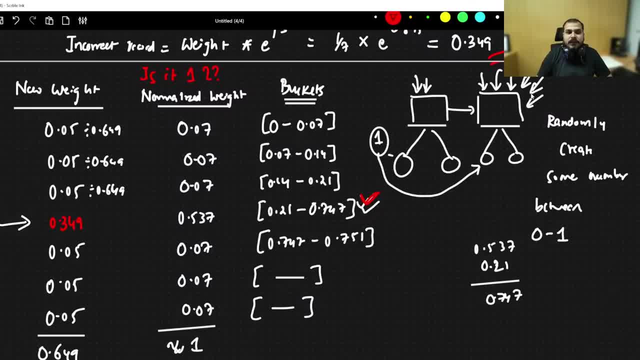 and then it will be gone to the second, and then it will be gone to the second tree. i hope everybody is able to tree. i hope everybody is able to tree. i hope everybody is able to understand right, understand right, understand right. so this is how this entire things will. 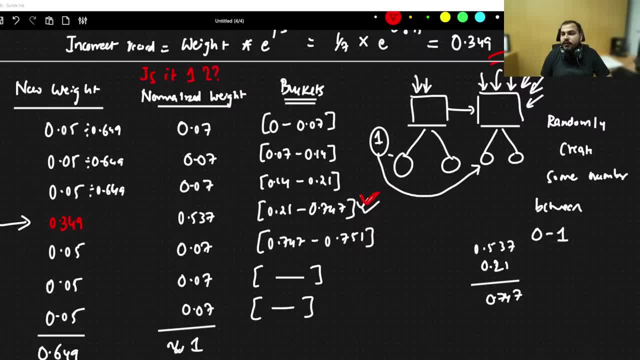 so this is how this entire things will, so this is how this entire things will be going on. guys, be going on, guys, be going on, guys. then again, you will probably go ahead, then again, you will probably go ahead, then again, you will probably go ahead and calculate again. you will do all. 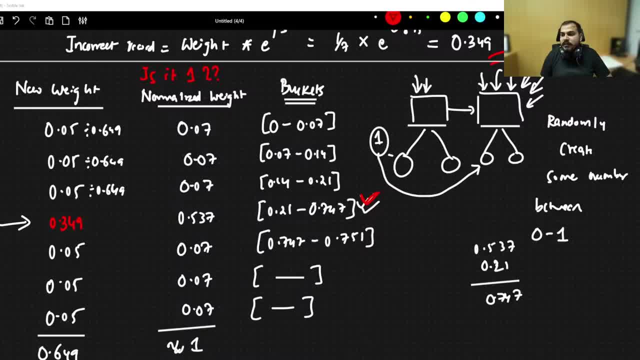 and calculate again. you will do all and calculate again. you will do all those things. did you get an idea till here or not? did you get an idea till here or not? did you get an idea till here or not? guys, right, right, right now, see what is happening. 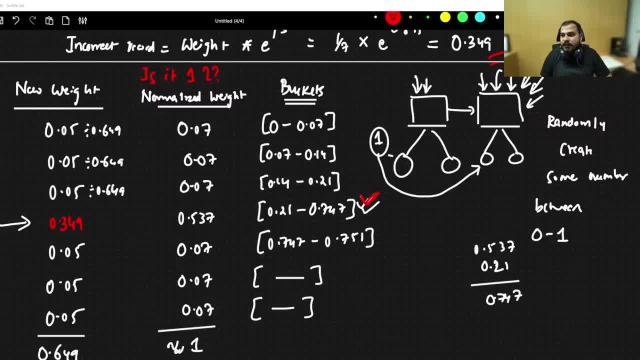 now. see what is happening now. see what is happening. i will draw this till here, did you? i will draw this till here, did you? i will draw this till here. did you? see what exactly will happen now? see what exactly will happen now. see what exactly will happen now. now, suppose i have this all records. 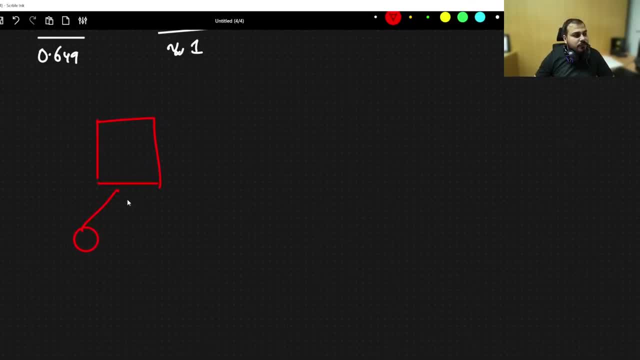 now suppose i have this all records. now suppose i have this all records. okay, okay, okay. so this is my first stump. so this is my first stump. so this is my first stump. this is my second stump. this is my second stump. this is my second stump. this is my third stump, similarly the third. 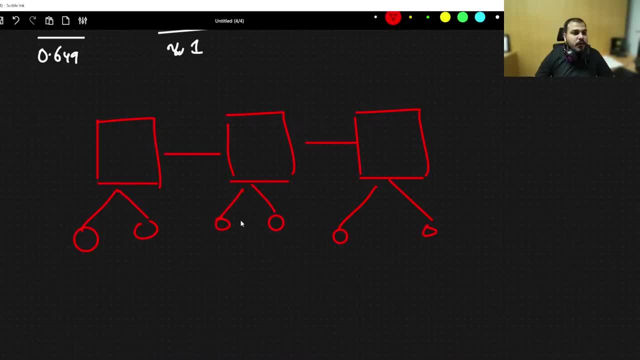 this is my third stump, similarly the third. this is my third stump, similarly the third stump from the second stump. whichever stump from the second stump, whichever stump from the second stump, whichever wrong records will be going, maximum wrong records will be going. maximum wrong records will be going. maximum number of records will go over here. 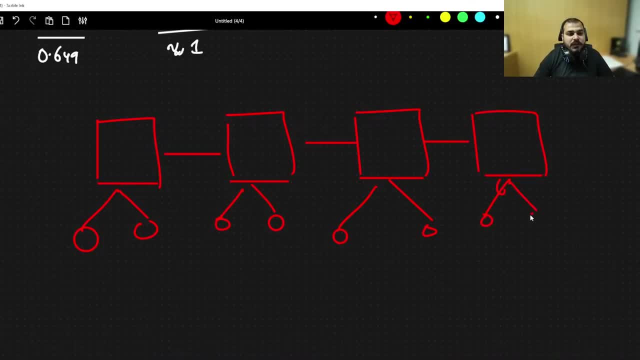 number of records will go over here. number of records will go over here. then again, it will be trained like this. then again, it will be trained like this. then again, it will be trained like this: will be having lot of stumps minimum. will be having lot of stumps minimum. 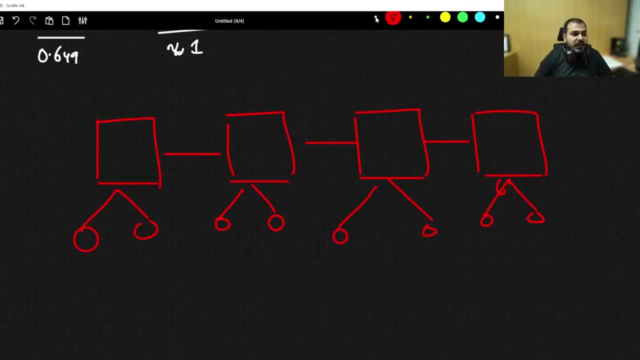 will be having lot of stumps. minimum hundred decision trees can be added. okay, hundred decision trees can be added. okay, hundred decision trees can be added. okay, you know that. every decision tree. will you know that every decision tree, will you know that every decision tree will give one output for a new test data? 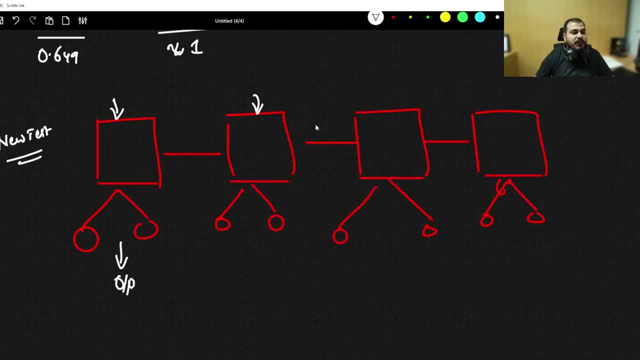 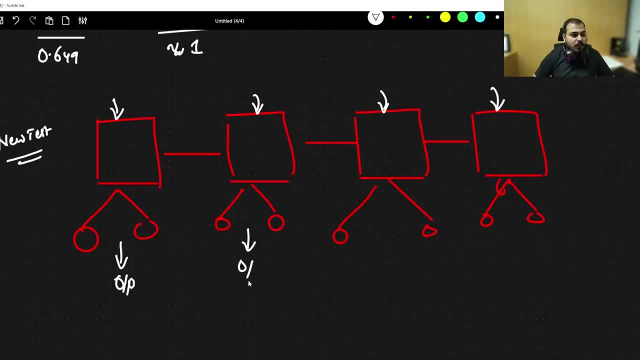 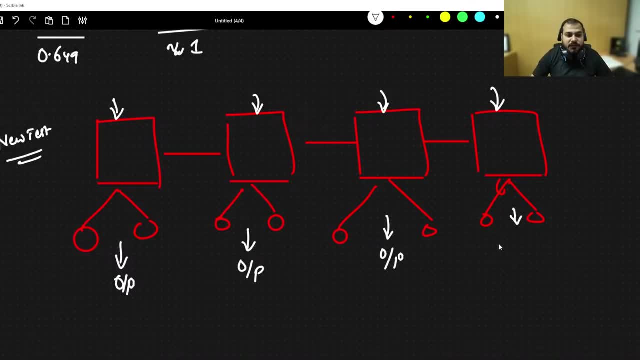 output. okay, okay, okay, obviously, at a time, complexity will be. obviously at a time complexity will be. obviously at a time complexity will be more, more, more now from this particular output, suppose now from this particular output. suppose now from this particular output, suppose it is a binary classification, i will be. 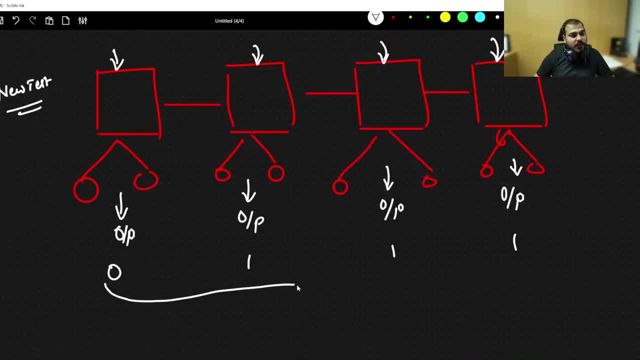 it is a binary classification. i will be. it is a binary classification. i will be. getting zero one one one. so again over. getting zero one one one, so again over. getting zero one one one. so again over here majority voting will happen and the here majority voting will happen. and the 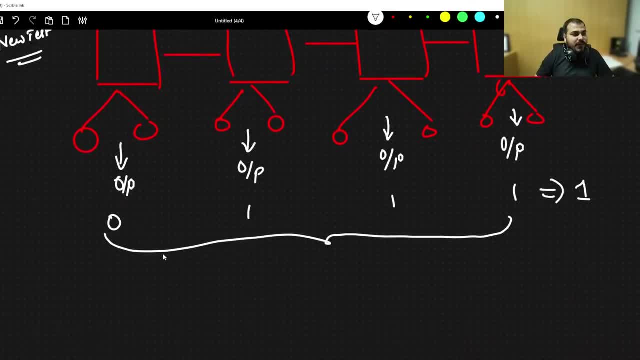 here, majority voting will happen and the output will be one. output will be one. output will be one. in case of regression problem: i will be in case of regression problem. i will be in case of regression problem. i will be having a continuous value over here. having a continuous value over here. 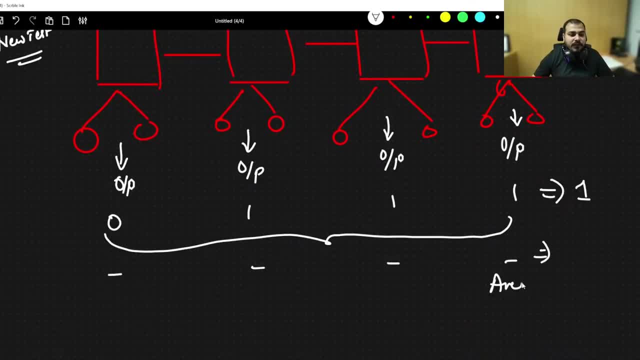 having a continuous value over here. okay, and for this, the average. okay, and for this the average- okay, and for this the average average will be computed. average will be computed, average will be computed and that will give me an output over here and that will give me an output over here. 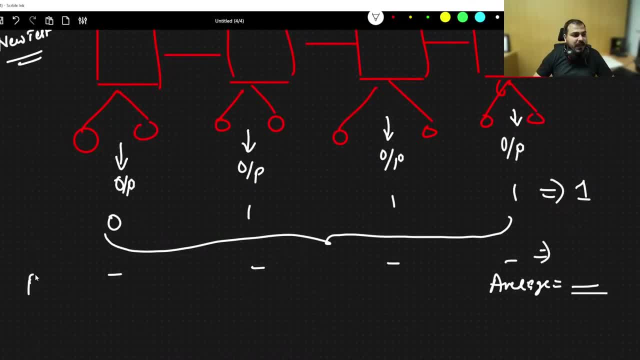 and that will give me an output over here. okay, okay, okay. so for regression, the average will be. so for regression, the average will be. so for regression, the average will be done, done, done for classification. what will happen for classification? what will happen for classification? what will happen? majority will be happening. so every way. 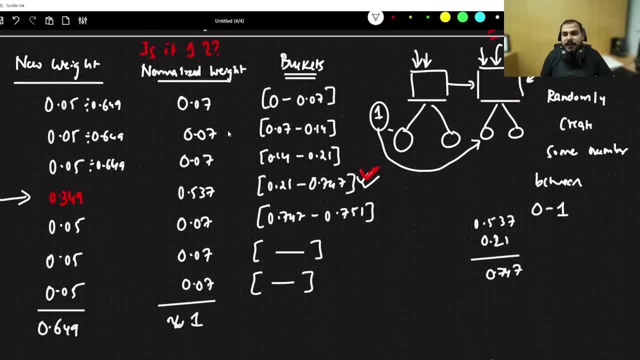 majority will be happening. so, every way, majority will be happening. so, every way, that same part will be going on. okay, that same part will be going on. okay, that same part will be going on. okay, buckets is very much simple, guys, buckets. buckets is very much simple, guys, buckets. 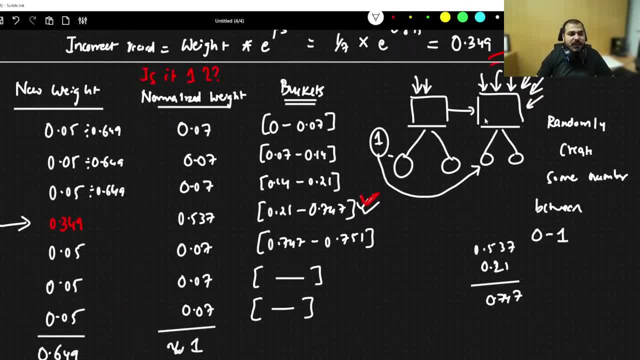 buckets is very much simple, guys. buckets basically means based on this, weights basically means based on this, weights basically means based on this, weights, normalized weight. we are going to normalized weight. we are going to normalized weight. we are going to create bucket so that whichever records, create bucket so that whichever records, 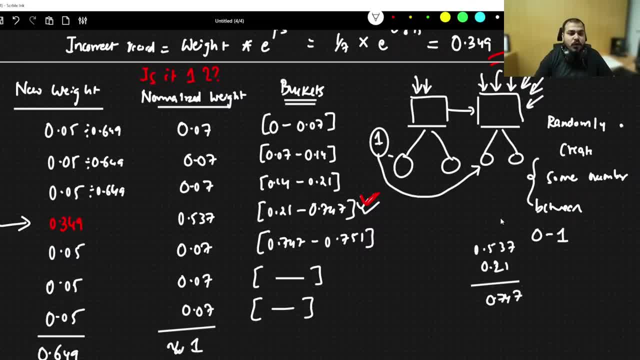 create bucket so that whichever records has the highest bucket based on this, has the highest bucket based on this, has the highest bucket based on this, randomly creating code. you know it will randomly creating code. you know it will randomly creating code. you know it will select those specific buckets and put it. 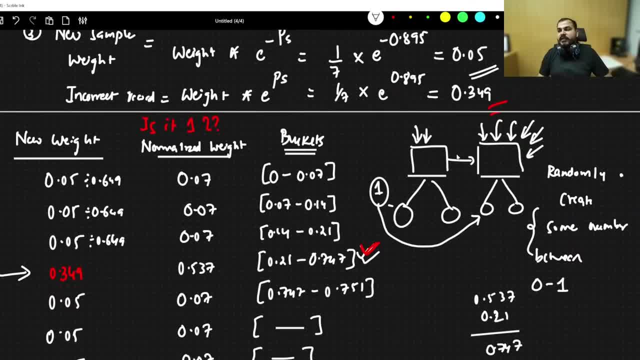 select those specific buckets and put it. select those specific buckets and put it into random forest, into random forest, into random forest. okay, the next decision tree. sir, we understand why this bucket size is. we understand why this bucket size is. we understand why this bucket size is big. 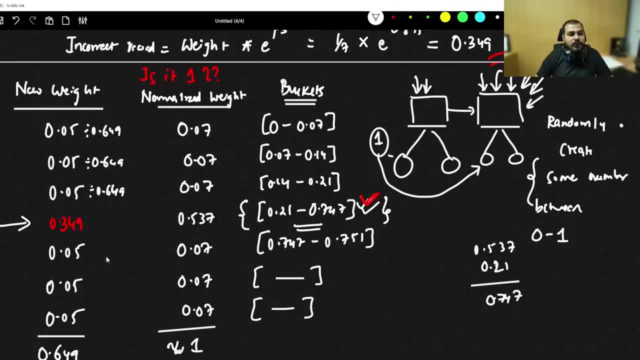 big, big the other wrong records. which are the other wrong records, which are the other wrong records which are present. right suppose they are more than present. right suppose they are more than present. right suppose they are more than four to five wrong records, their bucket. four to five wrong records, their bucket. 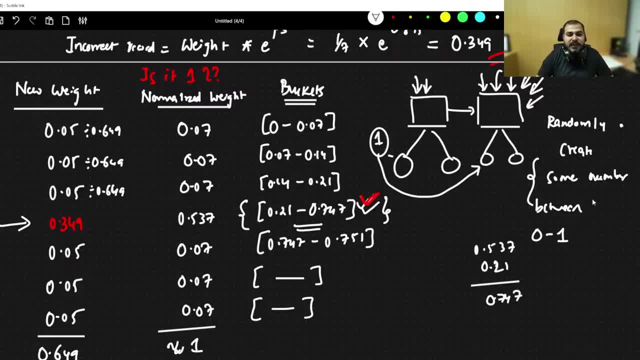 four to five wrong records, their bucket size will also be bigger. size will also be bigger. size will also be bigger. and because, based on this, randomly, and because, based on this randomly, and because, based on this, randomly, creating number between zero to one, creating number between zero to one, 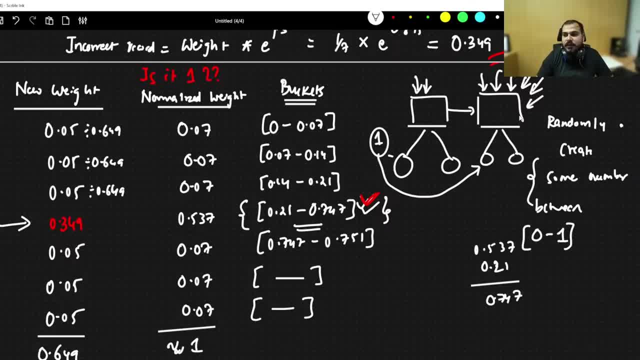 creating number between zero to one. most of the wrong records will be selected. most of the wrong records will be selected. most of the wrong records will be selected and given to the second stone and given to the second stone and given to the second stone. similarly, this particular decision tree. 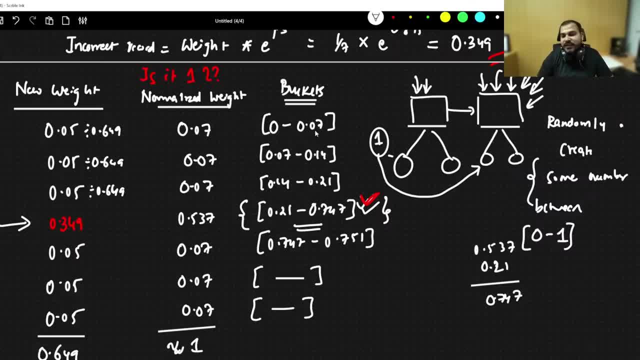 similarly, this particular decision tree, similarly, this particular decision tree will be doing some mistakes, then that will be doing some mistakes, then that will be doing some mistakes, then that wrong records will get updated, all the wrong records will get updated. all the wrong records will get updated, all the weights will get updated and it will be 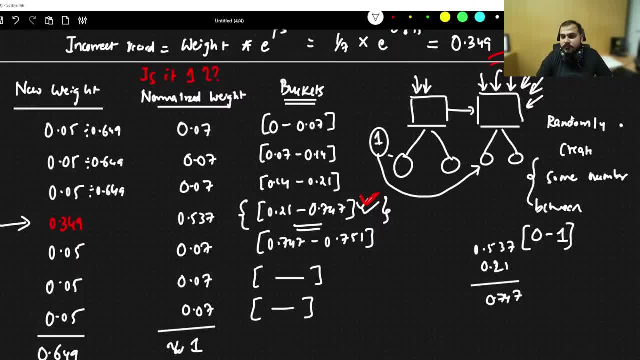 weights will get updated, and it will be. weights will get updated and it will be passed to the next decision tree. okay, guys, when i say wrong, record the output. guys. when i say wrong, record the output. guys, when i say wrong, record the output, will be same. only you know. 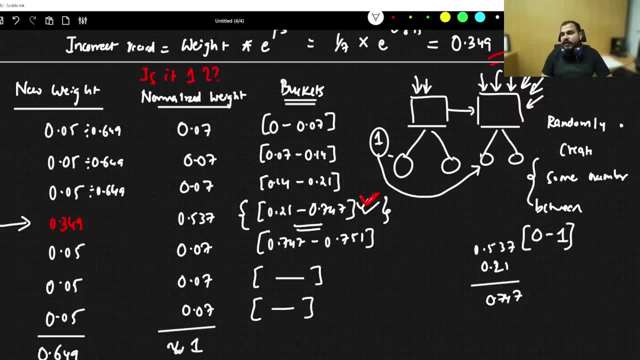 will be same. only you know will be same, only you know zero and one okay, zero and one okay, zero and one okay. so interesting everyone. i hope you so interesting everyone. i hope you so interesting everyone. i hope you understood so much of maths in ada boost. understood so much of maths in ada boost. 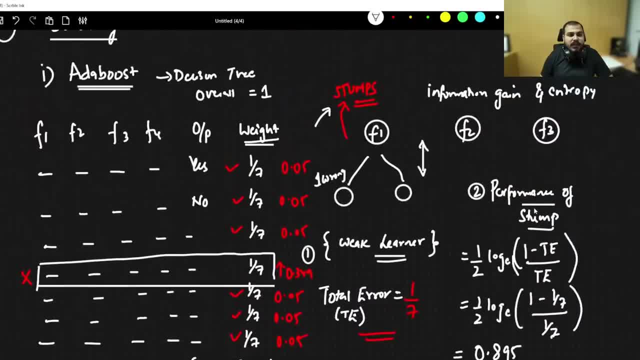 understood so much of maths in ada boost and how ada boost actually work. three and how ada boost actually work. three and how ada boost actually work. three main things: one is total error, one is main things, one is total error. one is main things, one is total error. one is performance of stump and one is the new. 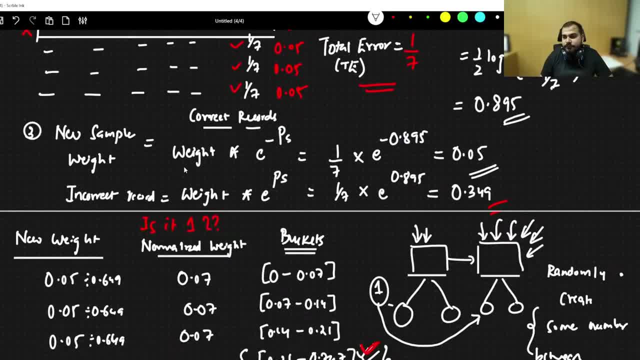 performance of stump, and one is the new performance of stump and one is the new sample weight. these things are getting sample weight. these things are getting sample weight. these things are getting calculated extensively, calculated, extensively, calculated, extensively. everybody clear, i hope you like this. everybody clear, i hope you like this. 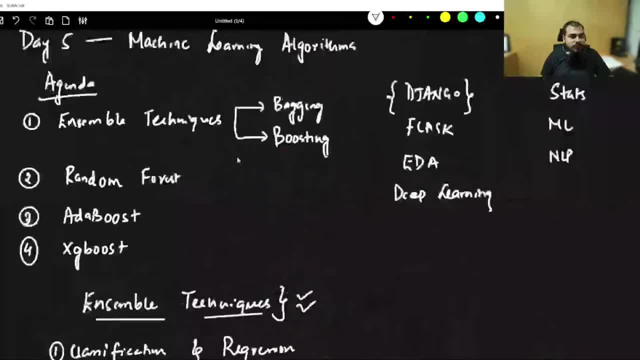 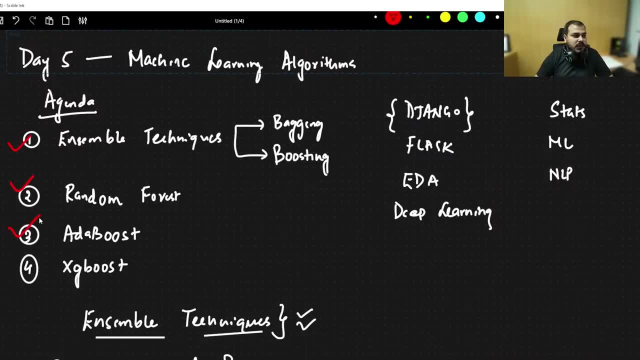 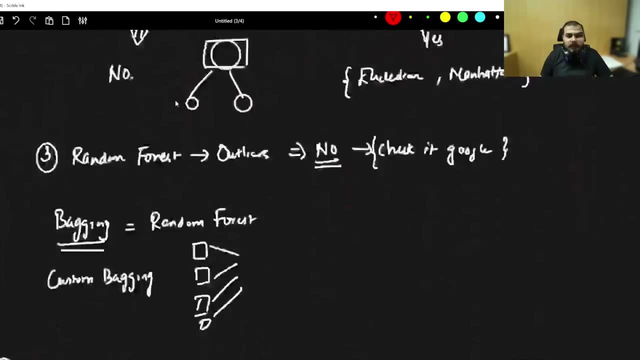 everybody clear. i hope you like this session. session, session till here, till here, till here. so we completed, so we completed. so we completed this. this and this: max normalized weight was basically used. max normalized weight was basically used. max normalized weight was basically used because the sum of all these weights 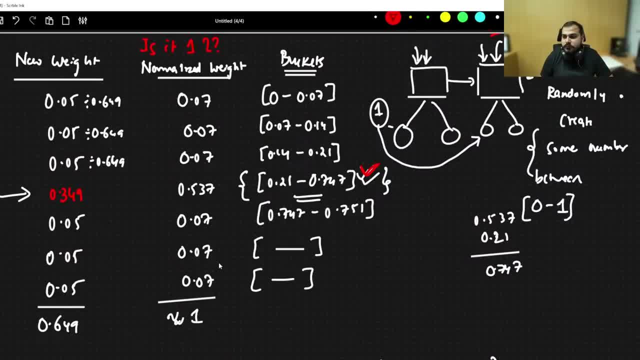 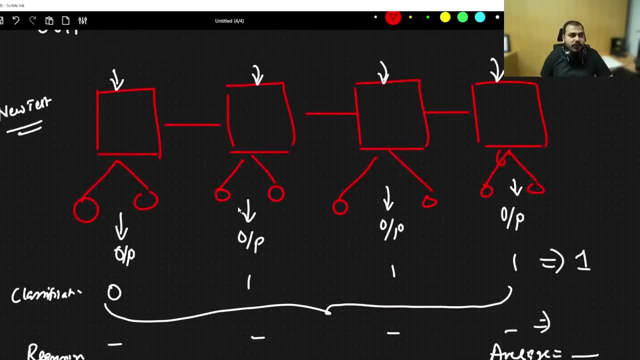 because the sum of all these weights- because the sum of all these weights are are- are approximately equal to one when boosting. why not take the last when boosting? why not take the last when boosting? why not take the last output? no, no, no output, no, no, no output, no, no, no. we have to give the importance of every. 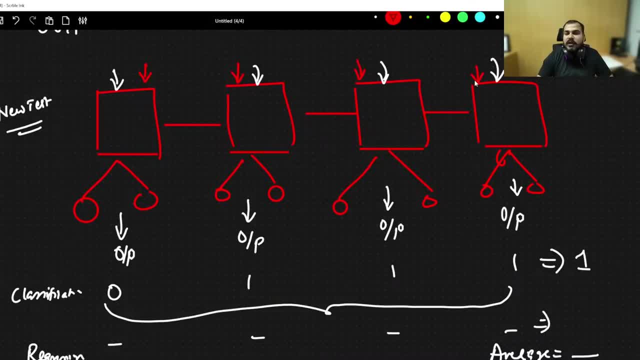 we have to give the importance of every. we have to give the importance of every decision tree output. decision tree output, decision tree output, every decision tree output are important, okay, okay, okay. yes, guys, you may have some doubts, revise. yes, guys, you may have some doubts, revise. yes, guys, you may have some doubts, revise. i have added everything what is possible. 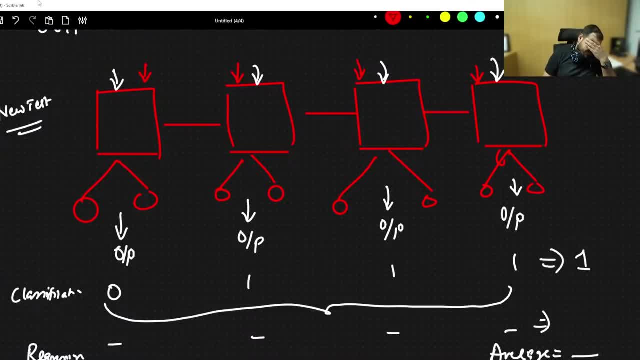 i have added everything. what is possible? i have added everything. what is possible inside this, inside this, inside this? okay, i know, nothing is simple, you know, i know nothing is simple. you know, i know nothing is simple, you know. okay, let me talk about one model, which. okay, let me talk about one model which. 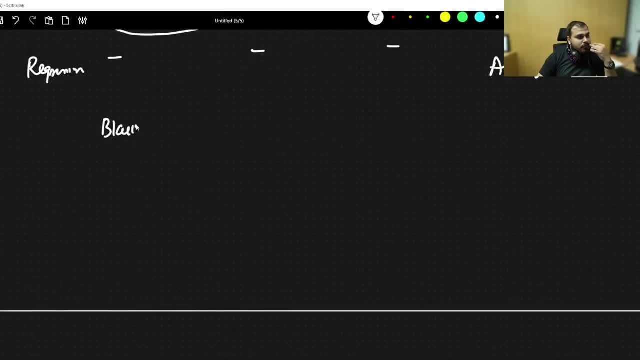 okay, let me talk about one model, which is called as is called, as is called as black box model versus white box. what is the difference between black box? what is the difference between black box? what is the difference between black box model and white box? if i take an example of linear regression, 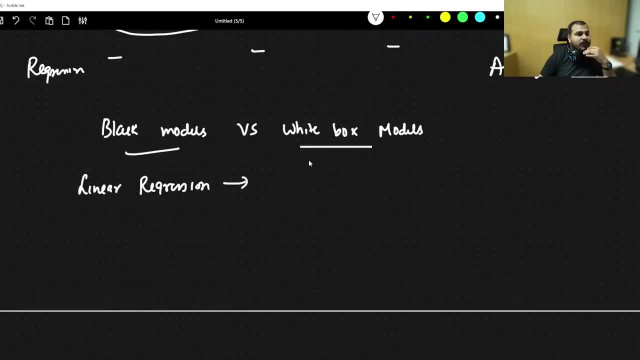 tell me what kind of model it is. is it a? tell me what kind of model it is. is it a? tell me what kind of model it is. is it a white box model or black box? white box model or black box, white box model or black box? if i take an example of random forest, 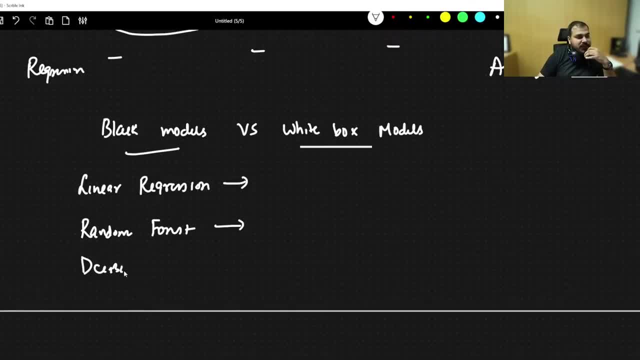 if i take an example of random forest. if i take an example of random forest, is this a white box or black box? if i, is this a white box or black box? if i, is this a white box or black box? if i take an example of decision tree: 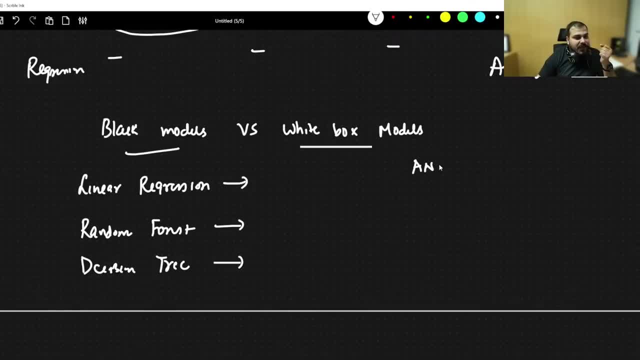 it is a white box or black box model. it is a white box or black box model. it is a white box or black box model. if i take an example of a and n, if i take an example of a and n. if i take an example of a and n, is it a white box or black box model? 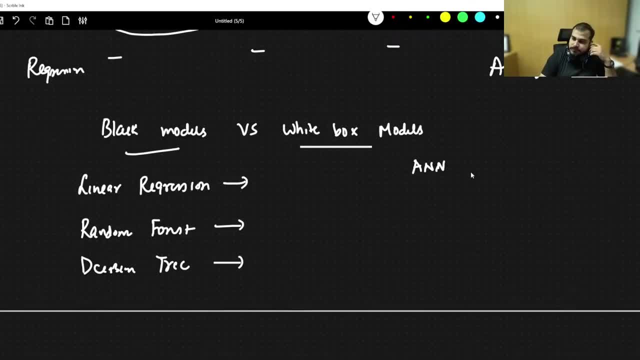 is it a white box or black box model? is it a white box or black box model? tell me guys, this is an interview. tell me guys, this is an interview. tell me guys, this is an interview question and why probably it is called as a black and why probably it is called as a black. 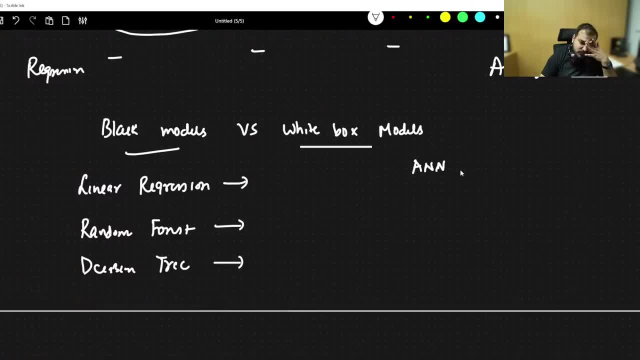 and why probably it is called as a black box model, black box or white box. okay, let me say okay, let me say okay, let me say linear regression is basically called as. linear regression is basically called as. linear regression is basically called as a wide, a wide, a wide box model, because here you can. 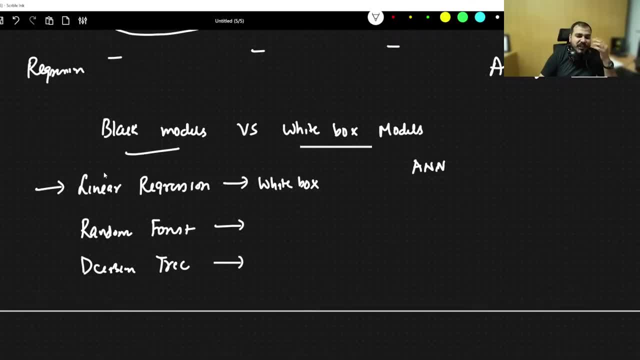 box model, because here you can box model, because here you can basically visualize, basically visualize, basically visualize how the theta value is basically changing, how the theta value is basically changing, how the theta value is basically changing and how it is coming to a global minima and how it is coming to a global minima. 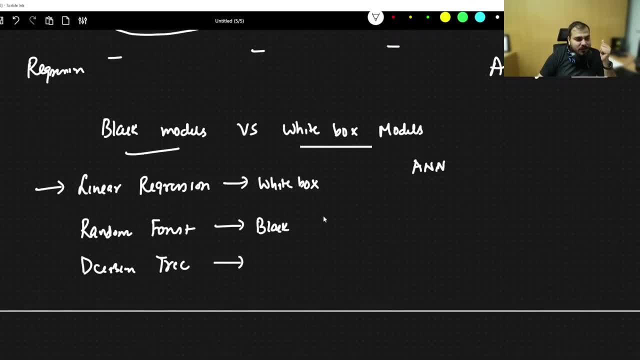 and how it is coming to a global minima and all those things and all those things and all those things. in random forest, i will say this as in random forest. i will say this as in random forest. i will say this as black box model, because it is impossible. 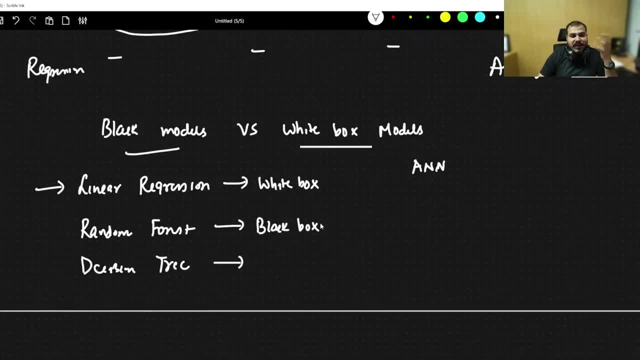 black box model, because it is impossible. black box model, because it is impossible to see all the decision tree, to see all the decision tree, to see all the decision tree how it is working. so that is the reason how it is working. so that is the reason how it is working. so that is the reason the maths is so complex inside us. 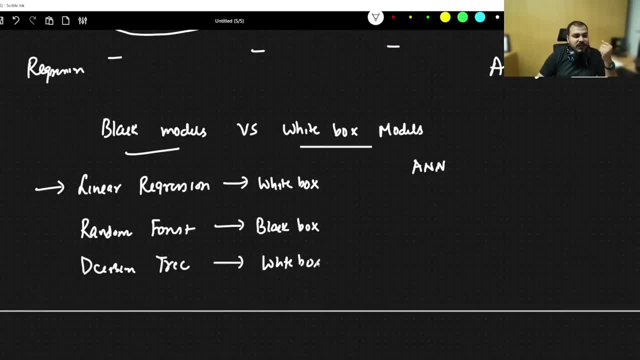 the maths is so complex inside us. the maths is so complex inside us if i talk about decision tree. this is if i talk about decision tree. this is if i talk about decision tree. this is basically a white box model, because in basically a white box model, because in 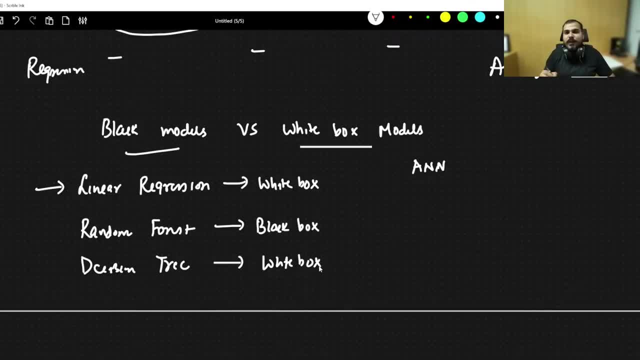 basically a white box model, because in decision tree, we know decision tree, we know decision tree, we know how the split are basically happening, how the split are basically happening, how the split are basically happening. with the help of paper and pen you will. with the help of paper and pen, you will. 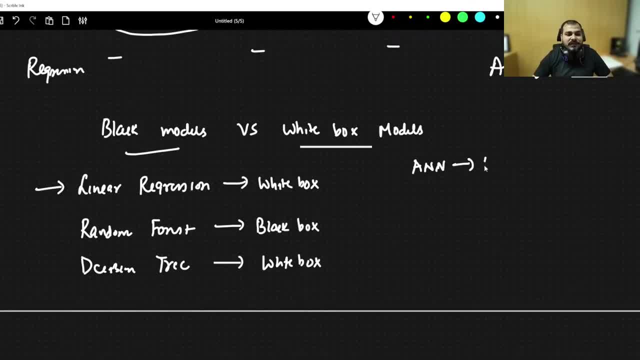 with the help of paper and pen, you will be able to do it. be able to do it. be able to do it in the case of a and n. this is a black in the case of a and n. this is a black. in the case of a and n. this is a black box model, because here you don't know. 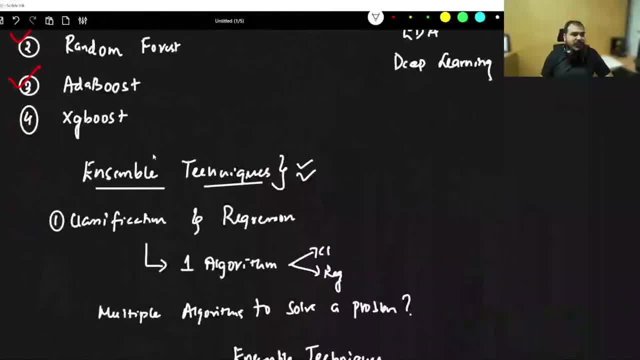 box model, because here you don't know. box model, because here you don't know. one more topic is left with respect to xg. one more topic is left with respect to xg. one more topic is left with respect to xg: boost, regression, boost, regression, boost, regression and classification. i'm having a bit of 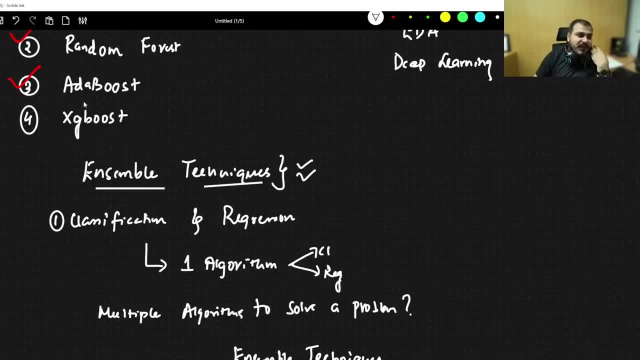 and classification. i'm having a bit of and classification. i'm having a bit of headache, so i'm closing the session now. headache, so i'm closing the session now. headache, so i'm closing the session now. but you can definitely check this out as. but you can definitely check this out as. 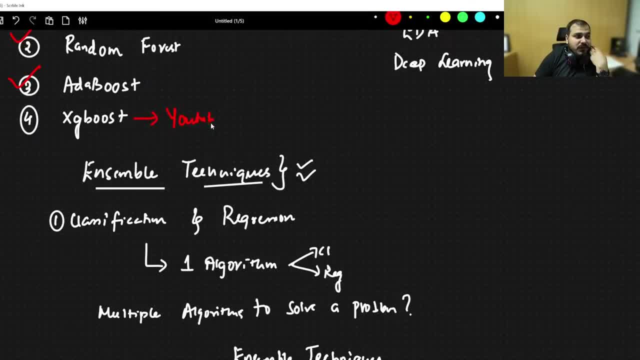 but you can definitely check this out as an assignment from my youtube channel, an assignment from my youtube channel, an assignment from my youtube channel. guys, guys, guys. okay. so from my youtube channel. i have okay. so from my youtube channel, i have okay. so from my youtube channel. i have already discussed about this in depth. 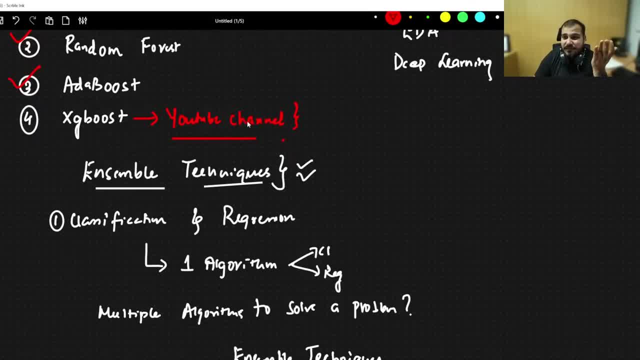 already discussed about this in depth. already discussed about this in depth. so please have a look otherwise. if i my so, please have a look otherwise. if i my so please have a look otherwise. if i my headache i if i was not having headache i headache i if i was not having headache i. 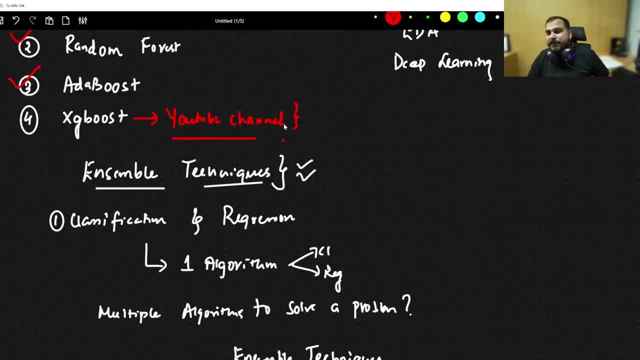 headache. i, if i was not having headache, i could have completed over here, could have completed over here, could have completed over here. okay, uh, and let's see tomorrow. uh, okay, uh, and let's see tomorrow. uh, okay, uh and let's see tomorrow. uh, probably i will take up all the. 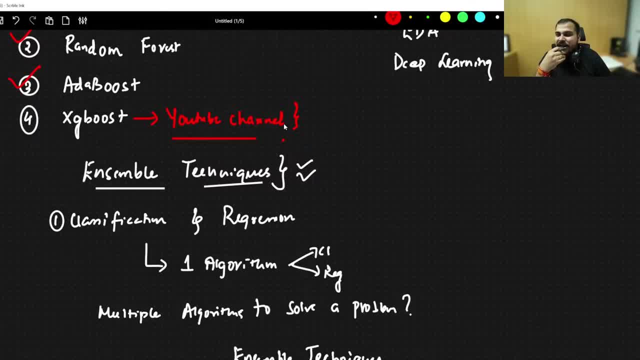 probably i will take up all the probably i will take up all the unsupervised machine learning techniques, unsupervised machine learning techniques, unsupervised machine learning techniques- and probably take one class completely on and probably take one class completely on and probably take one class completely on that. 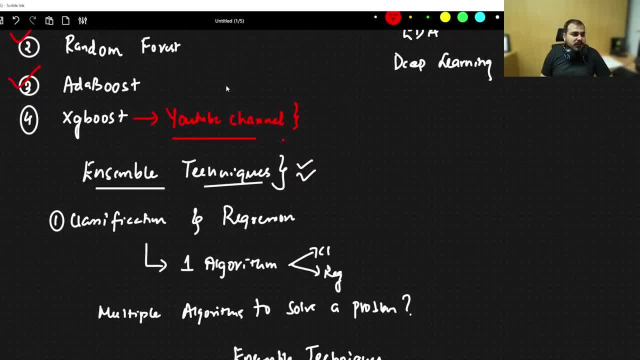 that, that, and uh, let's see okay. and uh, let's see okay, and uh, let's see okay. so, thank you everyone. uh, please make so. thank you everyone, uh, please make so. thank you everyone. uh, please make sure that subscribe the channel. hit like. sure that subscribe the channel. hit like.